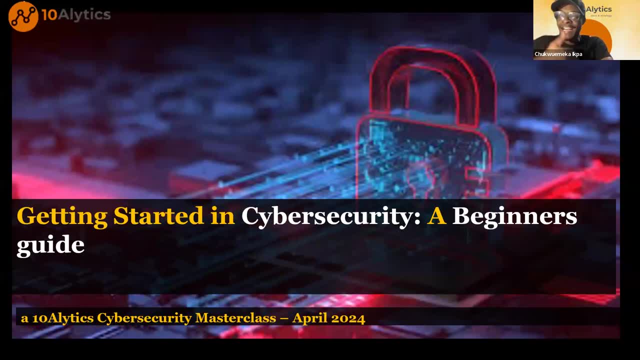 before now. you can type in a two so that I can also get to understand you. Amazing, amazing, fantastic. I'm going to say a couple of one, which means most people here today is the first time that we are joining a session. Okay, amazing. So we are going to dive right into it while we 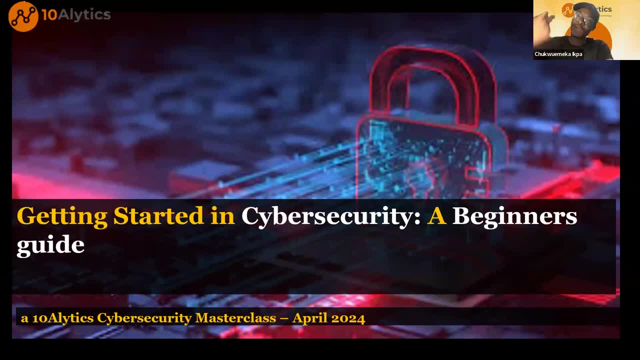 wait for others to join us. Remember, we are here today basically to talk about getting started in cybersecurity- a beginner's guide. You've been hearing about cybersecurity, cybersecurity, how can you get into cybersecurity- And that is what we are here for. 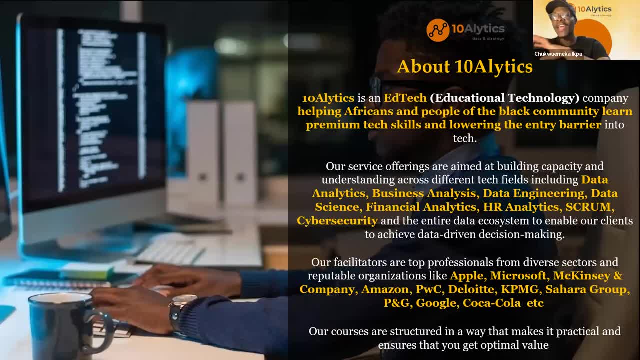 We are here today to diversify, right, And basically we are Tenality- right For people that today is the first time that they are joining us on this call. we are Tenality. We are an educational technology company that help Africans and help the Black ecosystem to get into the tech. 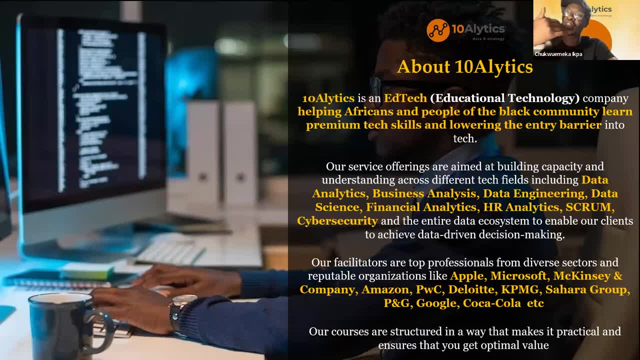 field. So what we do is we lower the barrier, the entry criteria into the tech field and make it possible for everyone that desires to be here to easily join the tech field, And our service services range over data analytics, financial analysis, data engineering, data science. 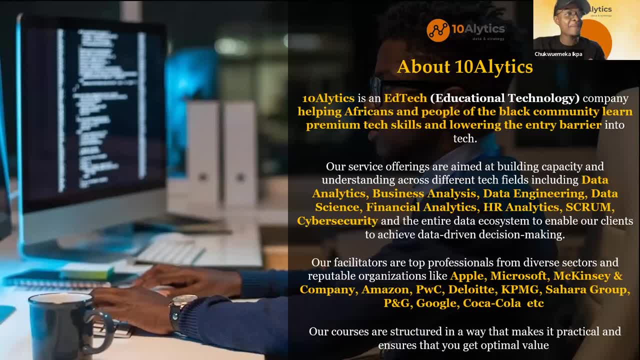 financial analytics, HR analytics, Scrum and, of course, cybersecurity, which is the main reason why we are here today, right, And we have amazing participants that join us from diverse sector, from Apple, from Microsoft, from McKinsey, from banks, from KPNG Assets, Bank, Deloitte. 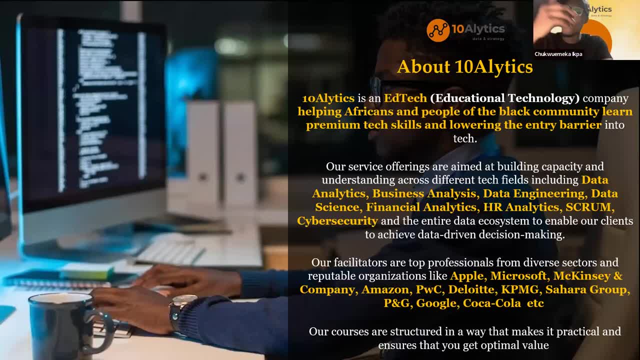 and so on and so forth, And we have our students also working in these amazing places, Right? So just rest assured that you are at the right place, because we are going to make sure that you understand all that you need to know regarding cybersecurity and all that you need. 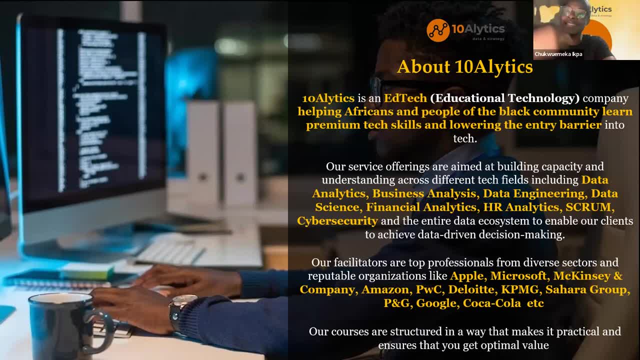 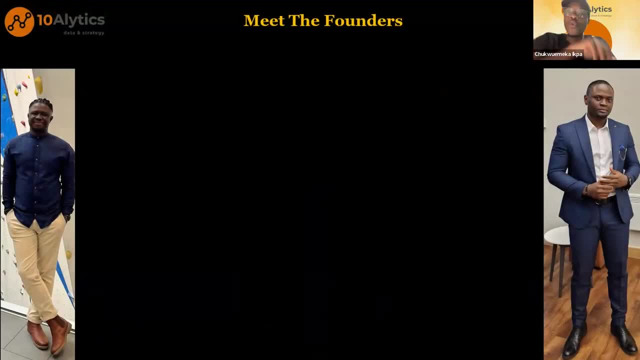 to know regarding how a beginner can get started in cybersecurity. So we have Adeza Suleiman and Efemena Ibro, who are the founders of Tenality right. So if you can see my screen, you can see Adeza. 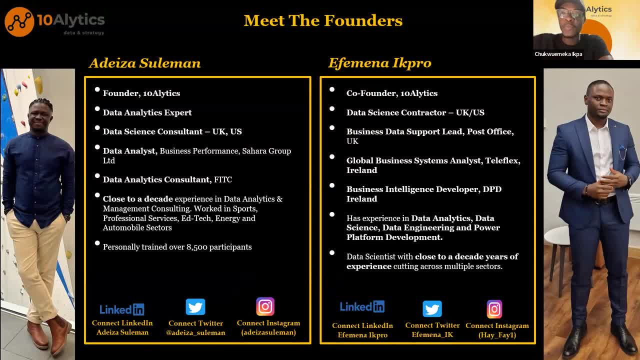 And Efemena. So Adeza is a data analytics expert that has worked across so many sectors- He's worked in consulting, He's worked in ed tech, in energy, in automobile- And he's worked across many regions- Africa, UK, Canada, right- So he is well-versed in this area And that is Adeza. 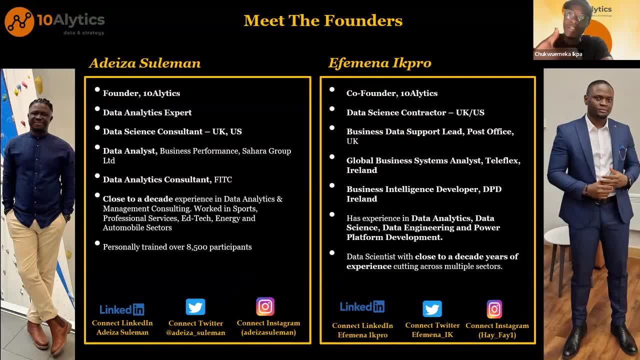 right Adeza founded Tenality when he was in the field and he was never able to see like-minded Black individuals that he can interact with, And that led to him founding Tenality. Also, we have Efemena Ibro, who is also the co-founder. 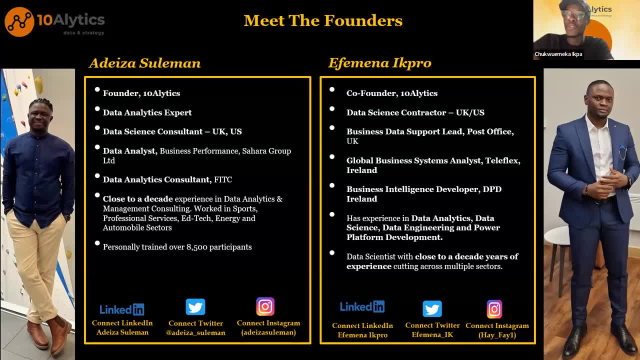 Efemena is a data scientist and he has worked across diverse sectors- right, He's worked as a power platform developer, He's worked as a data engineer, as a data scientist, And presently he is working in Canada. right, And both of them have over a decade experience in education. 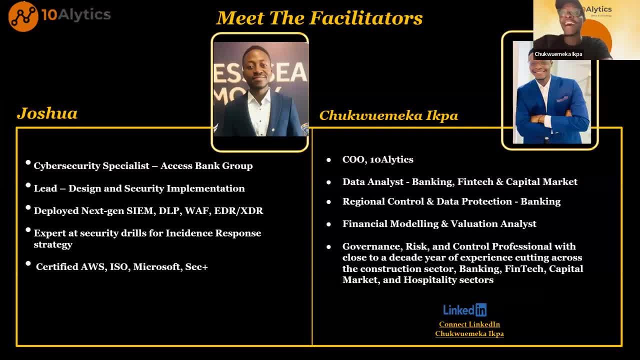 technology right- And this is a very important part of his career, And he's worked as a data scientist right, And both of them have over a decade experience in education technology right, And we have an amazing person with us, Joshua. Joshua, I don't know whether you're on the call. 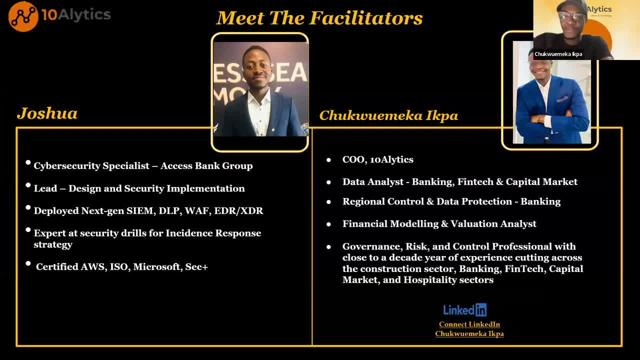 whether you want to say a couple of things to people before I introduce you. Hi Joshua, Hi Chukwemeka, Thank you very much. I'm Joshua, I'm a cybersecurity specialist and I work with Access Bank Group and also design security policies, And I've also 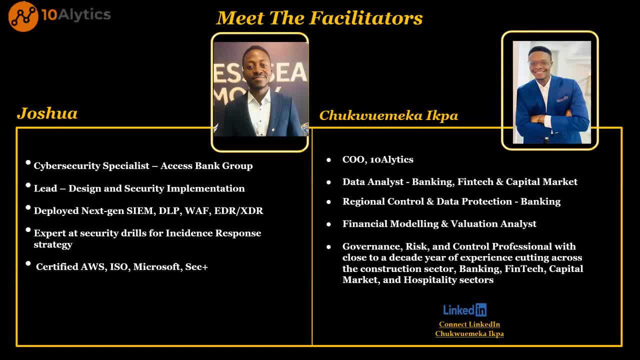 deployed security tools like the SIEM, DLP, and all of that, And working with Ten Analytics as well, has been very, very interesting. Thank you very much, Chukwemeka. Thank you so much, Joshua. Thank you so much, Joshua. Like Joshua has mentioned, 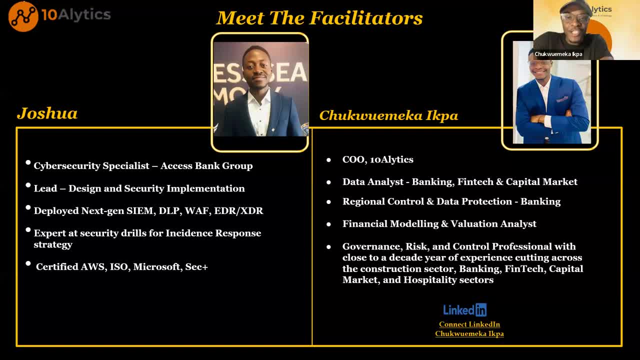 he is a cybersecurity specialist from Access Bank and he worked across so many projects And today he's here with us so that we get to understand how we can get into cybersecurity. a beginner's guide. I am Chukwemeka, the COO for Ten Analytics. Basically. I've worked across so many sectors. 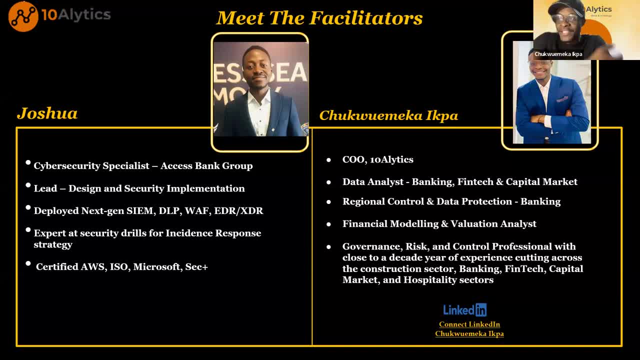 banking, fintech, Capital markets, hospitality business. I've worked in governance, risk and control, which is partly cybersecurity right, And basically I have close to a decade experience in all these areas as well, And today we are going to discuss things that are very 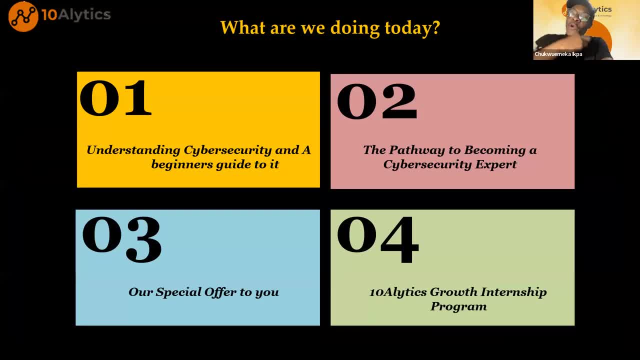 very, very important to us. right And number one thing that we are going to be doing today is to understand cybersecurity and a beginner's guide to it. right For us to understand cybersecurity and a beginner's guide to it. And also number two we are going to be understanding. 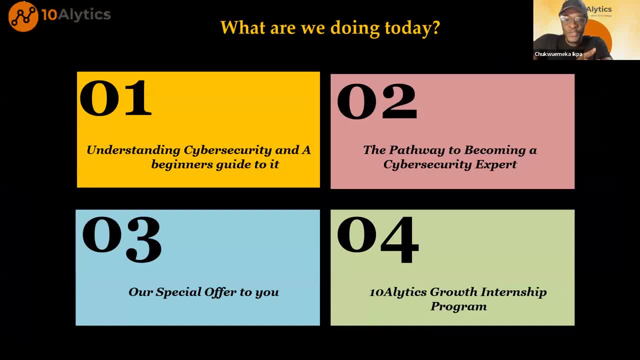 the pathway to becoming a cybersecurity expert. So you want to become a cybersecurity expert this 2024, how can you make it happen? right, We are here to let you in on the gist, so that we all can go together this 2024 and be able to make impact. Number three is that we are going to be bringing 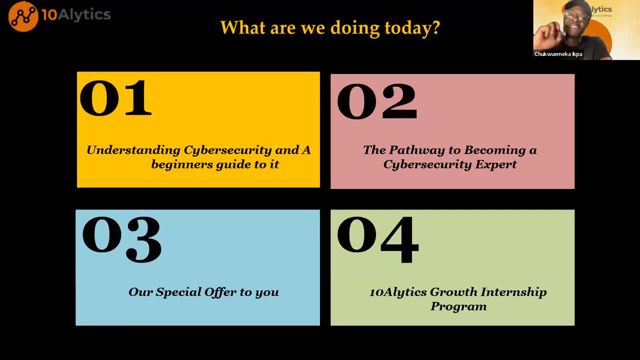 forth our special offer to you. So, by virtue of you being on this call, we have a special offer that was specially created for you And it's not for everyone, So just stay tuned and make sure that you partake in these amazing gifts that we have for you. this 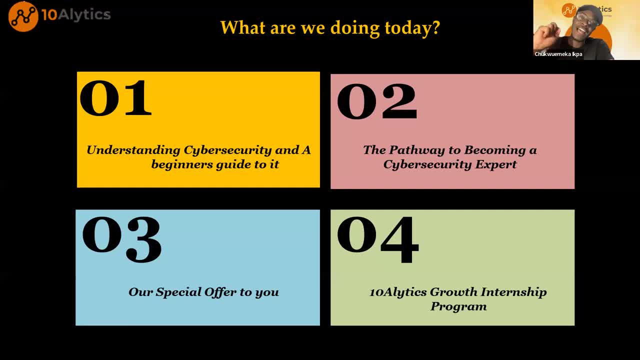 evening. And number four thing that we are going to be touching is the analytics growth internship program that will enable you to have experience. You're going to work on live projects that you are going to have on your portfolio so that when recruiters look at your portfolio, they will know. 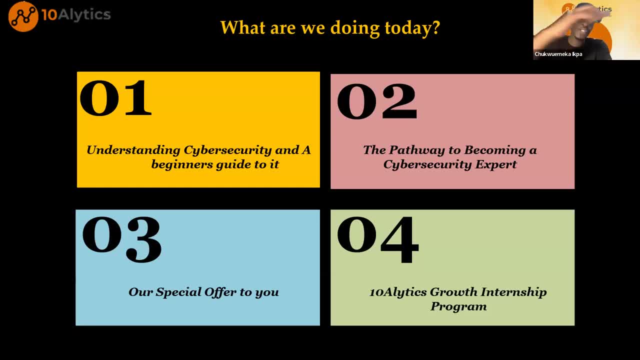 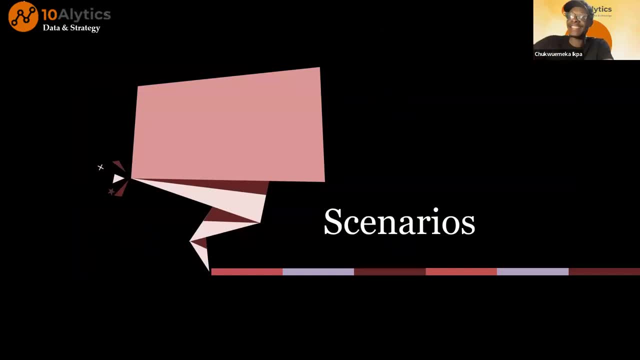 that you have the necessary skills and experience. So remember what we said: we are talking about understanding cybersecurity and a beginner's guide to it. How many of us here before now have heard about cybersecurity? So if you've heard about cybersecurity before now, just type a one so that I will know people that know what. 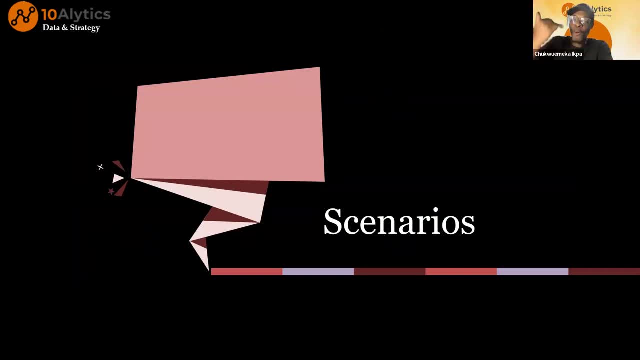 cybersecurity is all about, And I will know how I'll bring us up to speed to people that do not know yet. Amazing, Amazing. I can see a couple of one. I can see a yeah from King. I can see Daniel. I can see Elvis. I can see Brawler. Yeah, Amazing, Amazing. So we've all. 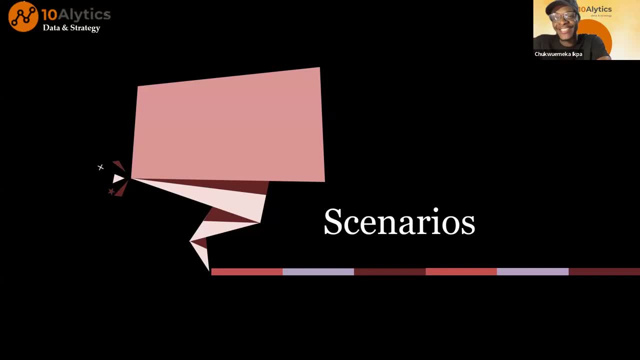 heard about cybersecurity. That means we should just close shop Now. we already understand what we need to know, right, But that's by the way. So I'm going to paint a couple of scenarios, right, that will enable us to understand cybersecurity fully. right, I'm going to. 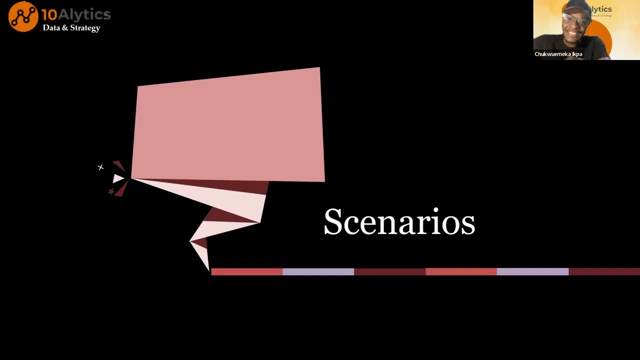 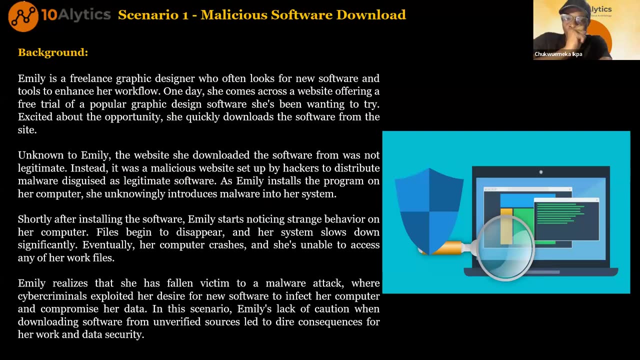 paint a couple of scenarios. that is going to enable us to understand cybersecurity fully. So I have on my screen a little story, right? So just walk with me so that you get to understand where we are. She often looks for new softwares and tools to enhance her workflow. One day she 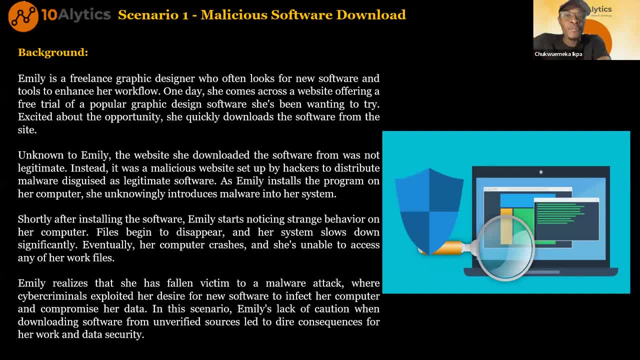 comes across a website offering a free trial of a popular graphic design software she's been wanting to try. Let's just put a scenario: You want to use Canva Right And you notice that Canva for the paid version is not really. you cannot afford it. 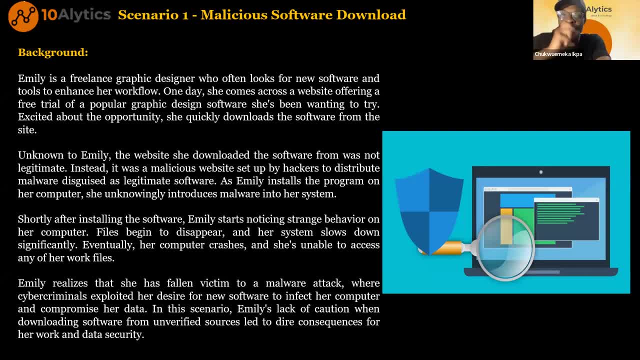 right And suddenly you get to see a. you know, in your email you come across an offering of a free trial for Canva, And Emily was excited about this opportunity. So she quickly downloads the software from the site Unknown to Emily. the website she downloaded the software from was: 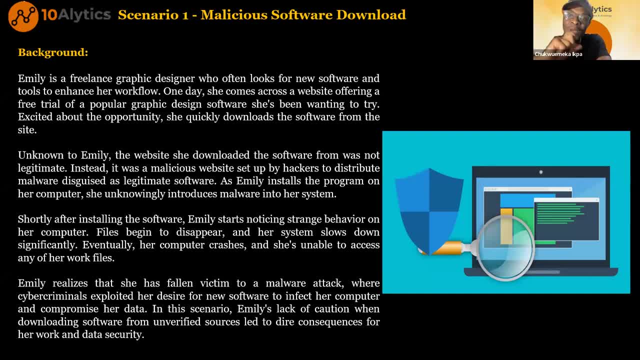 not legitimate right. Instead, it was a malicious website set up by hackers to distribute malware disguised as legitimate softwares. As Emily installs the program on her computer, she unknowingly introduces the malware into her system. Shortly after installing the software, Emily starts noticing strange behavior on her computer. Files begin to disappear and her system 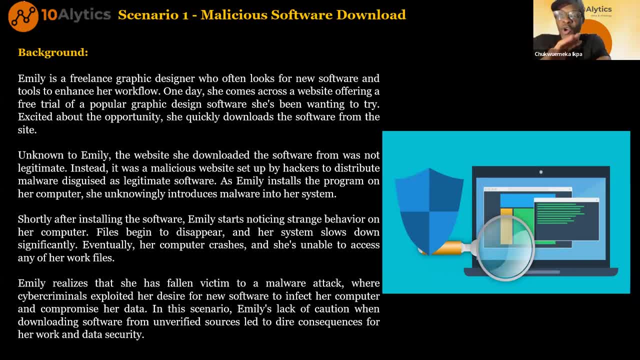 slows down significantly. Eventually, her computer crashes and she's unable to access any of her work files. So Emily realizes that she has fallen victim to a malware attack, where cybercriminals exploited her desire for new software to infect her computer and compromise her data In this. 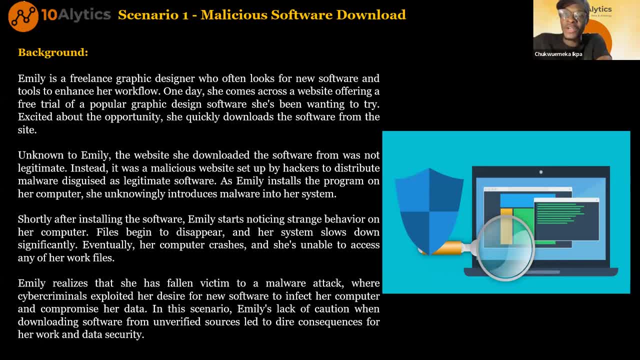 scenario. Emily's lack of caution when downloading software from unverified sources led to dire consequences for her work and data security. I don't know if we think Emily did the right thing or if we think is there things that Emily should have done. 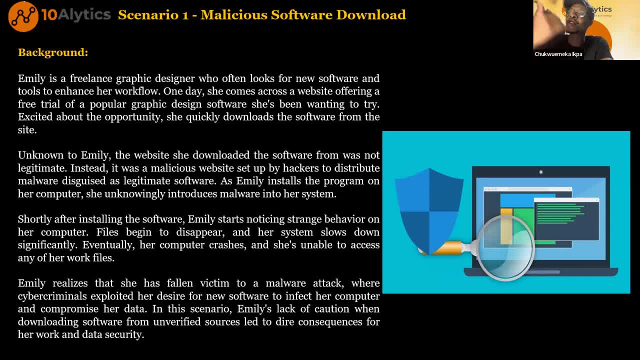 To prevent her from installing malicious software on her PC. On daily basis, we all make use of systems or phones or anything, And right now I'm sure we all have two-factor authentication on our WhatsApp, on our Instagram, on our apps. We all have two-factor authentication, right And that. 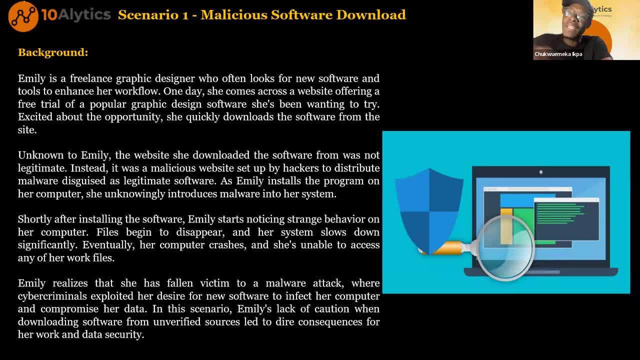 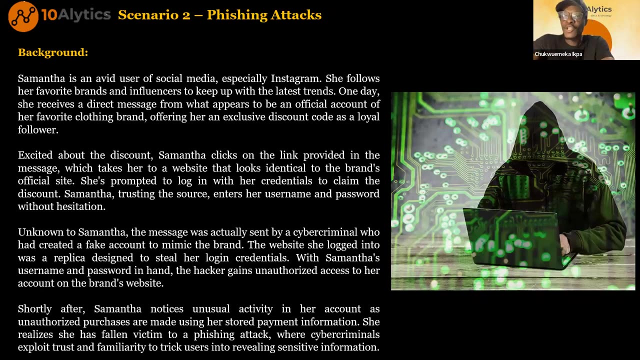 is us practicing cybersecurity on a minimal level, without knowing it right. So we all are cybersecurity experts, even though it's still at a minimal level, But we are practicing what cybersecurity experts do, Right? So it's basically about Samantha, right? So Samantha is a social media. 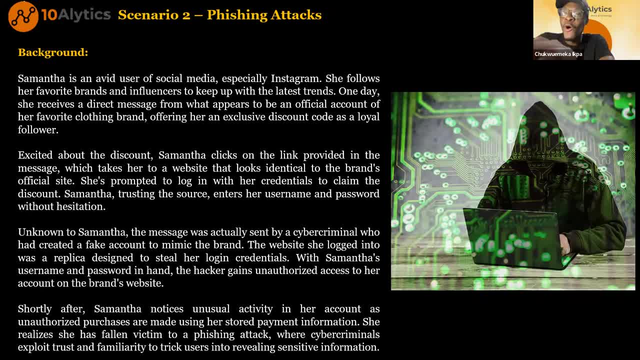 person and she uses Instagram On a daily basis. we all use Instagram And we've heard stories of people losing their accounts on Instagram. right, How do these things happen? What's going on? How do these people lose their accounts? So let's paint the story with Samantha She. 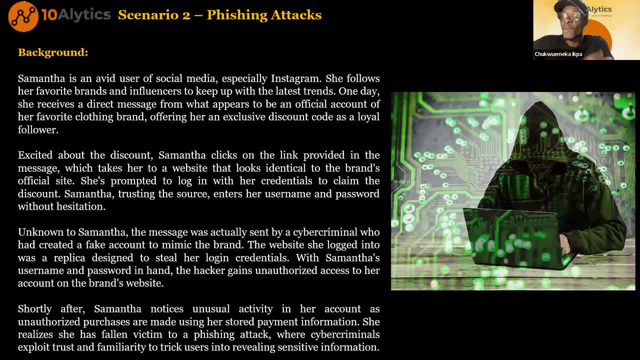 follows her favorite brand and influencers to keep up to date. Then one day she receives a direct message from what appears to be an official account of her favorite clothing brand, right? So let's assume, suddenly one day you are receiving a discount from Miss K. So if you're in Lagos, 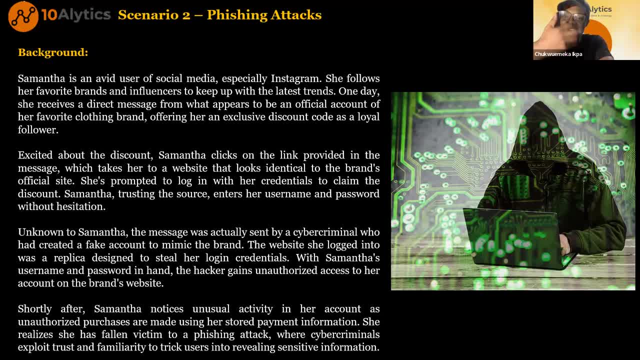 I'm sure you know Miss K- for the ladies here- right? So you are receiving a discount code from Miss K, right? And we're excited about that discount code. And we're excited about that discount code, So you clicked on the link provided in the message which takes you to their website. that. 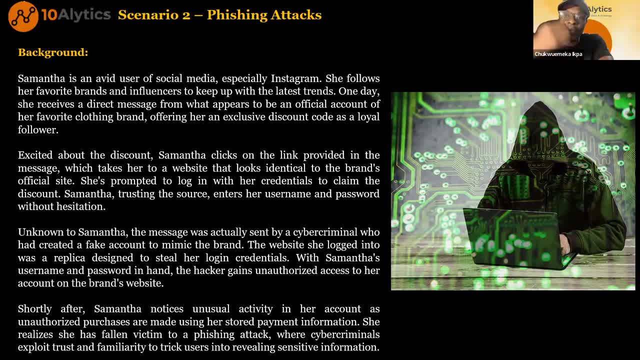 looks identical to the brand that you're officially patronized, right, And you've logged in your details, you've put in your card details, you've put in everything so that you can claim the discount, thinking that it is the authentic shopping platform that you are on. Then unknown. 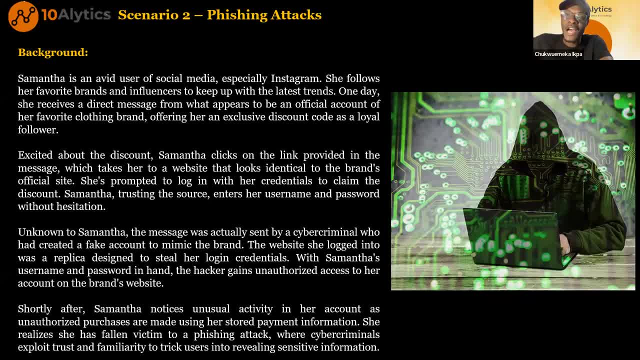 to you. the message was sent by cyber criminals who created a fake account On daily basics. we all see several accounts created on IG, on all social media platforms, on Twitter, trying to mimic the original accounts. right, And we can fall prey to what cyber criminals? 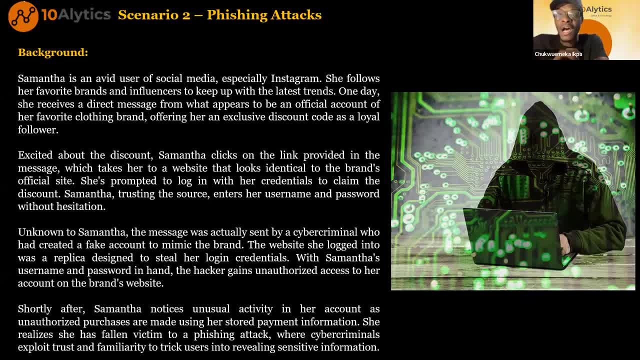 do if you are not careful. So shortly after Samantha repeated everything, she noticed that unauthorized purchases were made with her card and everything that she stole. she realized that she's falling victim of a phishing attack. In the end, she was able to claim the discount code. 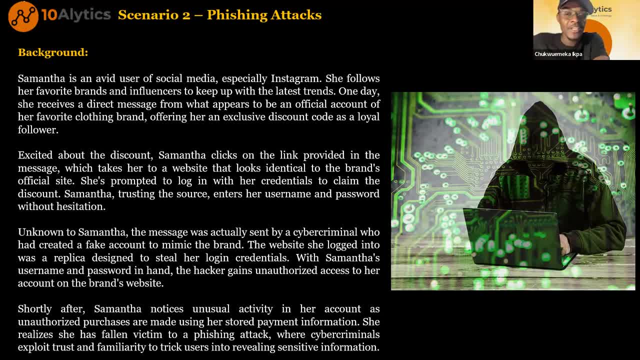 In this regard, cyber criminals exploited Samantha's trust and familiarity to her original brand to exploit her information right, And this is how phishing attacks normally come up and how they normally look like. Now Samantha has fallen victim of phishing attack. If you are just joining, 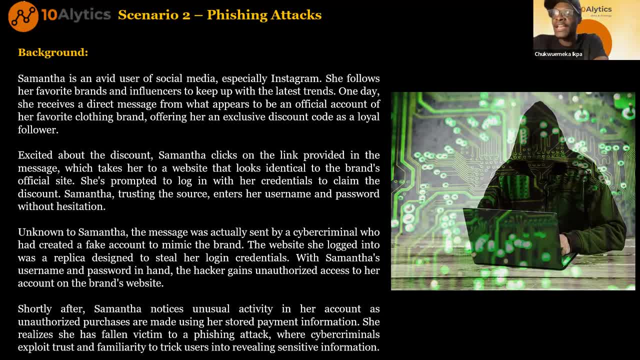 this session, please. my colleague Elijah and Lydia. they are dropping the attendants, So please feel free to fill in the attendance so that you can get the recording of this video and also get the file, the PDF, that we are using to teach. So we've talked about Samantha and Emily. that. 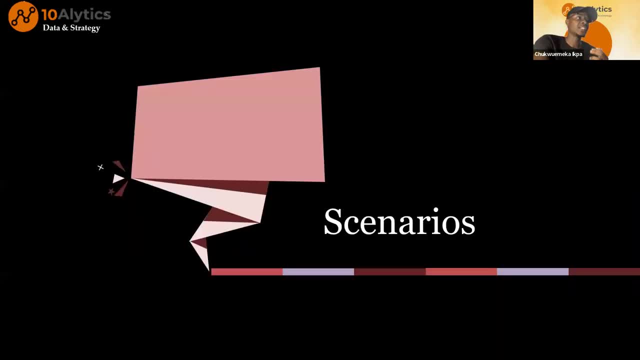 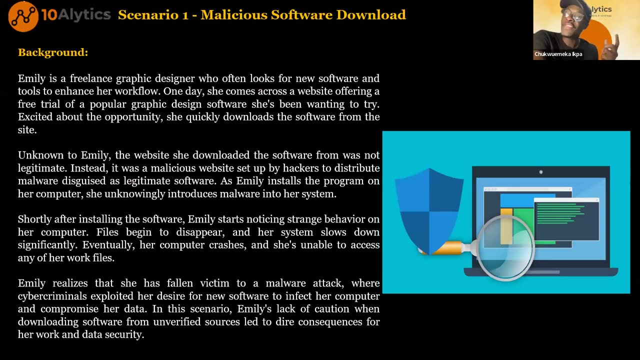 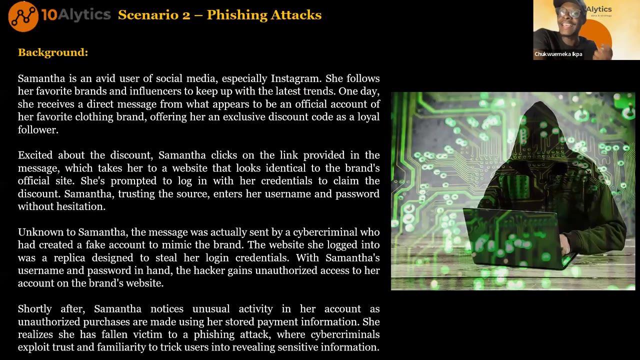 fall prey to phishing attacks and malicious software downloads. Now, these are specific issues, specific things that are peculiar to cybersecurity experts, And these are things that our members of the security staff have to deal with. So this is the first thing that we talked. 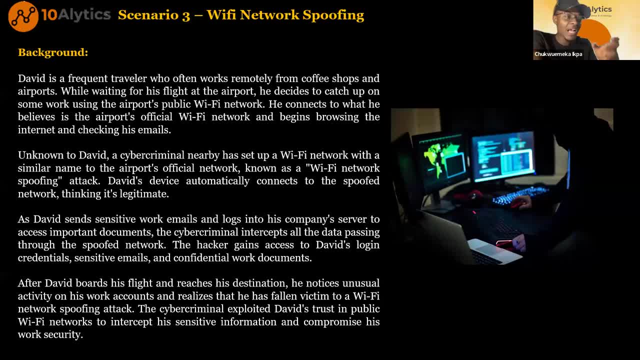 about The first question in the question: how can we get to block all these things from happening right? How can we make all these things? How can we bring data security to the organizations Now? lastly, let's look at this exact scenario Now. most of us when we fly, or maybe when you. 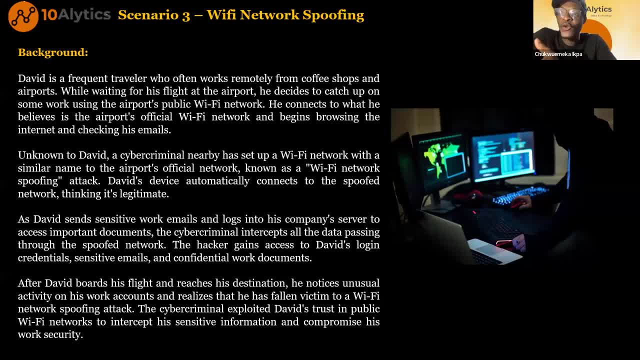 find yourself in restaurants or hotels, you tend to log into the public Wi-Fi right, And we have David here who travels frequently, So in the airport he just saw the free airport Wi-Fi and just opened the door to open an airport. Now I know that there are people who are the most suffering. 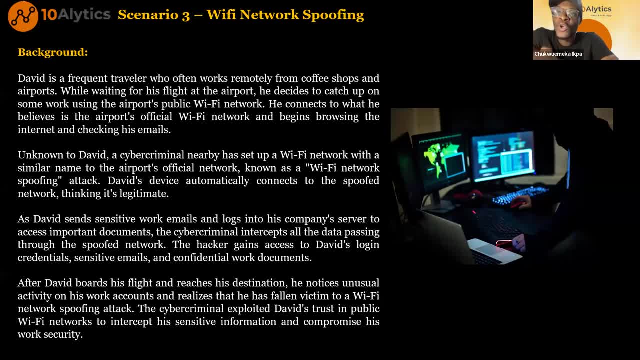 victims here. We need to be doing that. So this is what we're gonna talk about And this is the last and just logged into it. right, unknown to david, a cyber security, a cyber criminal, nearby has set up the same exact wi-fi name with the similar name for the airport, and that's the one that david 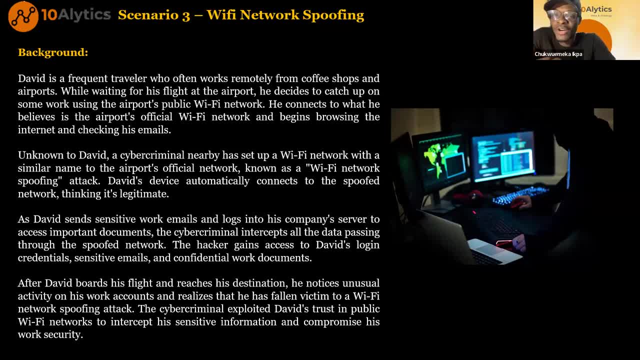 logged into. now david started browsing um trying to- you know, do so many things, so i see he's sending sensitive work emails and logs to his company server. the cyber criminal that opened that free wi-fi was not able to intercept all the data passing through the network, now unknown to david. 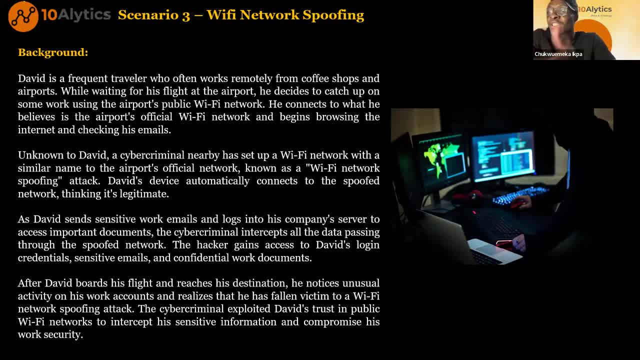 david has entered the plane he's flying and by the time he's dropping off, by the time he's touching down on the airport, he noticed that a cyber criminal has exploited his trust, and i've logged into his work emails and captured the company's data. now all these are areas how we can fall prey. 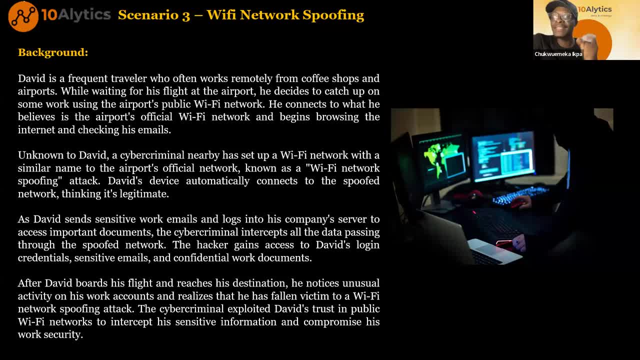 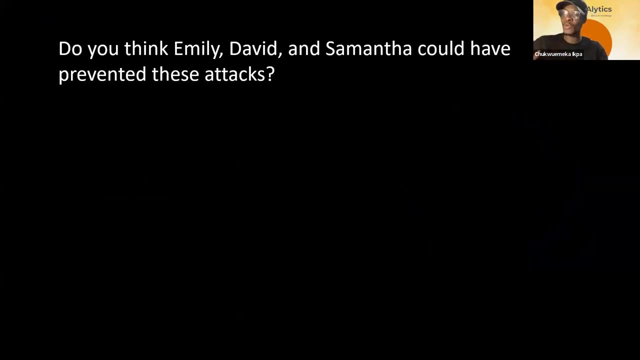 to cyber criminals. right, these are things that, and on daily basis. there is always new ways that these guys are coming up to try- and you know, capture all our data. in any field that you are in, there's always need for a cyber security analyst, which is why we keep telling people that cyber security is a field that will 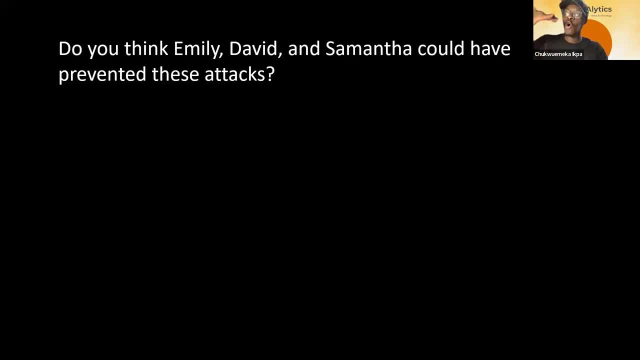 always continuously be in demand. right, it will always be in demand. now. do you think david and samantha could have prevented these attacks? right, let me hear what you think. just type in the chat box. do you think emily, david and samantha that fell to all these cyber attacks? 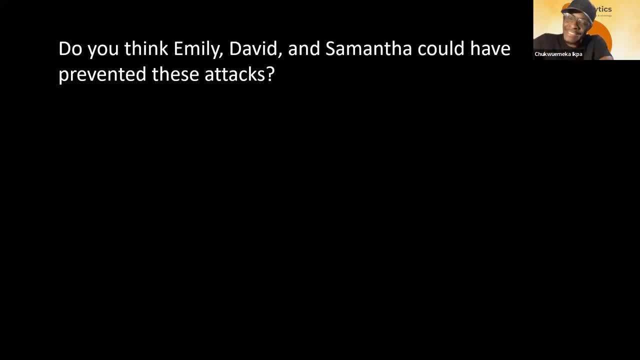 do you think that they could have prevented this? so just type what you think in the chat box. if you think yes, they can prevent it. if you think no, that they can't prevent it, just tell me so that i can see whether we are thinking in the same direction. okay, abraham. 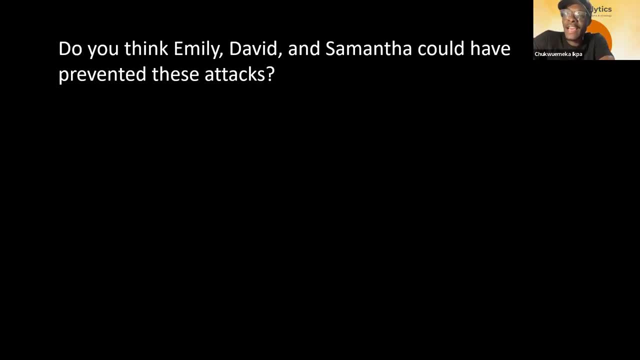 sharla said yes, that he thinks emily, david and samantha could have prevented these attacks, and the bio daramula said no, that he doesn't think this could have been prevented. amazing, i mean. i like. i like the fact that we are having different, different opinions. daniel apanam said: 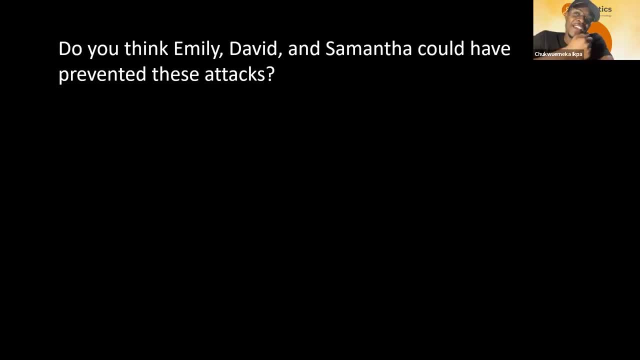 yes, they can. so i want to hear our thoughts. let me hear what's most of course on this call thing. let me hear your thoughts on this call thing. let me hear your thoughts on this call thing, what they think whether emily, samantha and david could have prevented this attack. okay, um, zoom. 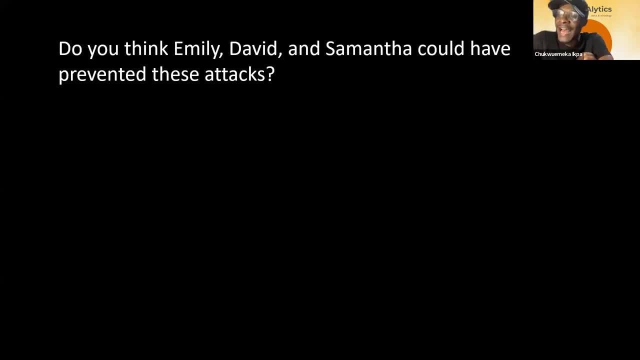 user said yes. he said yes, the attacks could have been prevented if they had basic knowledge of how to secure their online activities. amazing, yeah, carlo. amazing, all right. so david, samantha and emily: yes, the attack can be prevented. it is fun devil from charlie vibes, so we are going to continue. so, amazingly, yes, the attack could have. 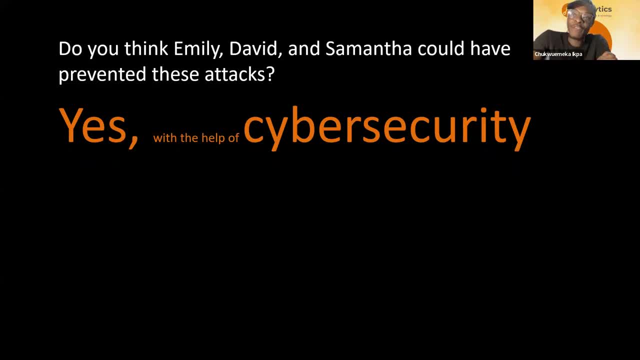 been prevented, right. right, this can, could have been prevented, and that is with the help of cyber security. so anything pertaining to cyber attacks- what cyber criminals are hitting on you, fishing attacks, um, malicious software downloads- this could have been prevented. right, and joshua is going to come up to talk us through how this could have been prevented. hi, joshua, you have. 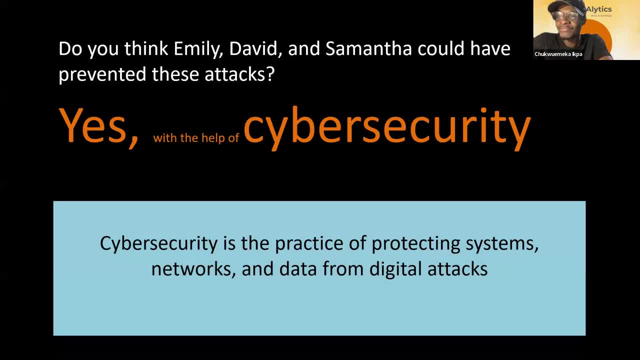 the time now. joshua, are you there? yeah, thank you very much. uh, chukwumika, you've done a wonderful introduction and that was a fantastic uh one day and uh. good evening everyone. i believe we are catching up with the flow. yeah, so i'm just going to be explaining um the cyber security. 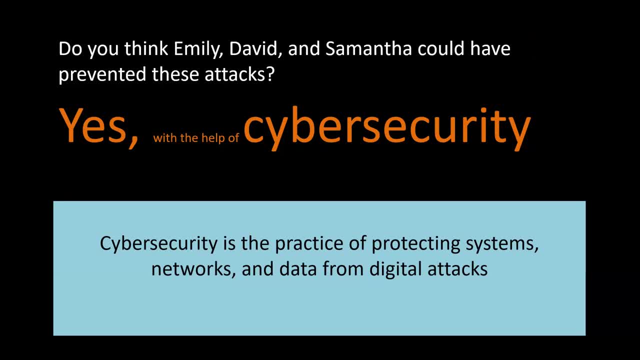 concepts and you know the scenarios. uh, we've all listened to the three different scenarios: emily, david and samantha. so they could have, they could be anyone, they could be a colleague, they could be, uh, brothers, they could be our family, they could be our friends, you understand? so i, i've met people. 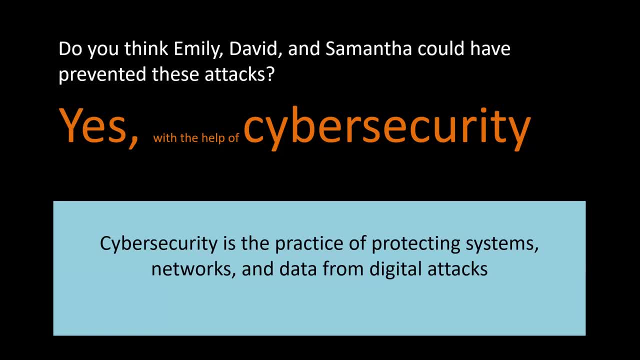 who say, ah, it will be very difficult for me to get, uh, hacked because i don't have any online identity, i don't have any social media profile, so nobody know anything about me. and what i tell them is that those you think you don't have an online identity, but you have an offline. 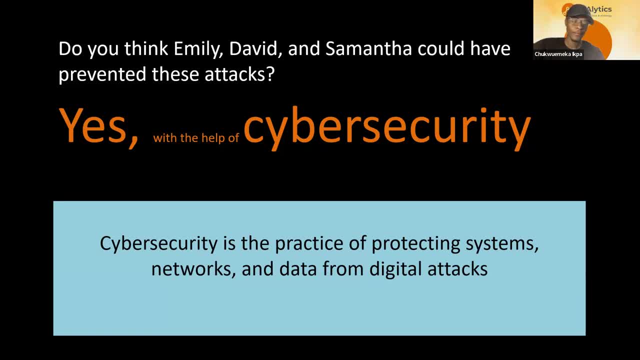 identity as far as you are communicating, as far as you are sending information in one way or the other, you know. as far as you are making use of phones, as far as you are making use of sms. and recently, uh phishing attacks and social engineering attacks. according to uh. 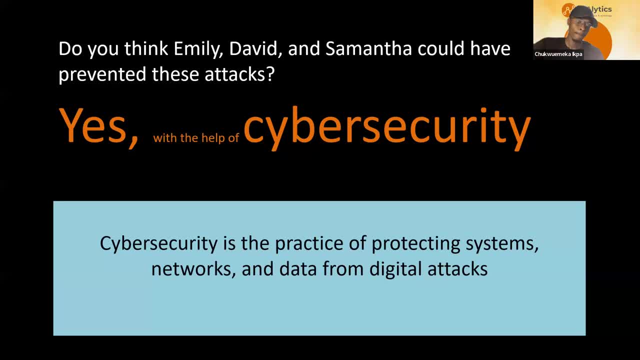 statistics and fbi investigation, he have recorded the highest number of successful cyber attacks so far amongst all other forms of cyber attacks. so so don't let us just uh look at it and say, okay, because it's a phishing meal or it's social engineering. the ultra have detected it, no, so 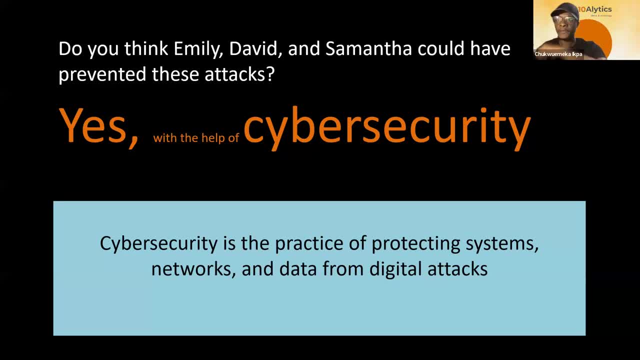 this is why cyber security is very, very, very important. so what is cyber security generally so, from from my own perspective, i would say cyber security is a way to protect individuals, to protect organizations and to protect the government at large. but when you are protecting this category of people, they make use of some things you know. so that is why the slide is talking about is the 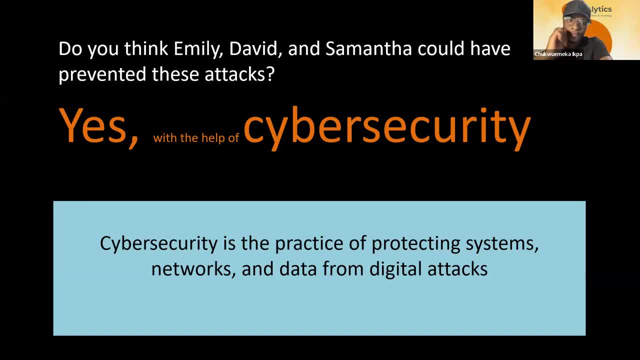 practice of protecting systems that the individuals make use of, protecting networks that individuals make use of and data from digital attacks. so these people- the individuals, the organizations and the nations at large- there are different categories of people that eventually need cyber security and you know, as technology is rising every day, we need um what they call the advancement in cyber security. so 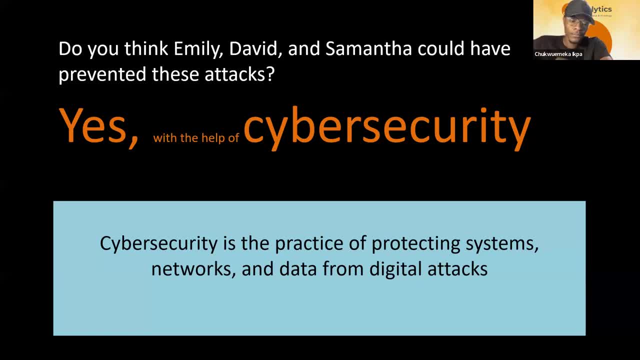 as technology is evolving, as we are having new updates from technology side, new innovations they also, as every innovation is unveiled, there are some flaws, there are some vulnerabilities around it. so that is a cyber security started. you know it is not exactly unethical to do so, but it won't lead to much more. but it will. 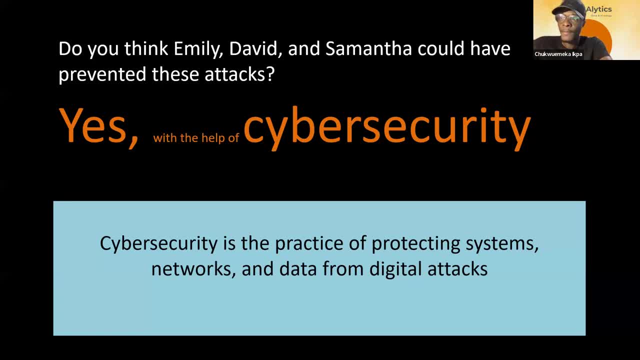 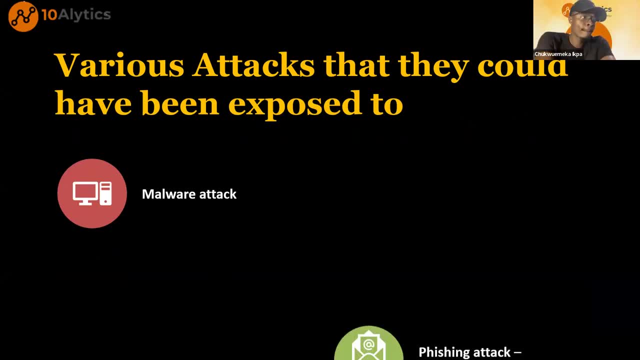 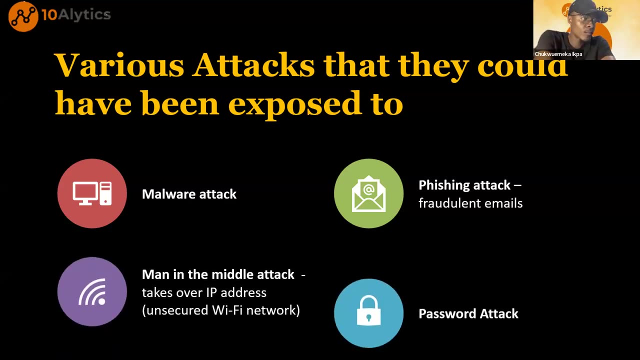 continue to be a very relevant uh discussion. you understand so. so just allow me to share my screen on second. all right, so now the various attacks that they could have been exposed to. you know we are talking about emily, i'm talking about samantha and the other guy from the three different scenarios. 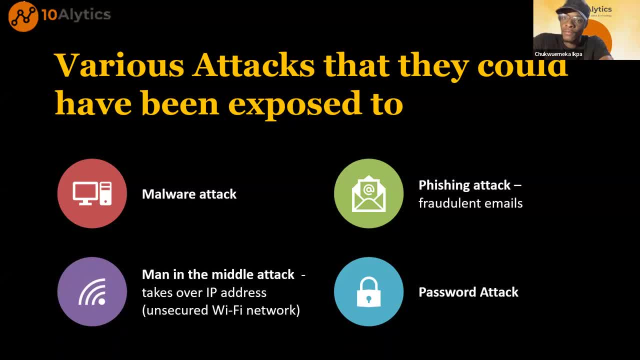 you understand. so the first one is my way attack pop into your mobile device can pop into any of your endpoints or assets or any uh workstation that you make use of, maybe personally or at uh at your organization or at your private firm, you understand. so a malware attack can be introduced through phishing meals, through 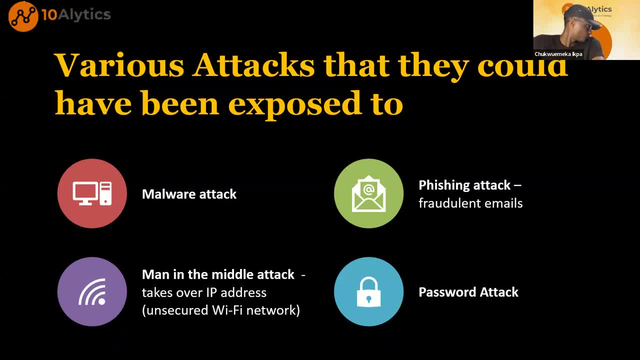 meals that you, you don't really know the sender as a cyber security specialist. there are some red flags you will see from an email that will give you, uh, an ink that, oh, this, this email is looking suspicious. you understand. so are the uh emily guy, the samantha guy. are they exposed to? 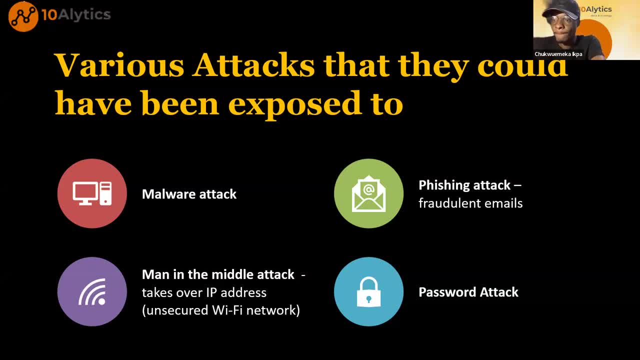 phishing attacks, of course, yes, you understand. so how do you even see a fraudulent email and pick it immediately? you know, immediately. you see some emails. just check the domains. okay, the domains are like a sender or the where the account is hosted on. you understand, just over your mouse around it. you don't? 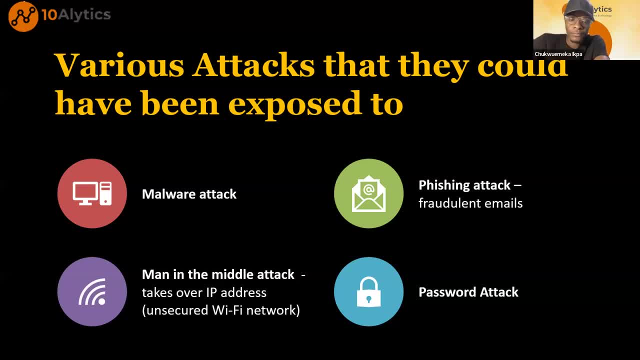 necessarily have to click it. so when you over your mouse around it, you see the the details of it and compared with the one that is showing on on the email that you just received, you see there's always a difference between them. so the domain, the actual domain, might, might be telling you it is. 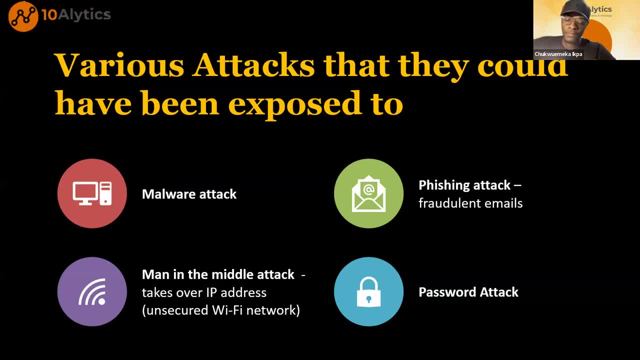 abccom. but by the time you over your mouse around the abccom that you're seeing, you'll be seeing x y z, x y z, one, two, three at, at, and different, uh, different um characters entirely, so that one alone is a red flag for you. you understand. so they could also be uh exposed to mitm. i call this mitm, it's uh. 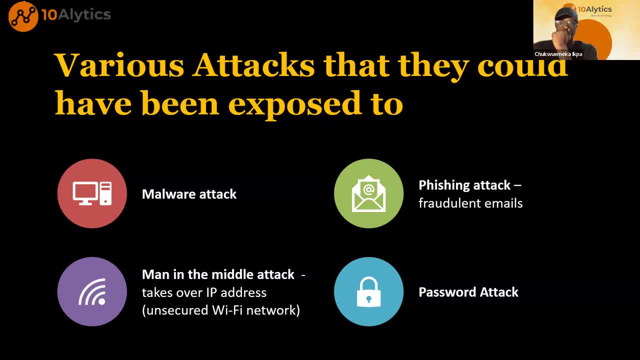 popularly known as man in the middle attack, because you know people not. naturally we enjoy free things and where we see free wi-fi password- uh, free wi-fi or public wi-fi- hotels, airport loans or all of that- we always like to make use of them, you understand, but the vulnerability there is that. 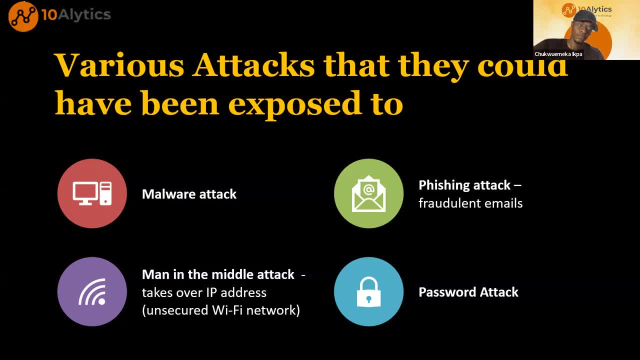 some of these public wi-fi addresses may have been cloned, and cloned in such a way that, okay, he said let's say the actual name of the public wi-fi you are using is abc, underscore, underscore 123.com, and you are seeing abc-123.com. so it might just take a little change and for you not to even 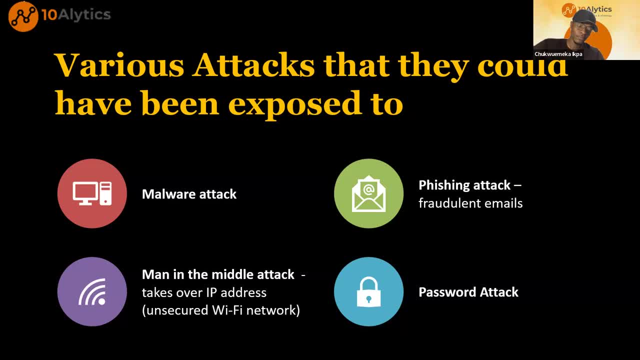 sometimes they even copy the exact name of the public wi-fi and you mistakenly or erroneously click on the fake one and you try to log in and you are using your, your, your personal system or you are using a system that belongs to a certain organization. you understand, and all of that so that alone, as you're entering your credentials to 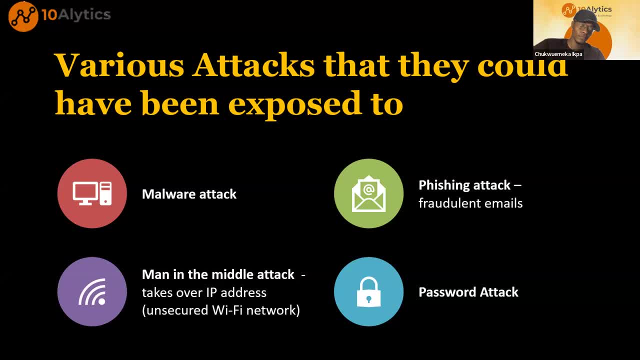 your social media profile. you want to check what's going on, you want to get updates and all of that that. someone is already picking all of those ashes as you are entering the password, as you are typing 1,, 2,, 3,, 4, 5.. 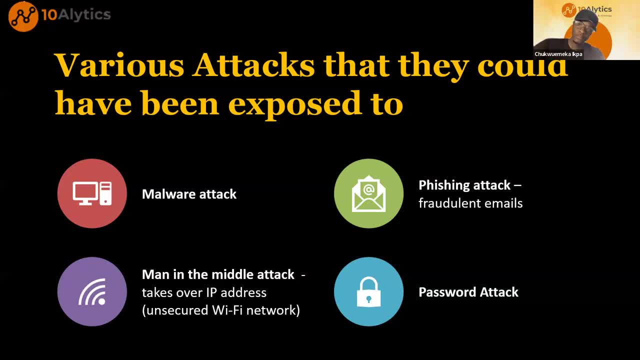 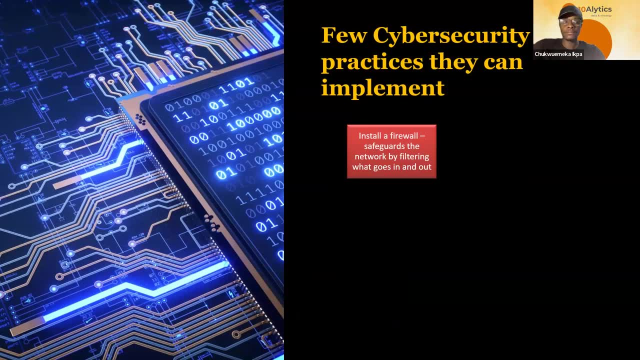 Someone is already seeing 1,, 2,, 3,, 4, 5 that you are typing. you understand. So that is a very serious form of attack. Now what are the few cybersecurity practices they can implement? So are they being? these guys are cybersecurity analysts. 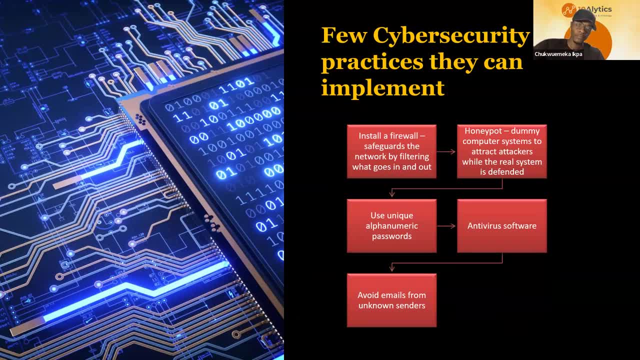 or they are not even analysts, but they are cybersecurity enthusiasts or they know little about cybersecurity. The first thing they would have done is to ensure they have a firewall. You know you can install a firewall that safeguards your network by filtering what goes in and what goes out. 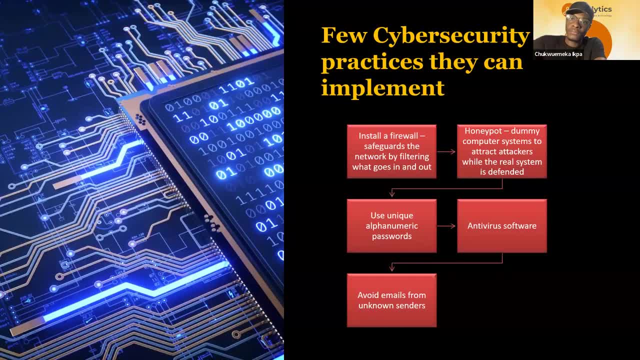 You understand? So these are the kind of things they can do. You can also install only port dummy on computer systems to attract attackers while the real system is defended, You understand? So we call it only port, only port technology. You understand? 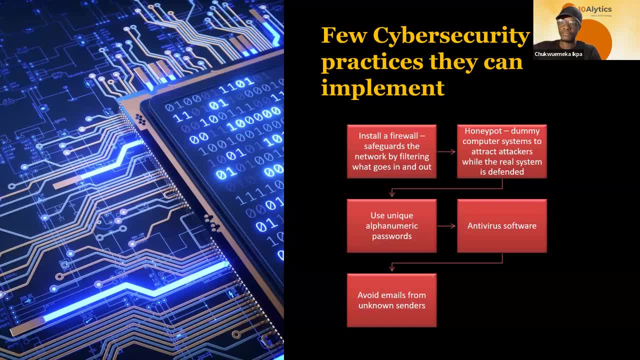 So these are the kind of implementations or drills that a cybersecurity specialist can implement for, maybe, the organization or for your own private firm, You understand. So when you are also using passwords, just make use of alphanumeric password, and not only alphanumeric password. you can make use of passphrase or paraphrase. 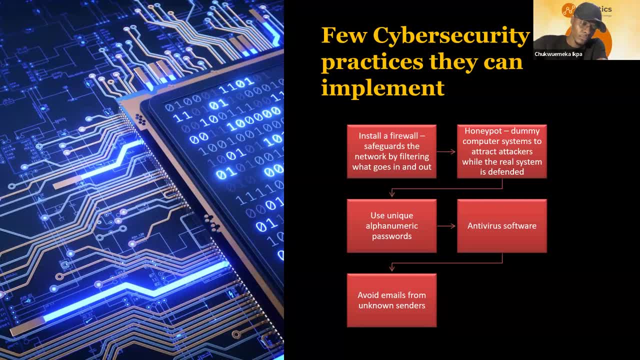 You understand. Make use of a phrase and change the letters to number. change the number and ensure that it meets the password. complexity, the criteria: It should be minimum of eight characters and 15, eight to 15 and above. You understand. 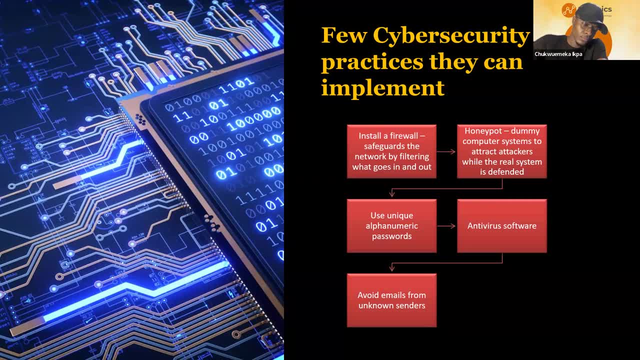 So make use of antivirus software, make use of emails from unknown senders and all of that. So all of these things does not guarantee 100%. Even the advanced OEMs- OEMs, I mean original equipment, manufacturers of IT solutions- they still get attacked. 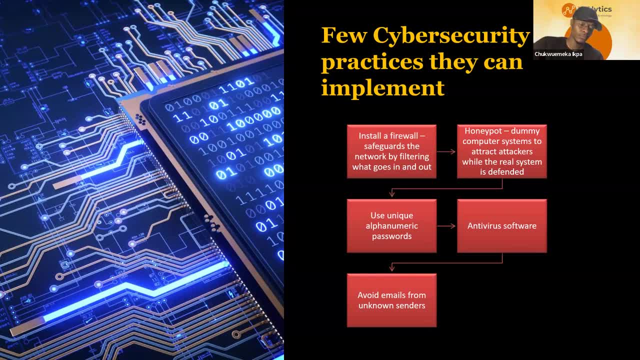 Microsoft still gets cyber attacks. Amazon still gets different kinds of cyber attacks. So where all these tools will help you is in detecting them and making proactive decisions, Because, based on past scenarios, you can predict the kind of attacks your hackers would like to. 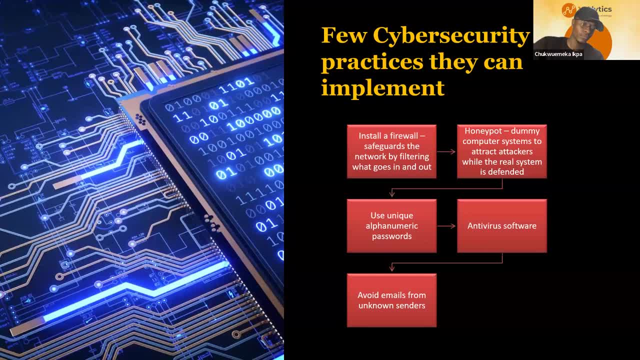 you know, would like to tap into, So it does not only give you the 100%. That's why cybersecurity specialists, cybersecurity analysts, cybersecurity engineers are always needed to fine tune these tools, to make use of these tools to analyze what 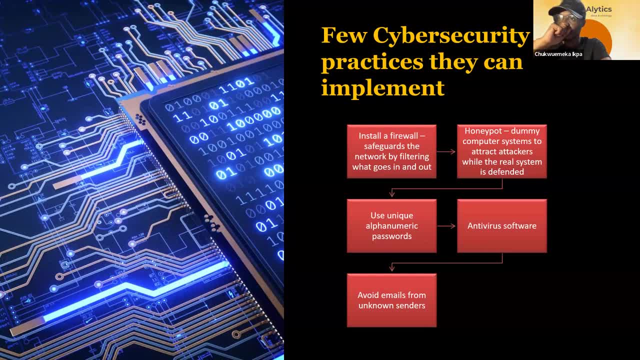 okay, what this tool has been able to detect, You understand. So we have the IDS, we have the IPS, we have intrusion detection system, intrusion prevention system, We have EDR tools, endpoint detection and response solutions that can help you. look at all these. 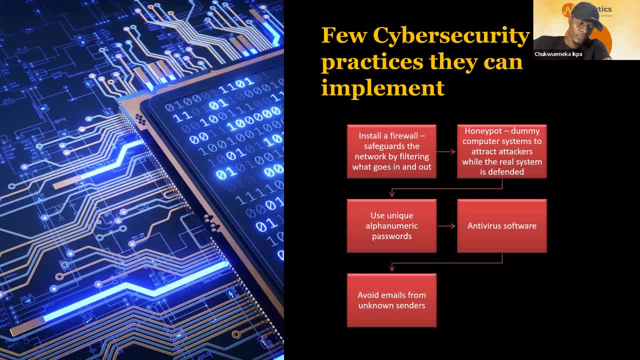 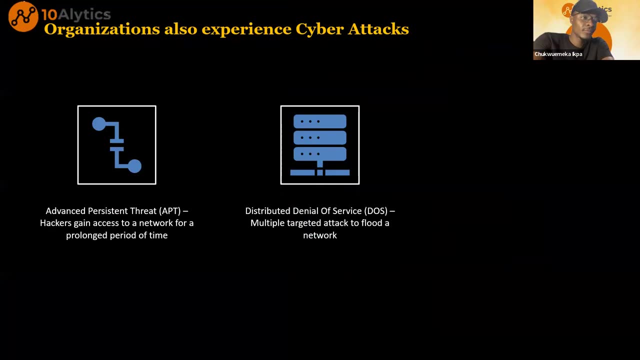 things and detect it. at a glance, You understand. So that these are just a few practices they can implement according to the scenario. Yeah, So I think we can. we can move. Yes, So, so organizations also experienced cyberattacks, as I mentioned this earlier. 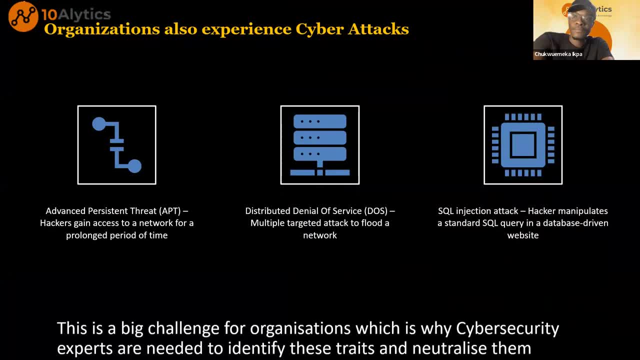 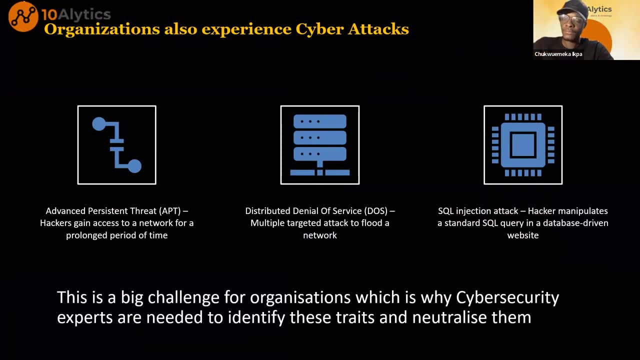 you know the kind of cyber attacks they receive daily, on a daily basis, depending on the industry they find themselves. we get APT. APT is advanced, persistent threats. You understand Hackers are trying to gain access to a network for a prolonged period of. 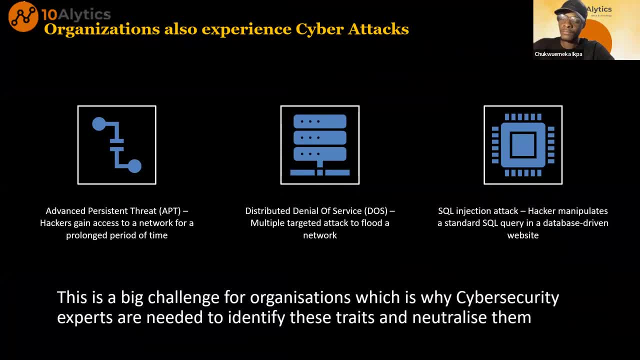 time, You understand. So they try and try and try. So that's how you get some kind of scans. You just discovered some unknown IP address, some some kind of strange IP addresses. as a cyber security analyst, When you see there are some red flags, 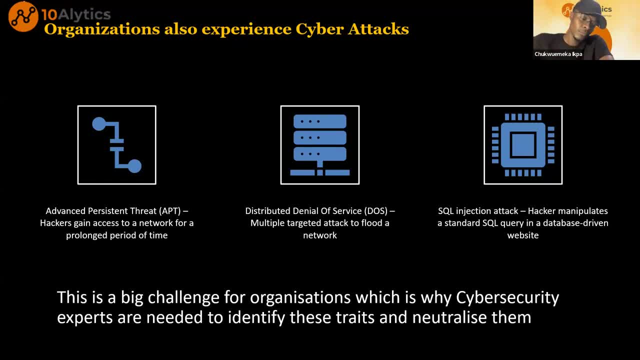 you see, when you see those kinds of events, there are some certain steps. Hi Joshua, Hi Adam, Can, can anyone hear me? or Joshua, Yeah, I think we lost Joshua there for a while. Okay, So basically what Joshua is trying to say, that is that we have 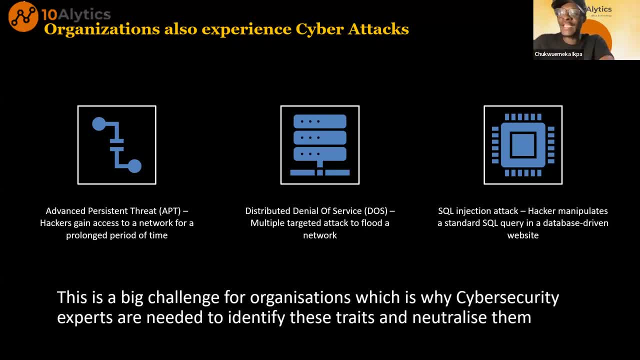 issues like these also coming up in organizations, right? So the same way individuals experience cyber attack, that's the same way of musician also experienced cyber attacks, And the truth is that they even experienced it on a larger scale, right, Because on a daily basis, 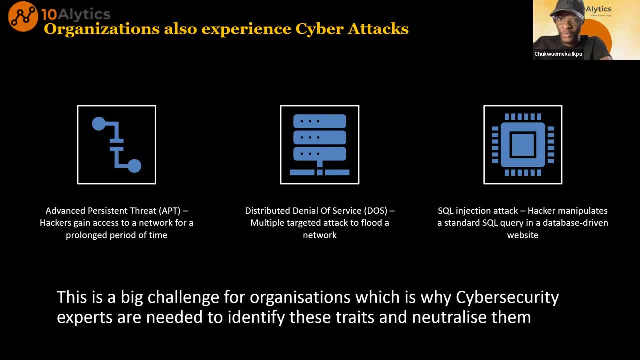 they are experiencing cyber attacks, and the truth is that they even experienced it on a larger scale. but on a day to day basis, hackers are trying to get into our financial institutions so that they can have access to your money. They're even trying to get access into, maybe hospitals so that they 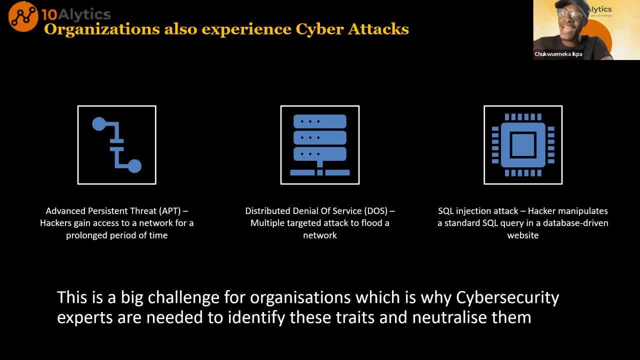 can blackmail you with your hospital record. So they are trying on a daily basis to get into all these organizations, And that is why it is very, very important for organizations to be able to protect themselves with respect to cyber attacks. Joshua, I don't know whether you are back. 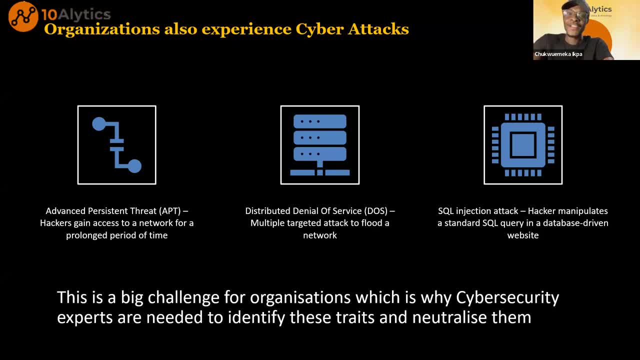 Joshua, are you there now? Absolutely, Thank you very much. All right, So so so, apart from DDoS, we also get SQL injection attacks. Okay, These are specifically attacks that are targeted towards your database, You understand. 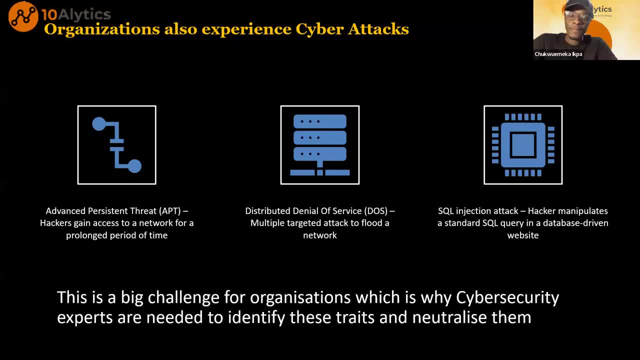 you know, the database is like the art of your application. So whatever resides in your database affects your application. So these are the kind of cybersecurity attacks they get. they get on a daily basis of big organizations and all of that. So it's a big challenge for organizations. 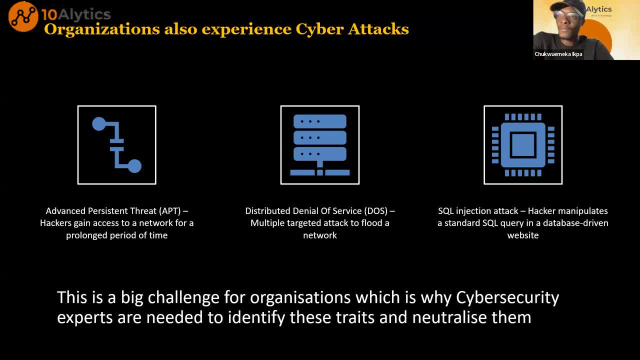 This is why cybersecurity specialists, the job rules, the job vacancies are on the rise, Yeah, On the rise. Recently, I just read that Zambia was the last week or so that they've been attacked, that they uncovered some syndicates, and these guys are from the. 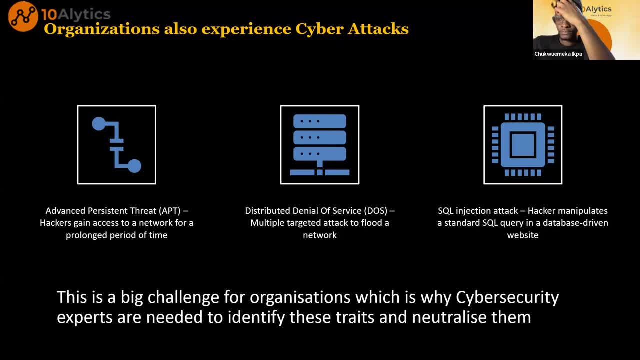 Chinese. They were already in their country. They employed young people from the age of 20 to 25, and guess what they've been doing? They've been calling on suspecting citizens of Zambia. You have been calling them, telling them. 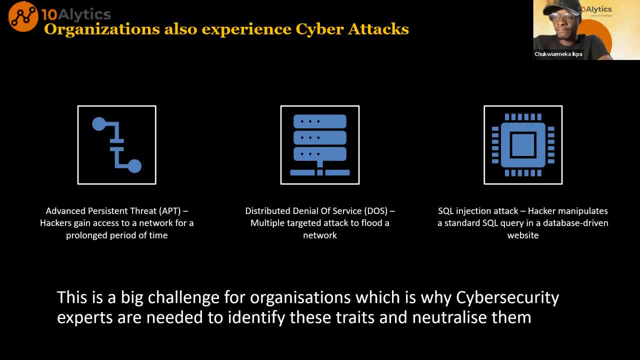 okay, we are bank employers. We want to help you. Your ATM is having issues. Just send us your password, We'll click on this link and all of that. And they've been getting serious debit a lot from different, from different angles. 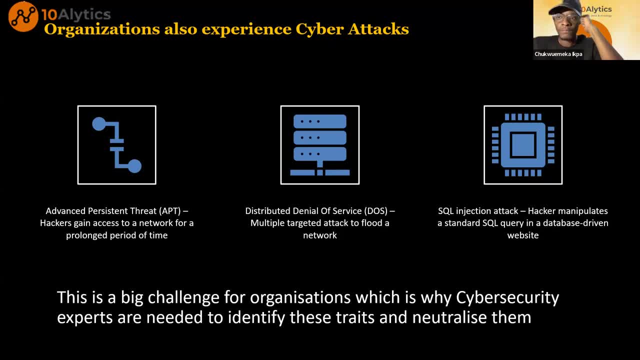 And when the criminal investigation guys would uncover them, they saw that they were a syndicate of China, Chinese guys, Cameroonians and they already. they have a company that they are operating. They have a young people that they were pretty, So they created a script for them and they were just reading. 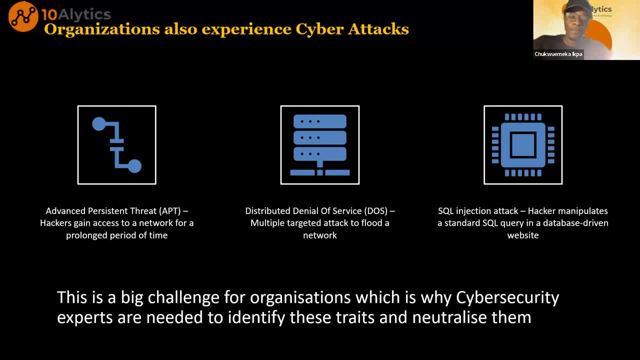 out all these scripts. see, you know calling people and maybe they use a particular number. They change the number and all of that. I know we've gotten those kinds of scenarios in Nigeria but based on the cyber resilience, cyber security experts and the actions they would. 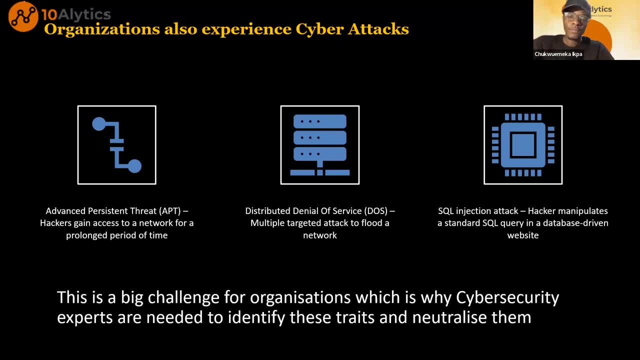 uh, that the expats took us. at that time, you were able to drive them away, because we're able to encourage the customers, We're able to create security awareness and all of that for them. So these are the things that cyber attacks will continue. 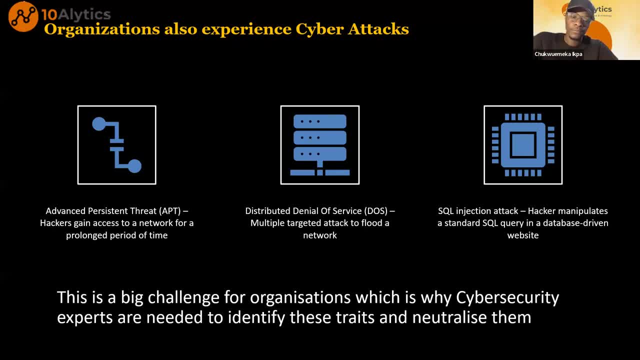 Cyber hackers will continue to do: when they discover that you've gotten their footprint in a particular location, they move to another location. So that is how they operate. So you can see how very, very important cyber security jobs and cyber security rules are there in. 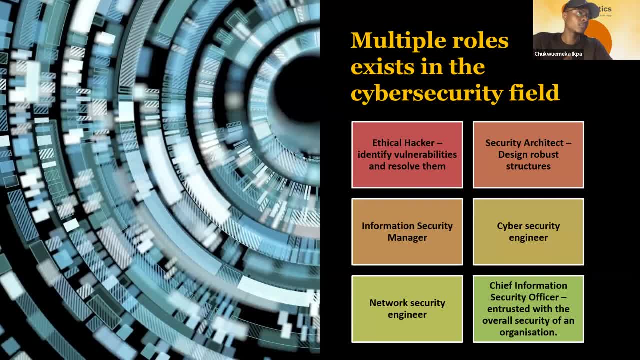 the industry. yeah, so i think we can move to the next one. yes, so this, this is a very this is a very interesting one. for me, it's very interesting part. this speaks to multiple rules that exist in the cyber security field. multiple rules that exist in the cyber security field. so, as a cyber security 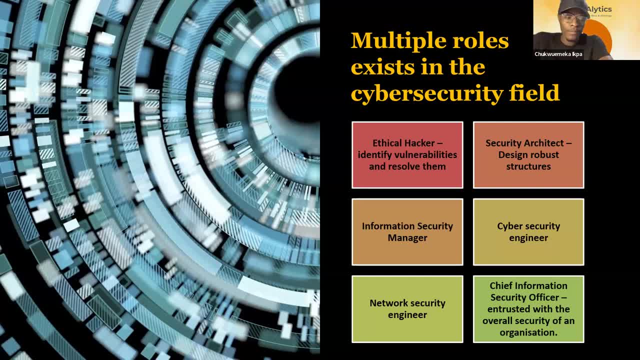 specialist. you can also be an ethical hacker. so what is your job as an ethical hacker? you can. all you need to do is identify vulnerabilities and immediately you can pick that there's a weakness in this particular application, or there's a flaw, or there's. it could be not. it could not only be. 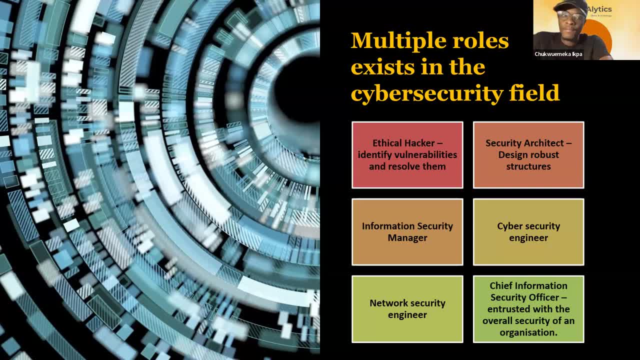 the application. it can also be a website or a program that someone is trying to develop in your organization. you can be working with your devops team, you can be working with your app managers, developers, and all of that before they go live with the application. going live means before. 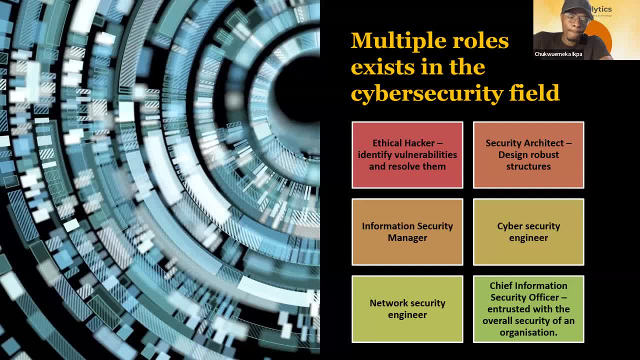 they launch their applications or before they've written so many codes- you you know you as uh ethical- before they even do all of that, you can try to identify flaws. you understand, do some vapt, vapt, vulnerability assessment and penetration testing and when you identify all these flaws, try to 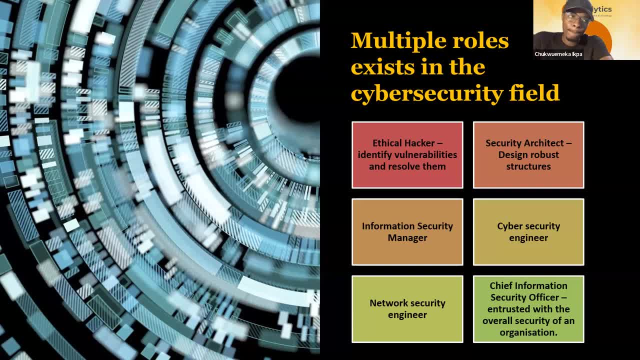 resolve them, give recommendations on how it can be resolved. you understand. so another role is a security architect. these are the guys that design robust security structures from the foundation, right from the foundation level up to the uh overview, up to every aspect, every domains in cyber security, ensuring that there is a security tool that is in place for every form of cyber. 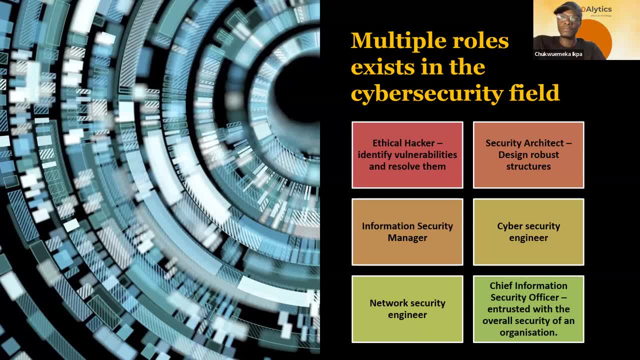 attacks. so those are the security architects. then we also have the information security manager. this role is a very important one because when you see uh, suck, suck in security operation center, you know we have four different levels in in in security and we are the security architecture. sock, you know it's not even captured here, but that is another rule, that's another fantastic rule. 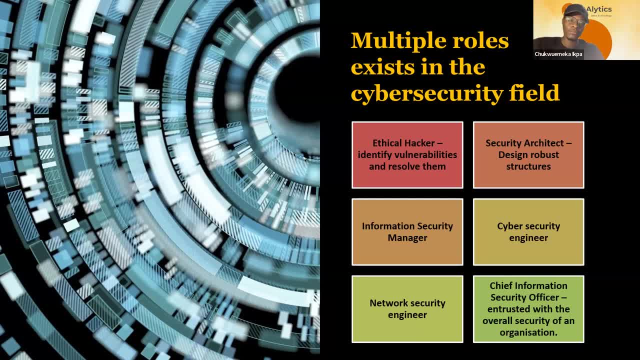 in in the cyber security industry. we have the level one analyst, we have the level two analysts, we have the level three, we have the level four. so the software are the ones. they call them incident responders or security analysts. you understand? the level two are like the ethical hackers. these 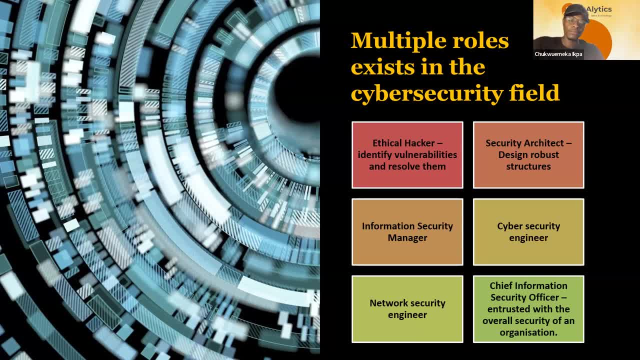 are the penetration testers. the level three is your um. is your uh escalation point? it could be your forensics department, it could be any form of uh um, of anything that has to do with root cause analysis, while level four is usually considered as a shock manager. so the information. 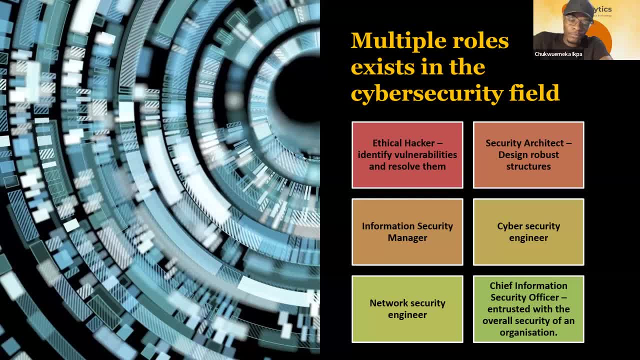 security manager are the ones that that um manage all security rules, security policies, security reports. you know you you'll be interfacing with your management team. you'll be talking to your cecils. the cecils are the chief information security officer. you'll be having the 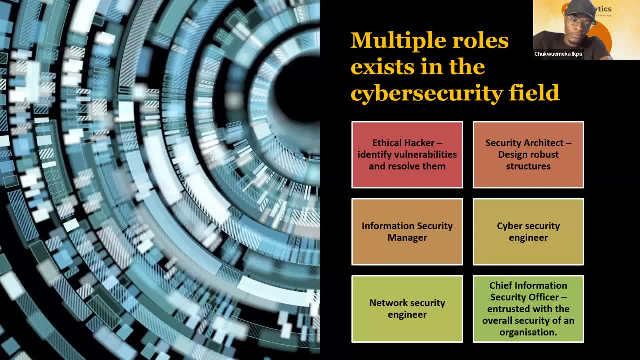 engagement with your cios, chief information officers or ctu or chief technology officer. you understand. so these are their rules. these are the things they do. they also advise based on security trends that is going on in their industry or in their country. they will give the best kind of. 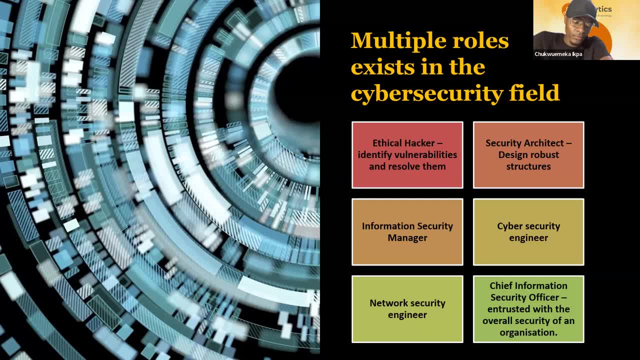 advice that the company can also take. you understand. so we also have this cyber security engineer. you know we have uh on-prem infrastructure and we also have cloud infrastructure. so as a as a cyber security engineer, you should be able to develop cyber security solutions both on-prem and on the cloud. 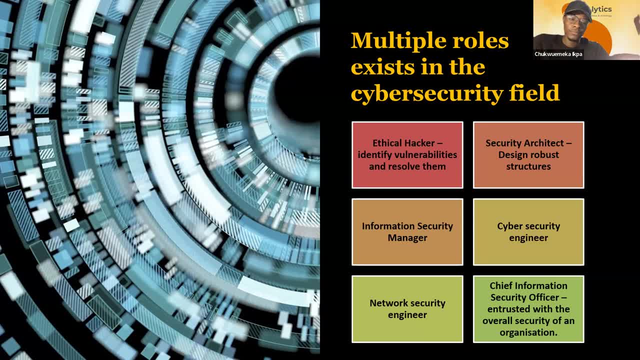 and this is their role. we have the network security engineer and these are the guys that make use of the meta exploit. they may ensure that their network security system is clean. there is no vulnerability on that level. you know, anything that has to do with that has to connect. 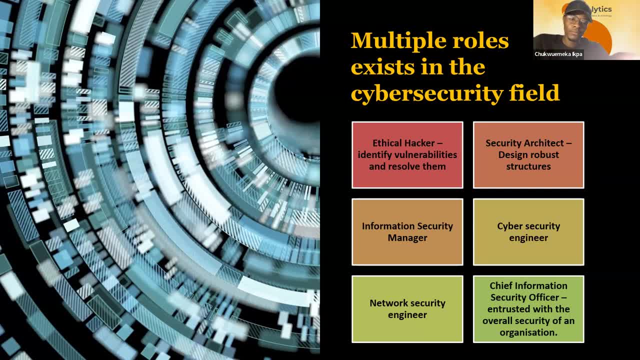 over the internet is properly managed and what are the kind of security tools you can use as a network security engineer and all of that. so these are, these are the functions of the network security engineer and the uh, the cso is like the top rule is the highest. 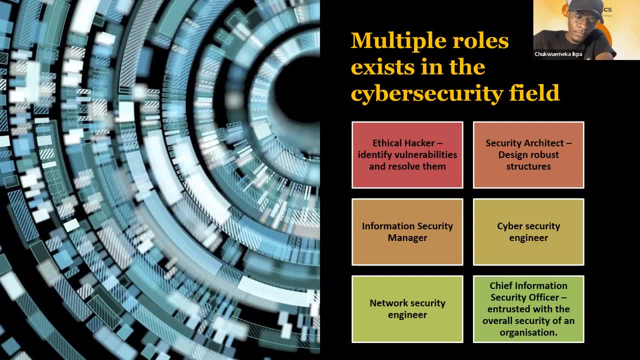 role in the cyber security field. you understand this person is entrusted with the overall security of an organization and they usually report directly to the nd. they report directly to the owner of the businesses because they make this the final decision on any cyber security policies and their major, their major work is to create. make sure you create. 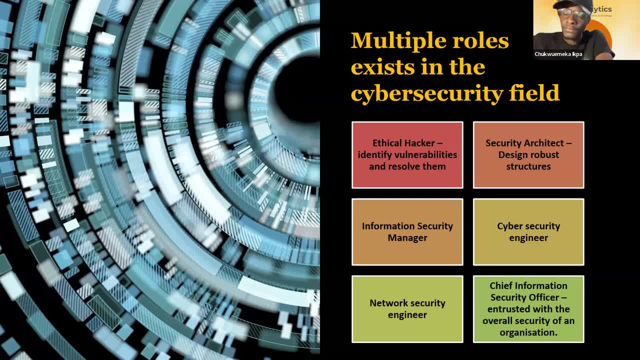 a security policy that fits into your, your company. you understand the kind of employees you have, you understand the kind of products you are selling and services, so you look at all of that and create security policies around that. you know, during the covet period we we have different forms of byod. 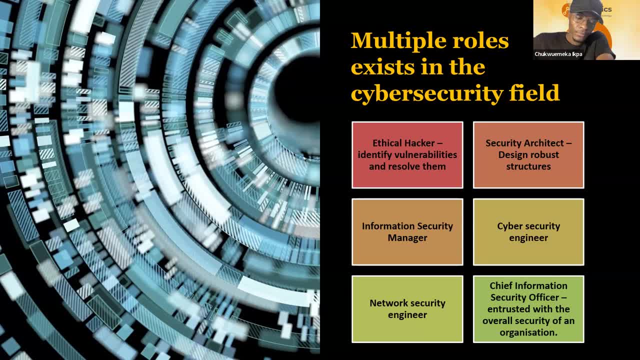 policies. bring your own divide policies. we have uh wfh, that is, work from home policies. we have remote work policies. these are the rules that the uh cecils are going to become creating. these are the kind of policies- security policies- they are to create and ensure that the 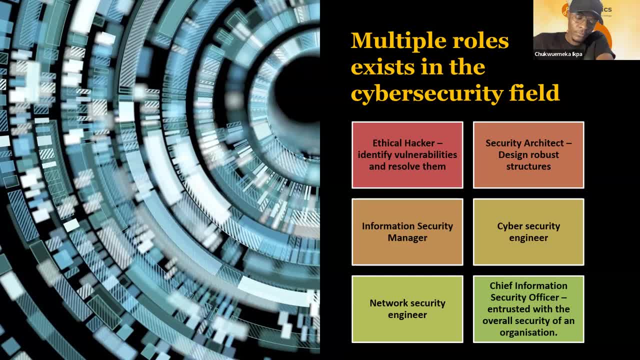 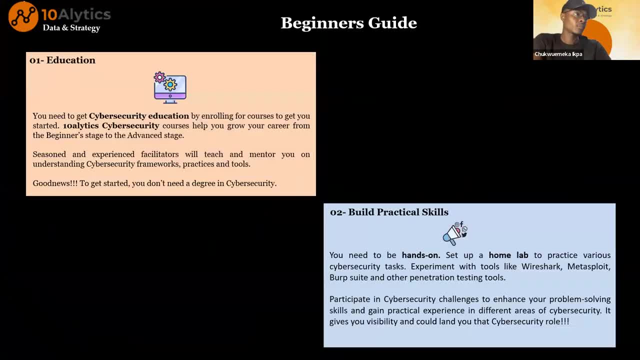 organization is in tandem with all of that. yeah, okay, so, um, i'll move to the next one. yeah, so now. this is a beginner's guide. a beginner's guide, so this is where i'll be taking you through, uh, this journey. you know 10? analytics is a fantastic learning platform that will help you, no matter, for. 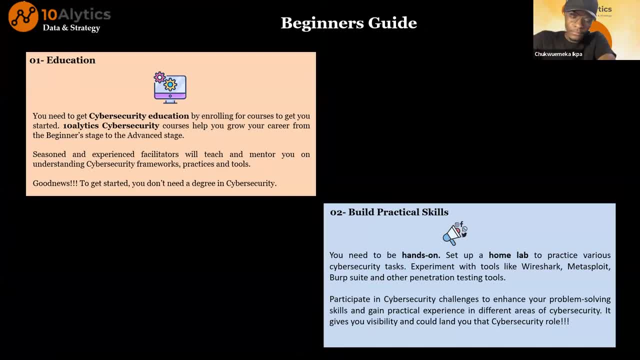 i studied mathematics and statistics and immediately after my graduation i didn't even jump into cyber security. i was into uh, telecommunications, doing contact center support, picking calls, nine to five, you understand, from nine to five. we started running shifts, doing it two, four, seven, explaining calling, taking calls from customers. i, i do uh um, that job for up. 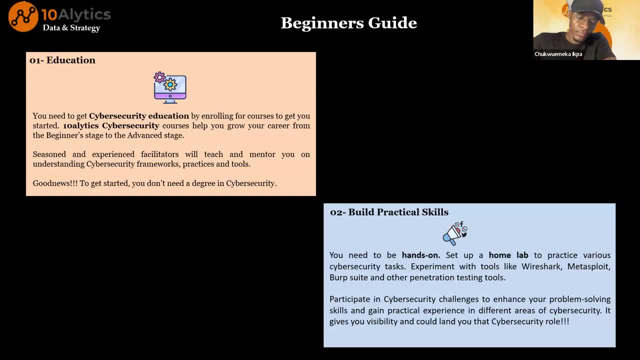 to a year. i was speaking because even when i, when i sleep, i can easily uh pick a nickel and attend to any customer. and the good evening, joshua. speaking, i may be available. we need to do this and all of that so, but that is. that did not uh debar me from getting into the. 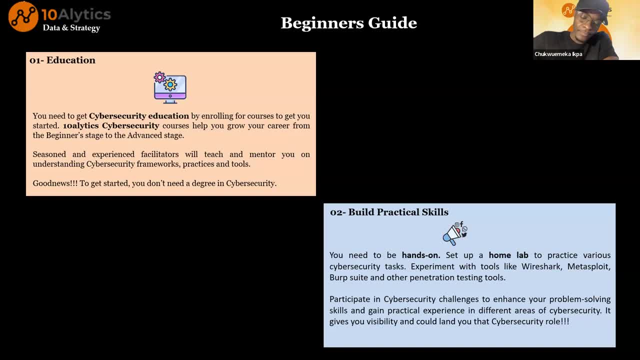 cyber security field. so i got an opportunity to work with access bank, where i learned a different banking um concept, different banking framework and all of that. i know everything about banking, so when it was time to be posted, i was just thrown. i i made some uh inquiry that i don't really, i just 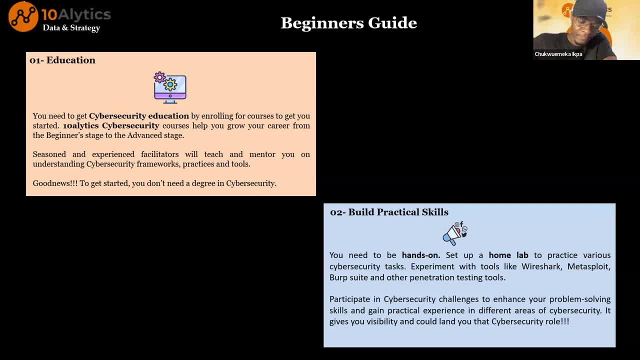 want to go into cyber security. i don't really know what to do in that field and someone advised me that i should just take uh, take the the course. take cyber security field and try to even look at platforms, look at different ways that you can improve on yourself. and let me tell you, since 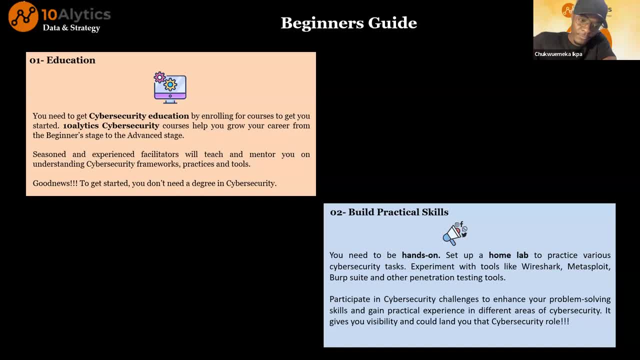 i joined that field. i've been learning and i've been having different uh insights. you understand. one very good thing about cyber security is: the more you learn, the more you want to learn more uh something about application security. today you'll be getting new updates on them, so that 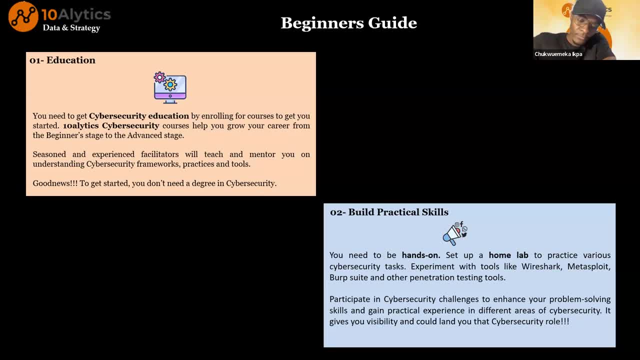 is why 10 and uh, 10 analytics is here for you, to help you, to guide you, no matter what your background is. so it's not compulsory. you have it background. it's not composite. if i have people that are into law, that you know the transition from law into cyber security and they are doing. 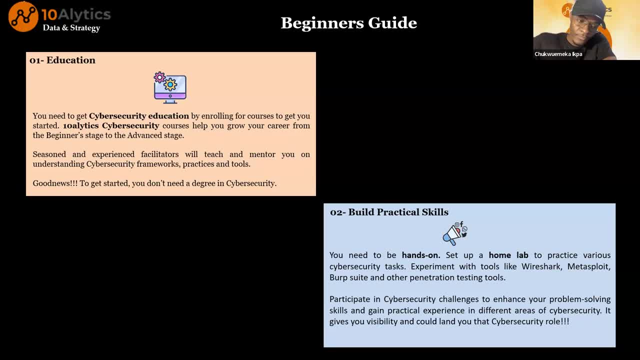 fantastically. they are doing well, they are doing great. so another uh area is build practical skills. You know why, on this journey, with 10 Analytics, we have platforms, we have Anson Labs- we'll be having different kind of labs that you can, as an individual- you can even set it up personally- you understand will help you to set up home labs. even after the training, even while you get a fantastic cybersecurity job, you can still be using these home labs personally to you know, to run different kind of simulations to see how it works in the real life scenario. you understand. 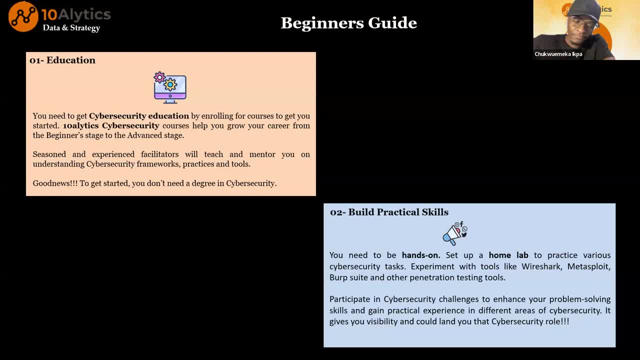 So we'll be making use of tools like Wireshark, Bobsuit, Kali Linux- you know, security tools that will help you, that people make use of on a day-to-day basis, you understand. So these are part of the journey and the beginner's guide. Yeah, please, you can move to the next slide. 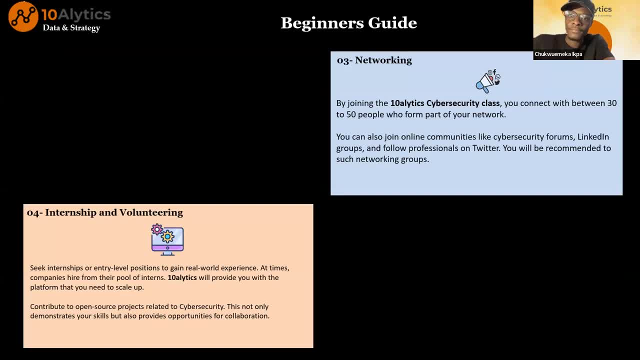 Yeah. so the third one is networking. You know we'll be meeting different people from different fields. you know, by joining the 10 Analytics cybersecurity class, you have the opportunity to meet up to 30, from 30 to 50 people from different parts of the world, from different networks, from different fields. you understand. 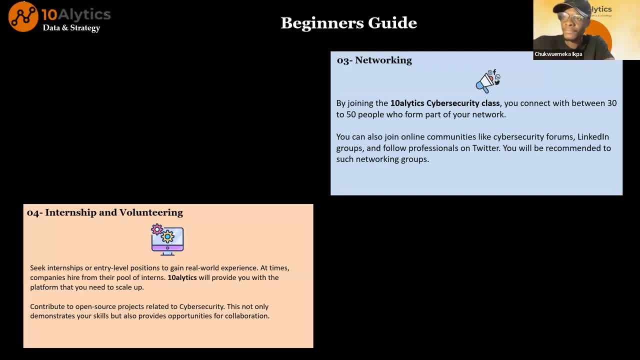 You can also join online communities like cybersecurity forums, LinkedIn groups. you know Professional cybersecurity handles that you can follow on Twitter. that we also recommend for you, you understand? So it's going to build your networking skills. like to meet with people and you have the opportunity to even chat with people. you understand. 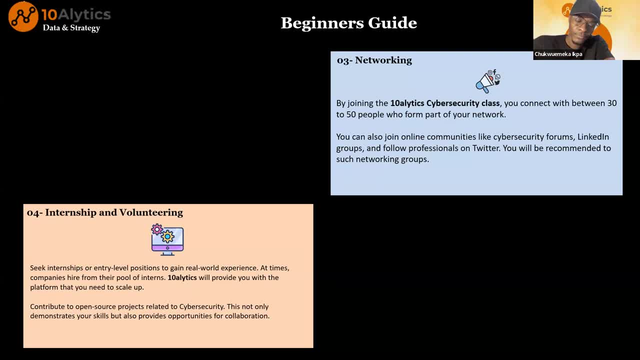 So you know that is what cybersecurity does. you know we have a community where we learn every day. you know, when you see new updates, new trends, like the scenario I just painted from Zambia is from one of the communities that I joined. you understand. 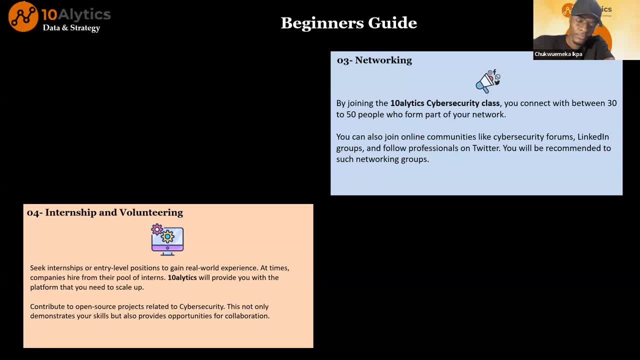 So you get information, You get up recent security trends, You understand. Then the fourth one is internship and volunteering, you understand. So you seek an internship for entry-level positions to gain real world experience. you understand. at times company hire from their pool of interns. 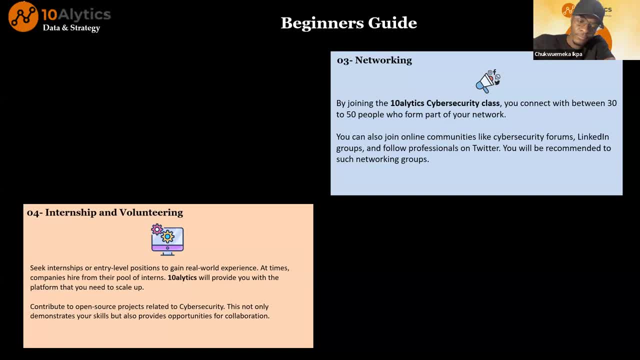 It's not compulsory. you start with an expert job or an advanced level job. But if you meet the role, if you fit in, you can start with that. but it's always advisable to even start as an entry-level job. But you know, it's always advisable to even start as an entry-level job, but it's always advisable to even start as an entry-level job. 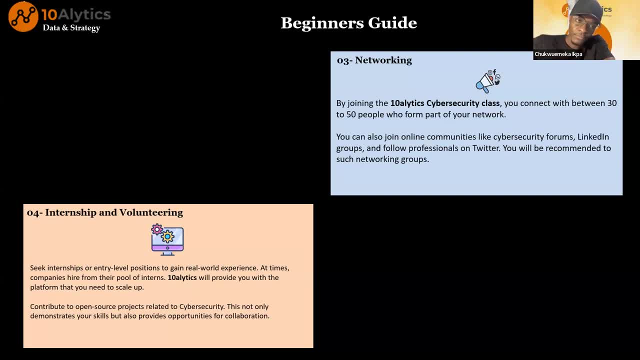 So you seek some of those Research's to afford for simple business positions. as easy work to do, It makes a difference. I know I've seen information, an entry-level position or intent. you understand 10 analytics will provide you with the platform. 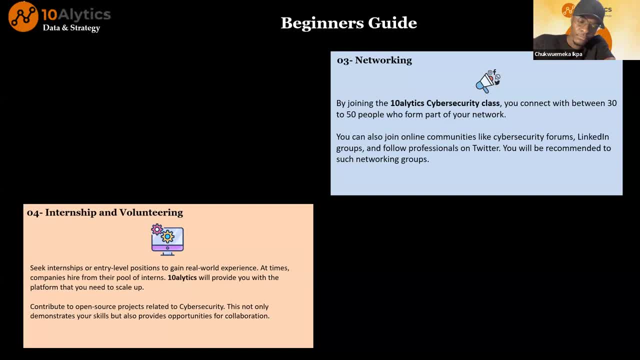 that you need to scale up. it's a very fantastic one, you understand, so. contribute to open source projects related to cyber security. this not only uh demonstrate your skills, but also provides opportunity for collaboration, and these are what uh employers are looking out for. you understand- people that are ready to contribute even before they get paid, you understand, so these are what. 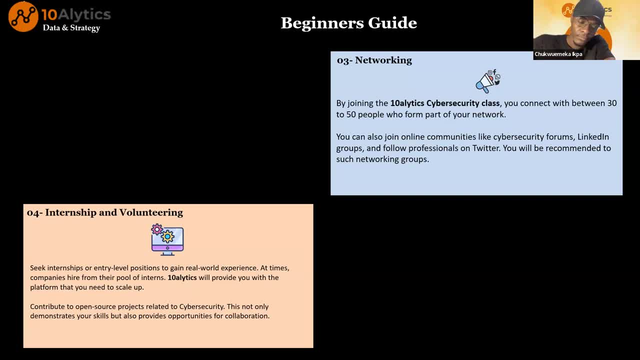 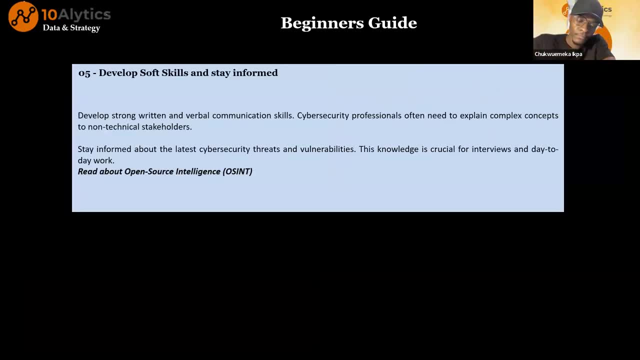 10 analytics will help you in achieving. yes, please, we can move to the next one. okay so, and another very important area is um: develop soft skills and stay informed, you understand, so we can have different cyber security professionals, like, for example, in my field. i know we have many, uh, cyber security experts, cyber security professionals, but what? 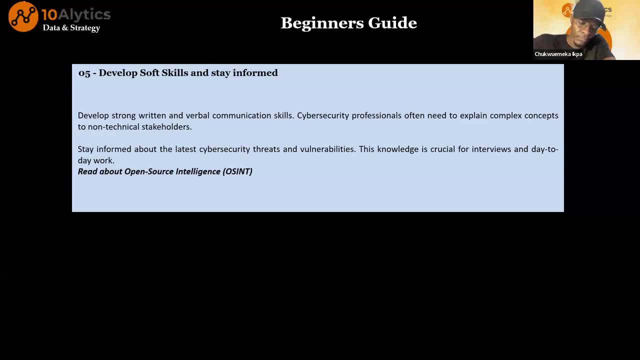 will make you stand out is your soft skill. you understand how to manage people, how to explain concepts to non-technical stakeholders, how to sell security tools. you understand how to engage people to let them know that, okay, this, these are cyber security flaws, not making them uh look very stupid. you understand, but 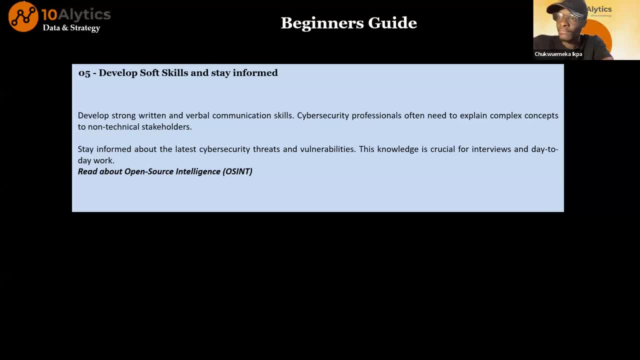 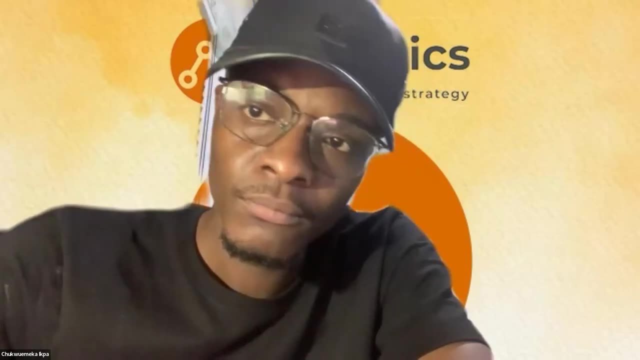 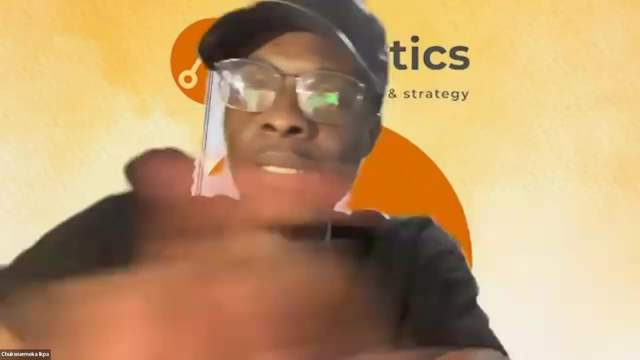 just trying to explain to them, trying to bring them up to speed. you understand, stay informed about the latest cyber security threats and vulnerabilities. so these are the kind of uh 10 analytics will also be providing for you. so this knowledge is crucial for interviews and for day-to-day work. thank you very much. all right, all right, yeah, okay, thank you so much. 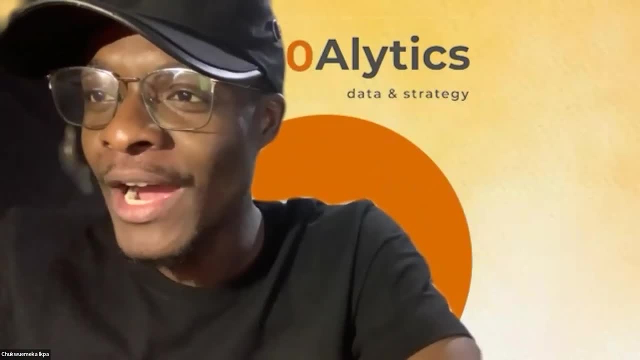 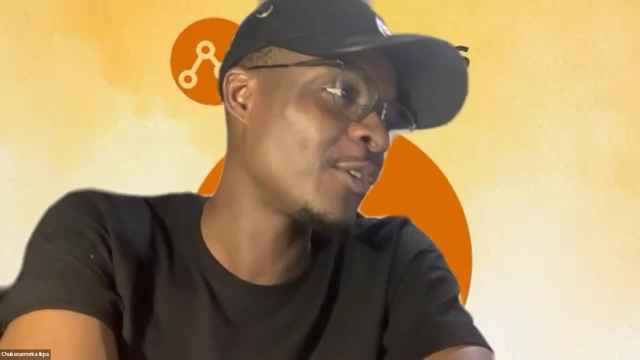 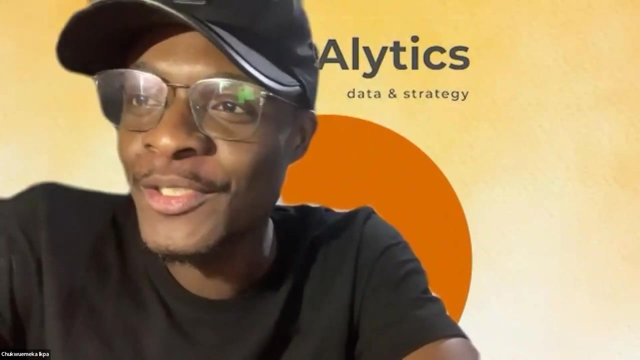 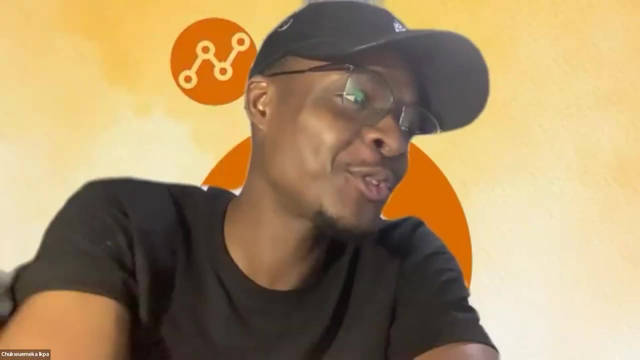 joshua, hi, um, i'm. i'm right there, hi i'm. i can't share my screen. i don't know what just happened. hi, elijah, hi lydia, my screen just went off. please, you can hear me. just, uh, confirm that you can. hello. so, thank you so much, joshua. joshua has walked us through a great deal of how we can. 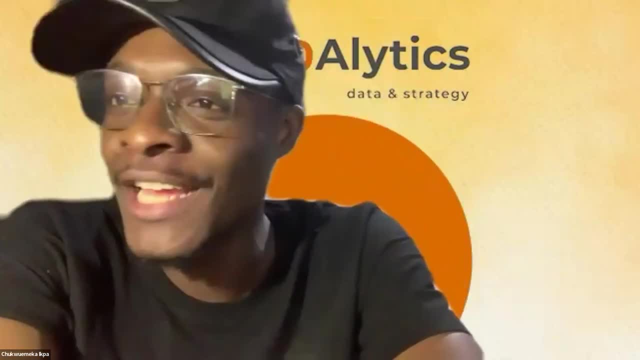 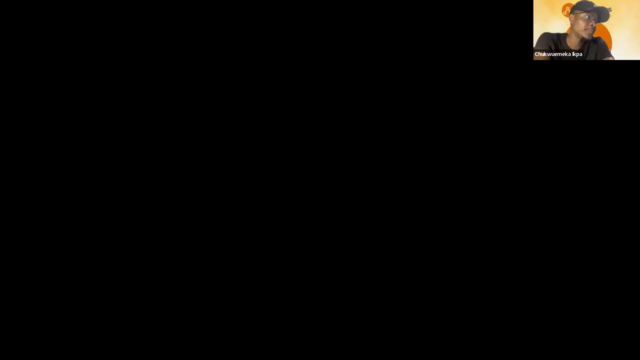 get started in cyber security. hi, lydia, please reach out to elijah. i can't share my screen, i don't know. okay, yeah, it's coming back up now. all right, thank you for that. okay, so, uh, joshua has walked us through a great deal of. 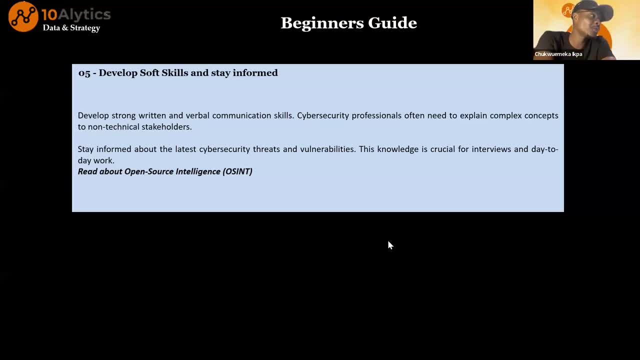 how we can do all this thing right. so before we move on- joshua- i know you wanted to be able to, you know- show us a small demo. i stayed there, joshua, yes, please, all right, so you have the flow right now. yeah, if you are still following us up to this moment, please drop a one so that 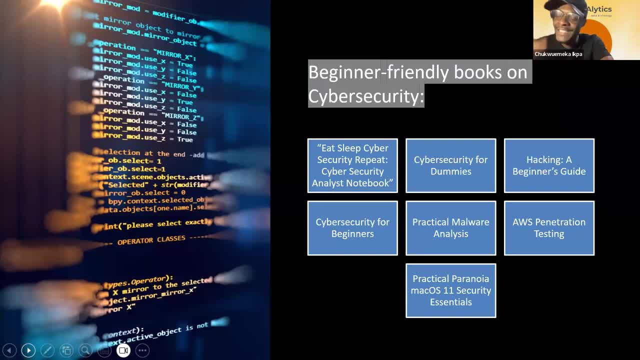 we know that we are talking to people. if you are still following us up to this moment, please just drop a one in the chat box so that we can continue and be able to know that you are following us. okay, so please just drop a one, just drop a number, just drop a fire in the chat box so that we can know. 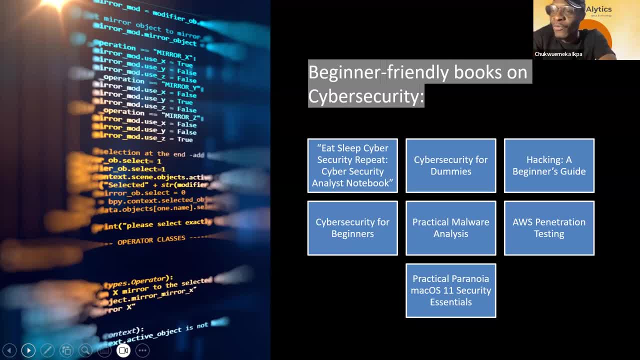 that you are still here with us. fantastic, i can see a couple of ones, amazing. all right, joshua, i have the floor. please fire on. all right, thank you. please confirm if you can see my face. i'm turning on my video right now. okay, amazing, it's good of you to show us your face. finally, joshua, thank you. 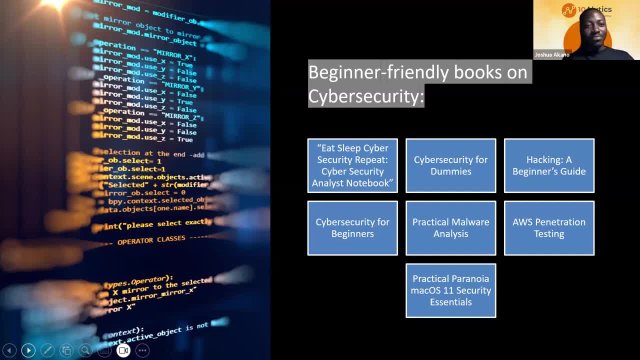 no, no, it's not yet up. okay, it's not yet up. okay, yeah, we can see you right now. amazing, amazing, we can see you now. thank you, all right. please go ahead, joshua. all right. so before we uh get into some uh lab sessions, just to showcase one. 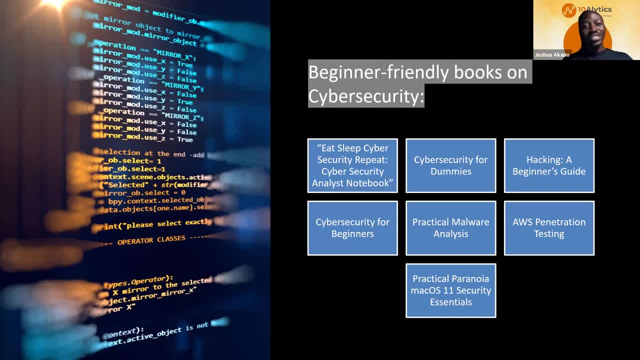 or two things, uh, it's also important to know there are some beginner friendly books on cyber security that can help you to kick start this journey, you understand, and the one one of them is eat, sleep. cyber security repeats, you know. so you can get it in amazon stores. 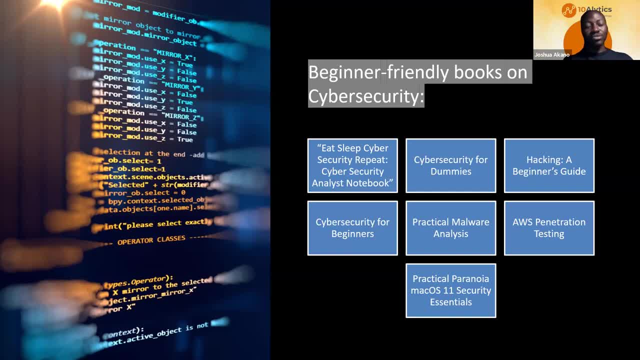 you know, these are books that give you a background on what to know. you understand starting a career in cyber security. you understand it. so what i tell people most time is that just make sure you get resources, you get books and as you spend more time in it, 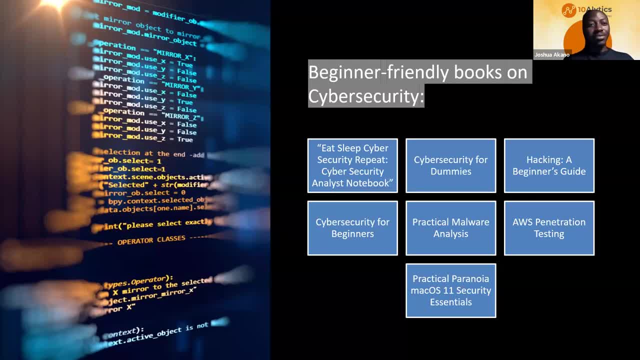 you begin to see all these concepts as a normal day-to-day activity. you understand so, and also, it's always very good to have a networking background. but these are the things that 10 will help us in achieving. another book is cyber security for dummies. we have hacking- a beginner's 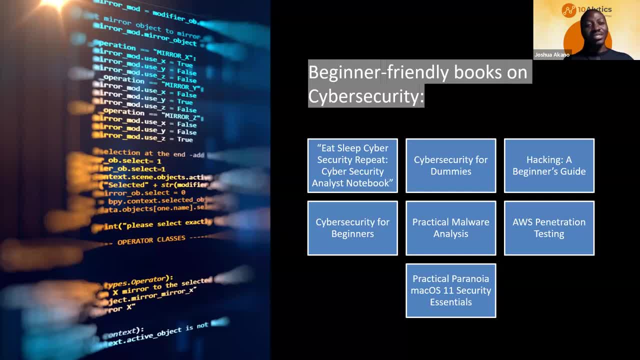 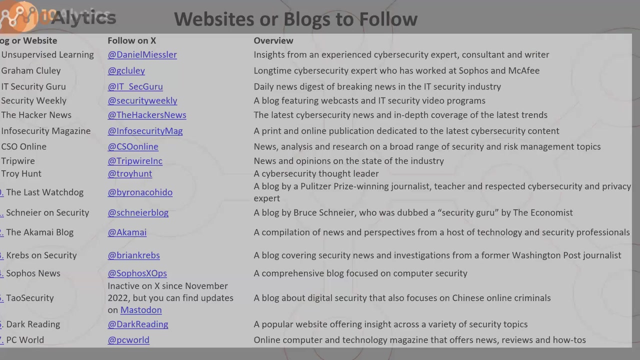 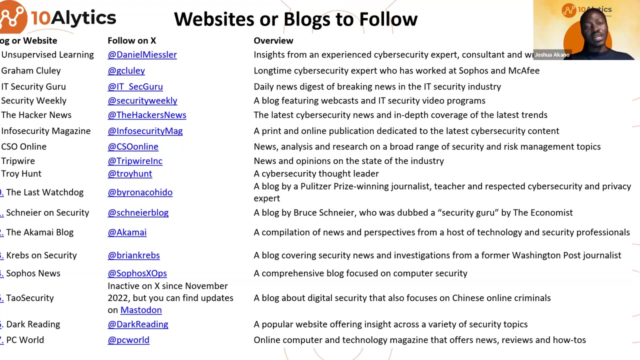 guide: cyber security for beginners, practical malware analysis, aws penetration testing, practical paranoia, mac os 11 security essentials. so these are different books that can help you to get started. yeah, all right, so i think we can move to the next one now. yeah, so, and these are some uh interesting uh blogs and handles on x that you can follow. 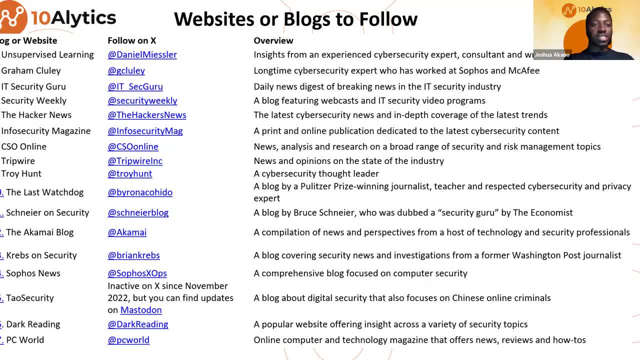 you understand, uh, i've listed them here. you can also share them with you, maybe after uh the session or the master class session. so these are uh important. um, uh handles. that gives you a blog featuring webcasts and it security video programs. you know you get up-to-date analysis. 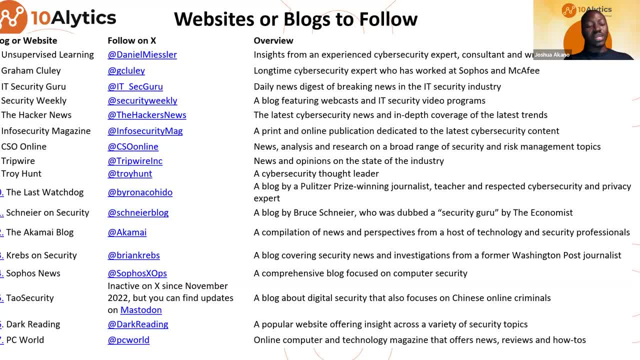 of security trends, security incidents. you get vast in it, you understand. so some of the interview questions you get are usually related to: okay, what's what's going on in? maybe you're applying for a role in germany- and you just ask: okay, what's going on in germany in the cyber security space? 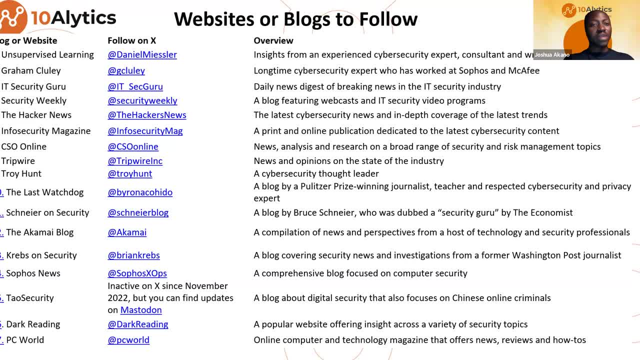 or which country are you currently applying from? okay, applying from canada. you're applying from nigeria, you're applying for? so they want to know what's the current uh security incident that happened, you understand. so, following all these um handles keeps you. uh. there are more, but i just 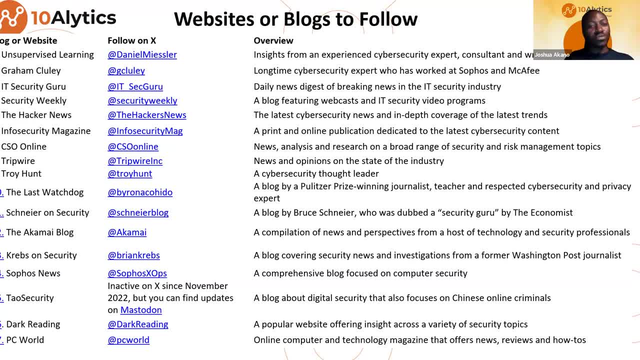 limited it to this so they keep you informed. they give you uh, up-to-date information and all of that you understand. so you can. it's not necessary you follow all of them so you will not be too overwhelmed. you can just pick like two or three. you can scan through any of them and see the one. 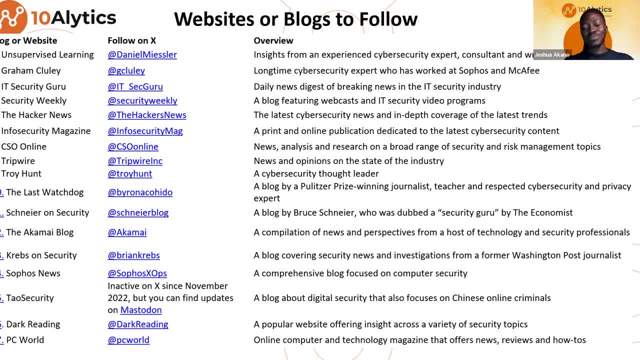 that uh fits what you're actually looking for. yeah, so i think we can move to the next one now. okay, so i think we can move to the next slide. hi, can anyone hear joshua? yeah, can you hear me? yes, joshua can hear you. all right, all right. 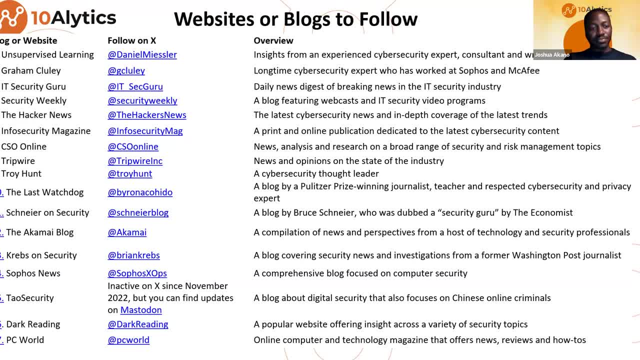 so, uh, you can move to the next slide. okay, all right, so let me, let's just go straight to the uh anson labs. so it's just a simple. it's just a simple uh test to see how our email addresses are doing. if our email addresses are fine, you understand so. 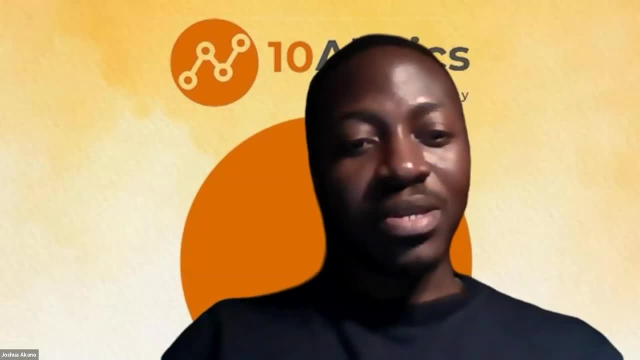 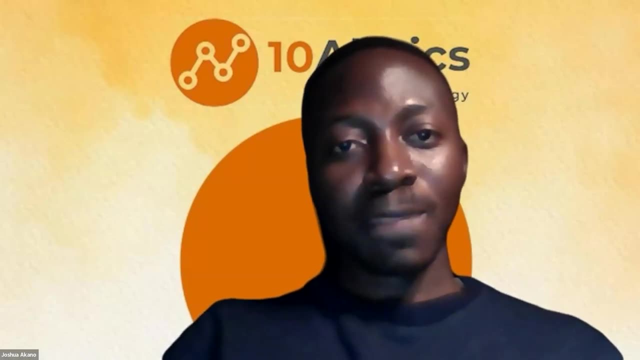 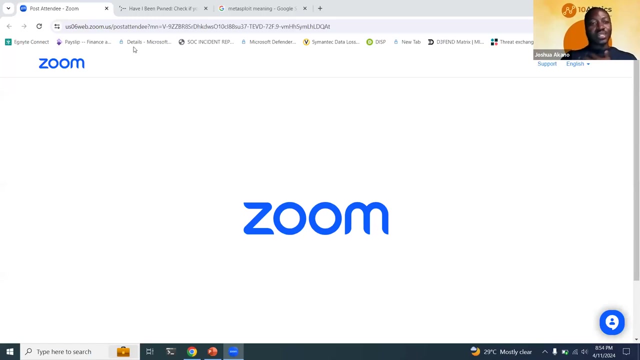 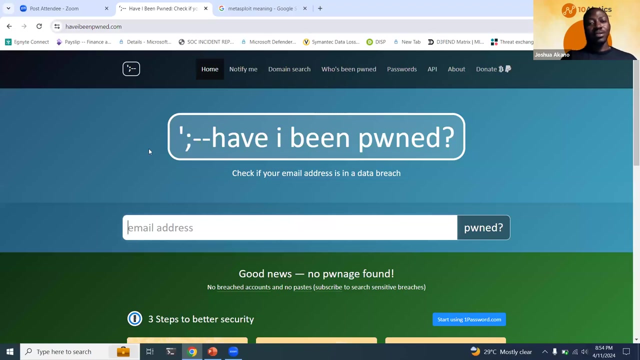 it's called. have you been pawned? you know, let me share my screen from here. they do. let me know if you can see my screen. it's popping up. popping up here is the uh lab session and the url is a vibeon pointcom. understand, so you can also. 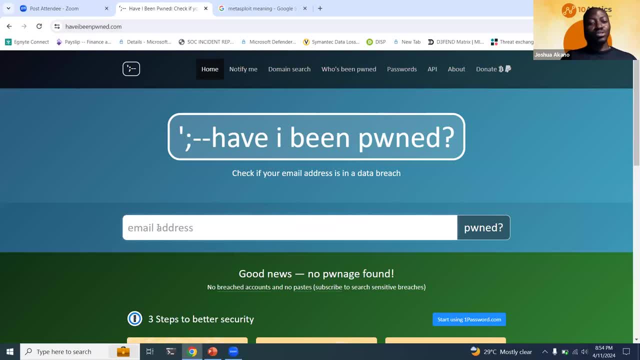 practice this when you are alone. so what? what do you want to achieve? we just want to check if uh email addresses have been uh detected for any compromise, or maybe our passwords have been detected in some sites that have been hacked and you know there are some breaches and all of that. you understand, so i'm going to test with my contact screen. you understand, so i'm going to test with my contact with me community. okay so, and so no one knows the answer. but yes, so if you know a link up, something around тö, mitOOOO, tighten to system, have an engagement so that your contact will be strong and to connect to content. start, provided contact level will be there and content focus: end of sale. you need something to do. you already show a text to me and that is. you know i've been planning months, oh and so along those dates we will let others click. so in the chat and now, 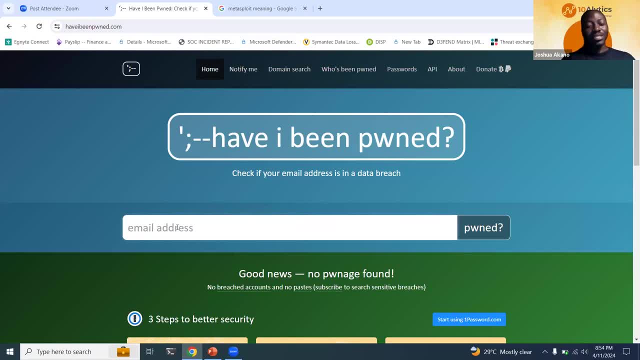 my own email address first and i will get different email addresses from the platform from the session. you can just drop your email address on the chat and we'll just help you check if your email address have been pawned or have been detected in any compromised website. so 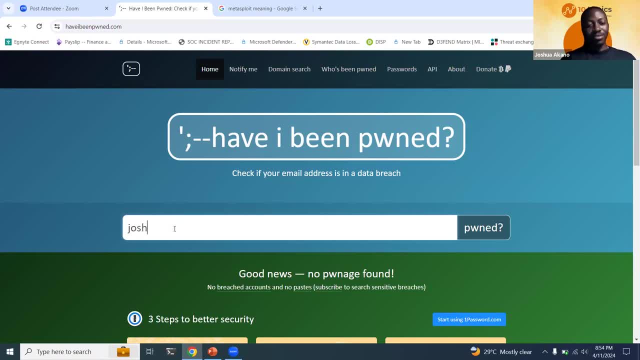 let me start with mine. i'm going to use my yahoo mail, just your email address, that's all. we don't need the, the password and that's so. it's searching, wow. so this is the result: good news: no pawned found, no account and no paste subscribe to search sensitive breaches. you understand so this. 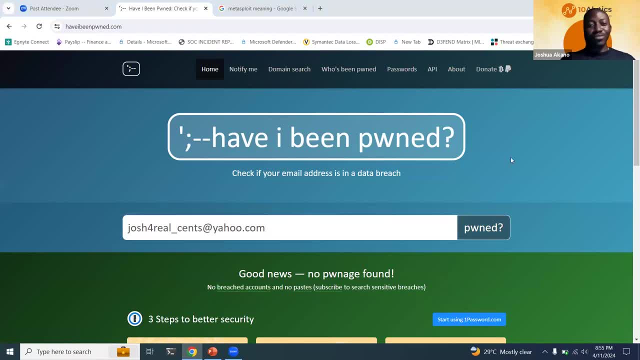 this is the result you get, so let's see if we have anyone volunteer. oh, nice, nice, okay, let me start. okay, let me start with um. let me start with techno. okay, i can see, i can, i can see michael, all right, oh, fantastic, okay, let's. let's start with um the zoom user. 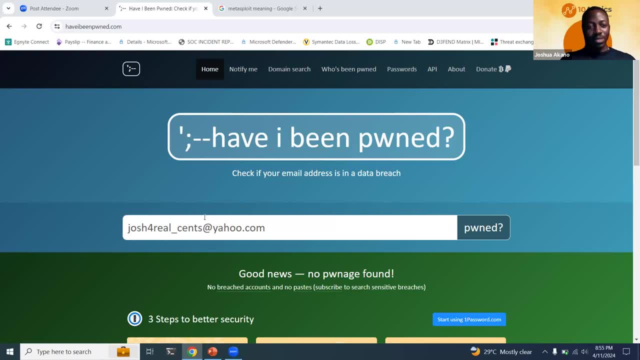 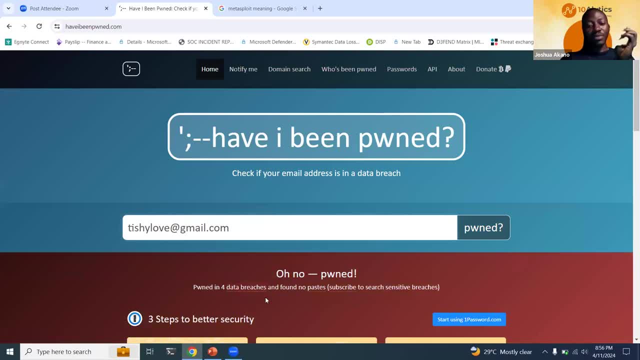 but your email addresses has been found in four different data bridges. So what does this mean? So it means maybe, okay, you try to log in with your email address to a particular website or to a particular platform, To a particular website or to a particular. Yes to a particular platform that has already been compromised. You understand. So what you can just do is, first of all, there are recommendations here, but just make sure you change your password. Avoid using simple passwords like this. You understand. 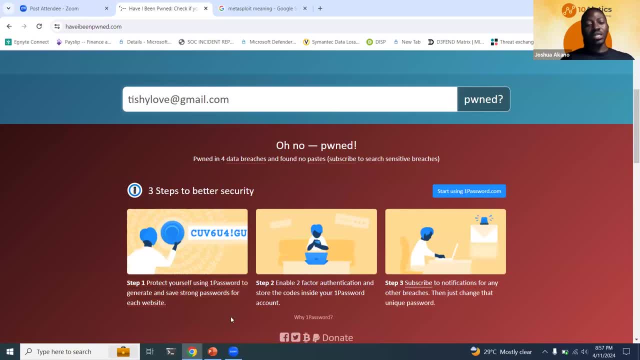 Avoid using simple passwords. So make your password complex. You understand There's something we call password complexity, You understand. So you look at the number of characters in your password. Is it up to eight? Is it up to 15?? Do you have symbols in your password? 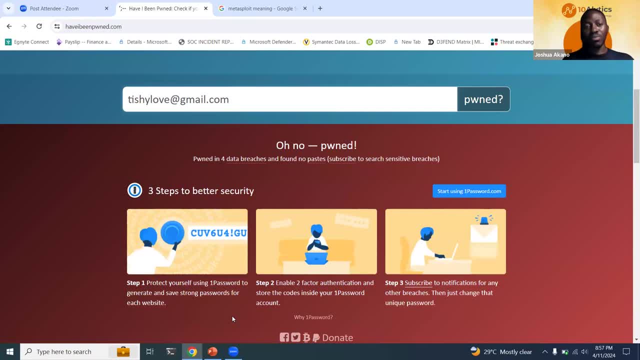 Do you have characters? Do you have numbers in your password? Do you have uppercase- lowercase? Can you even create a paraphrase And say: okay, my name is Uyeng Bing Pei. I create something from it, You understand. 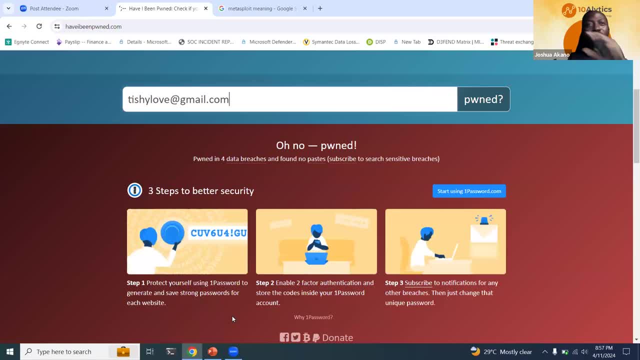 Oh, I love Bing Pei. From there, you can change the I to one, You can change the E to number three and stuff like that. You know, just play around your password. Another thing is ensure that you make use of 2FA. 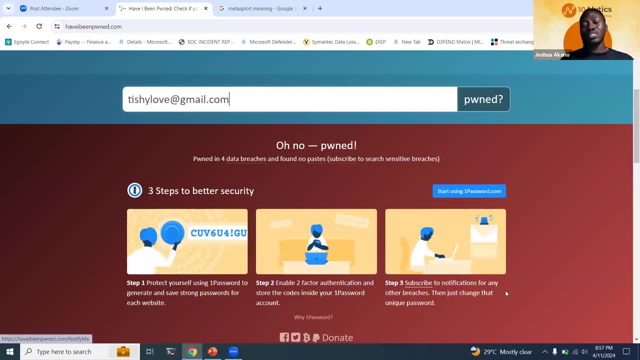 You understand: Ensure you make use of 2FA And also ensure that you do not use the same password for different platforms. You understand: You are using the same password for your Gmail. You are using the same password for your Facebook, for your Instagram, for your Twitter. 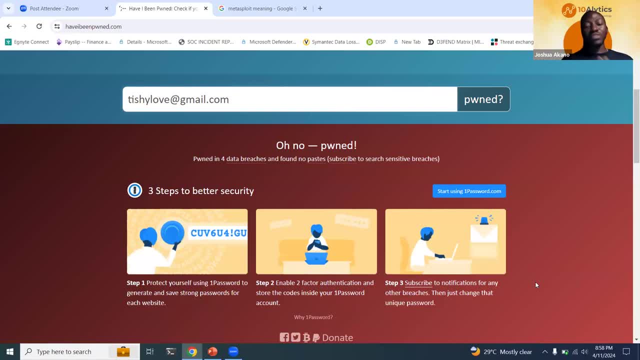 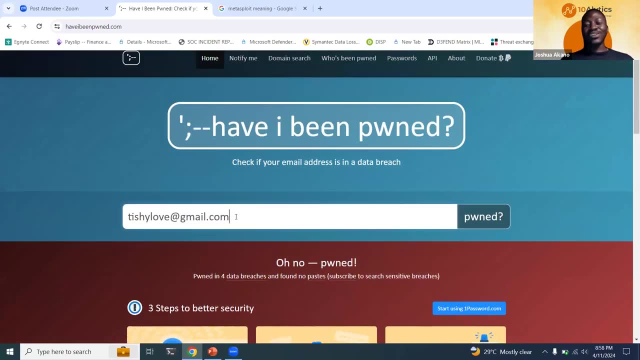 You know all of those scenarios. Ensure you have different passwords for them. So this could be the cost. And it's not a bad thing that it happens every day, You understand, Because websites get attacked, get compromised every day, So it could be anyone. 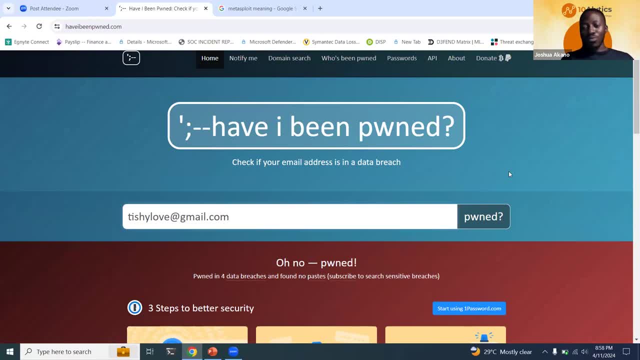 So let me just try to check another one: Taewoo Mac controller. Okay, Okay, let's see, let's see, Okay, so this also has been. So I wanted to say maybe the Yahoo guys are the safest, but no, this is another one. 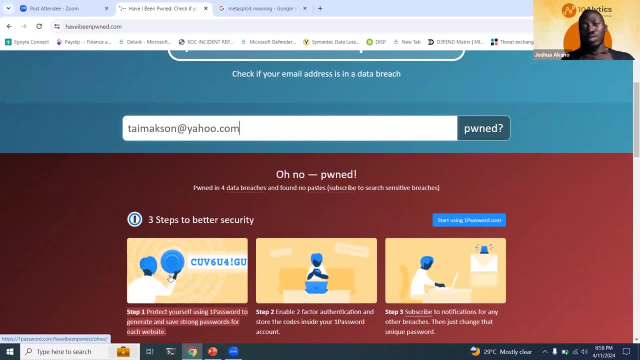 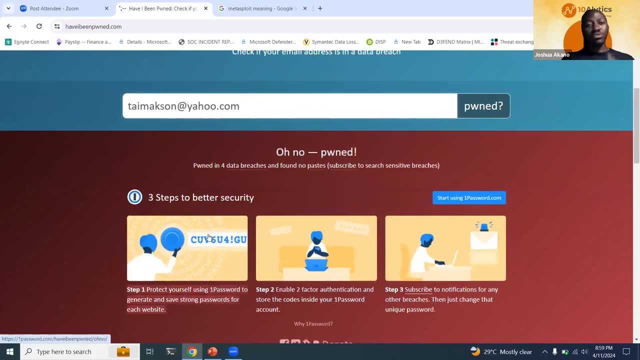 So just the same thing I explained to Bing Pei, So it's the same precautions you should take. First of all, just change your password. It means maybe your password If your password is weak, and all of that you know. you know there are also URLs. 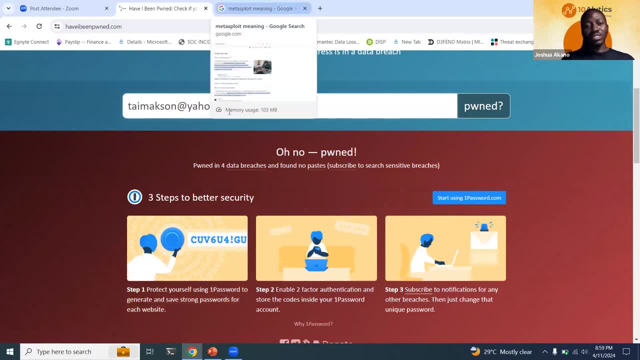 There are also platforms where you can check your password strength. you know, even apart from checking your password strength, security has gone beyond just password and username. you can enable 2FA. You understand. 2FA means two factor authentication or MFA. 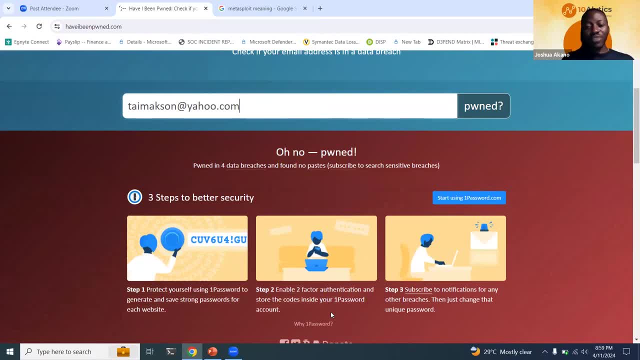 It means multi-factor authentication, So you have different kinds of security layer. even if your username and password are very weak, you still need to 2FA, you understand, And 2FA can be your OTP. OTP means one time password. 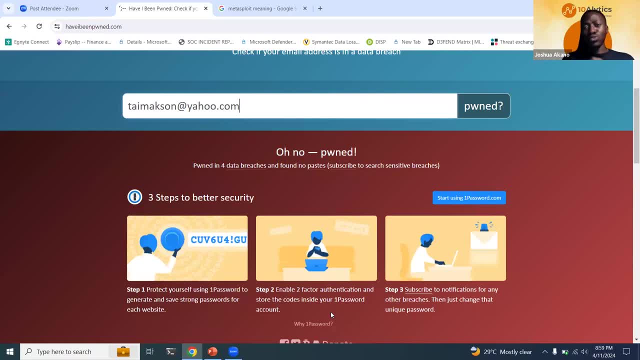 It could be your fingerprints, It could be what you have, It could be what, who you are, It could be your islands and all of that, So it could be different forms of security. We also have tools that you can use to manage password, that they can also help. 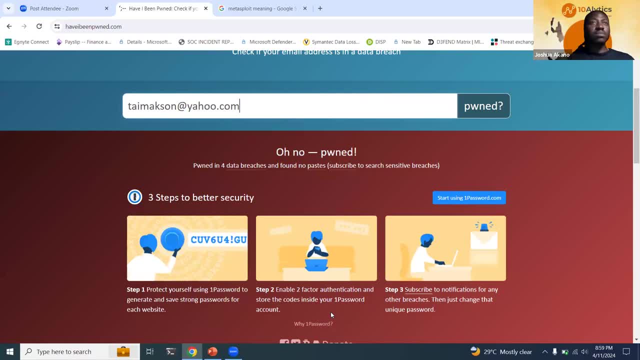 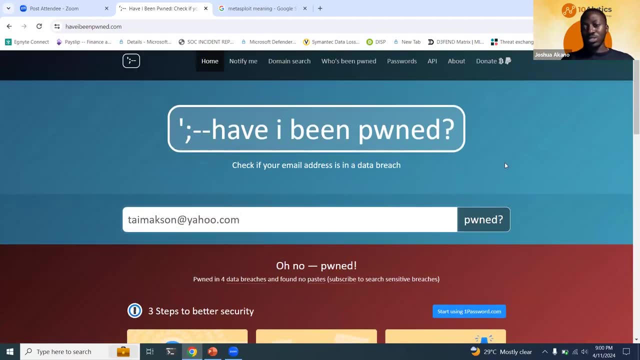 Instead of entering your password directly, it gives. it sends the password automatically to the website. So, depending on how best you want to use your email, you understand. So let's Check others. I think we've only seen two or three. 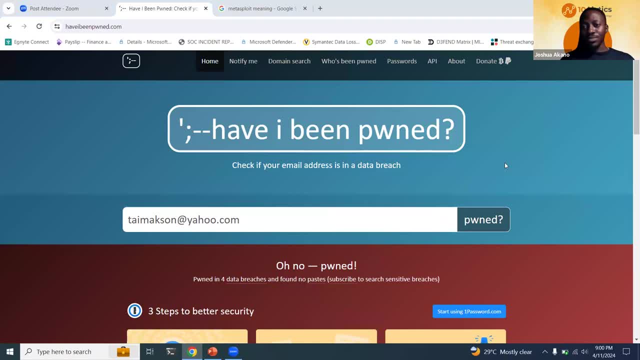 Let's see Chukwemeka. Let's see Right, So this is okay. Good news: No, no point found. So, uh, I think this is a good one. So let's see another one is a good one. 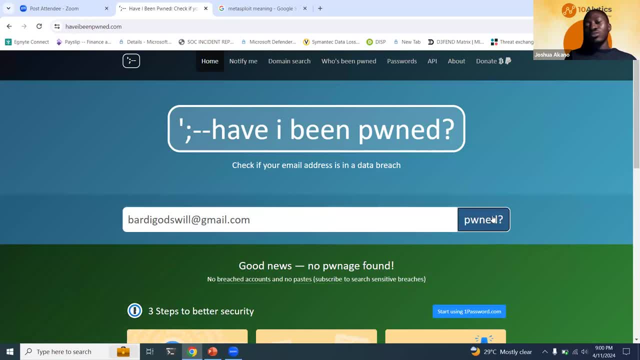 So it just speaks to: um, I will make use of our email addresses, You understand. So this is another good one from God's will in Stan. So it's. it does not mean because your uh email address is clean today. 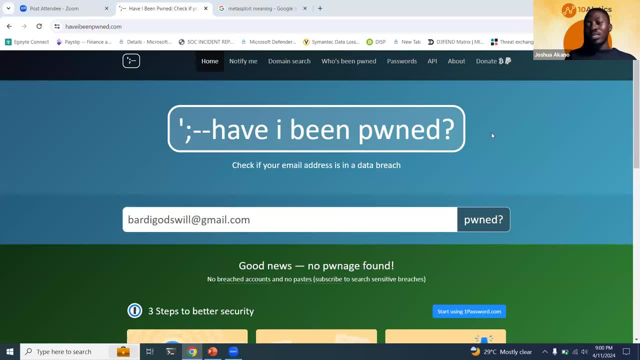 That can be act tomorrow. So it depends on how you use it and the platforms you register them on. So you remember I said nobody's a hundred percent secure in the stance. So our tax every happened every day. And just the first precaution when you see that your email address has been. 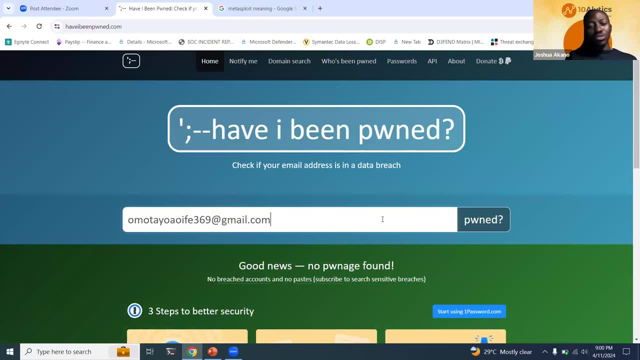 pawned. first of all, change your password immediately. So this is also a clean result. So it's not too bad for you to be able to. you know you can. you can check your email address on here and it makes a lot of sense. 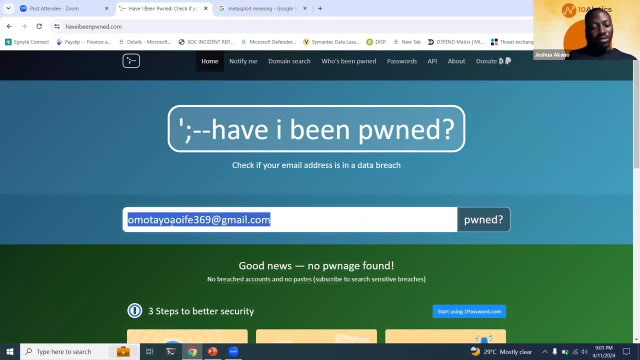 Yeah, I don't think this is too bad for for for Omotayo. Let's check for God when. So I'll do like five more so we can move to the next uh Discussion. So, Michael Gordon, wow. 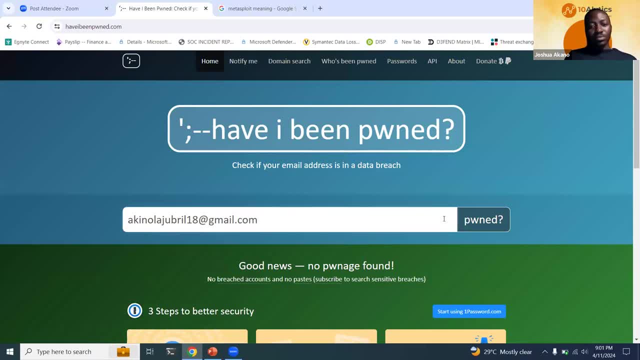 This. this is good. Okay, Let's see for. Okay, so this is another one. So you can just ensure you change your password immediately. You can change it immediately after this session. Ensure you are making use of a complex password. 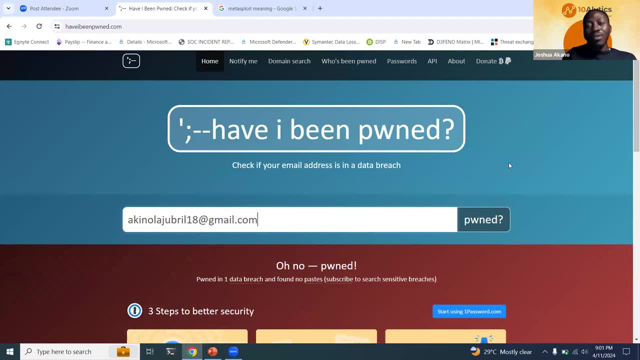 Use paraphrase. Don't just make use of a word. Use a paraphrase Like: just say, a sentence or a short clause that makes meaning to you. Then change the letters. Change some of the letters to numbers. You can even include parentheses. Include some special characters that are not. 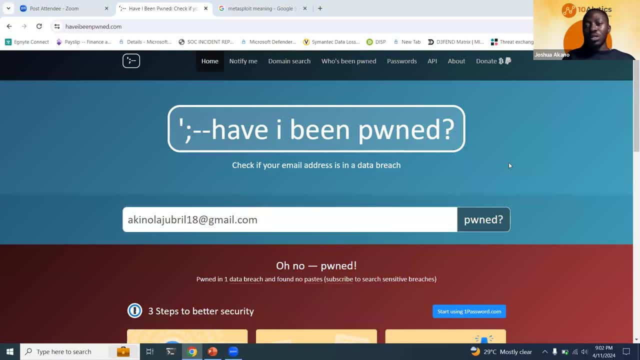 really common And you can make use of password manager tools, Password manager tools that can help you keep your password. If you are the type that you have up to 14 different accounts that you log into every day, this password vault, this password manager tools, 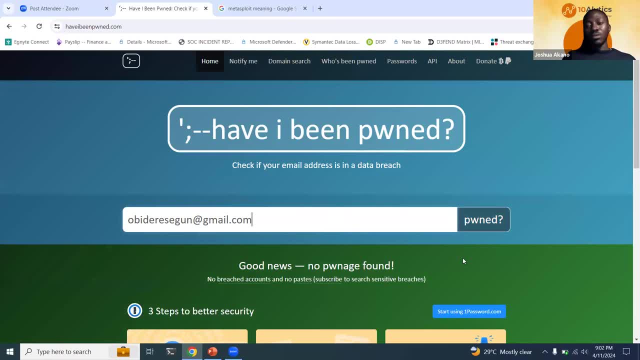 can help you with all these kind of scenarios. So this is a sharegoon. I think sharegoon is good. Okay, So we've checked chat. Let me just pick one more: Random, random, random, random. Okay, Let me pick this. So. 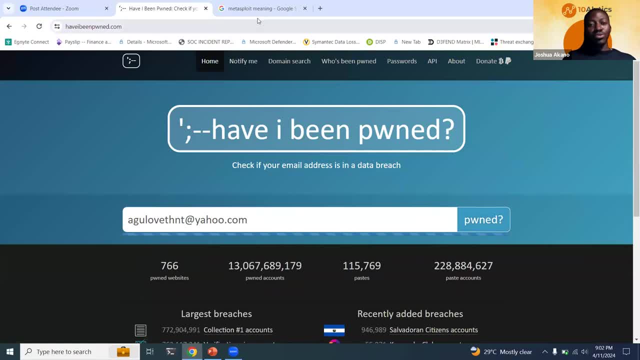 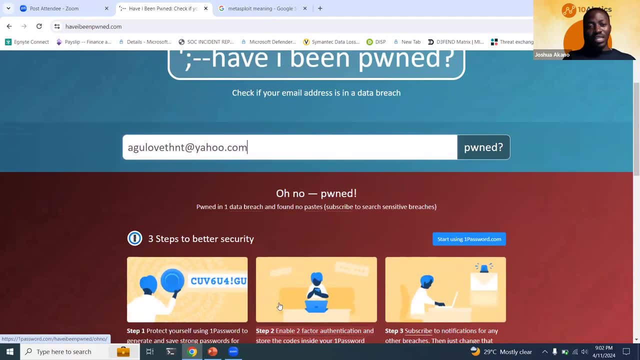 this should give us a clear result, So let me just quickly give us a bonus URL. Oh wow, This is a one data bridge, Okay, Okay. So, as I've said earlier, just ensure you quickly change your email password. You can change your password. You can change your password. 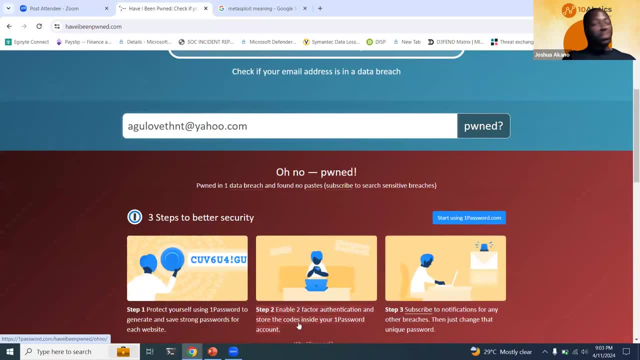 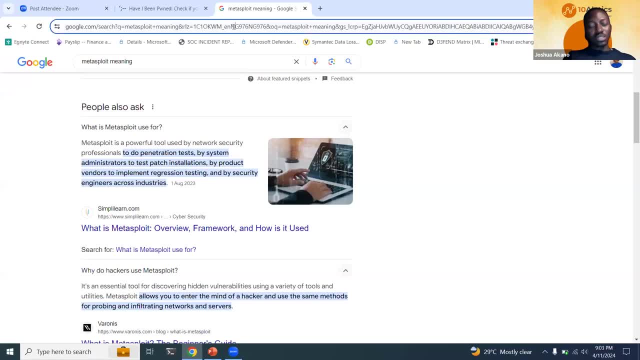 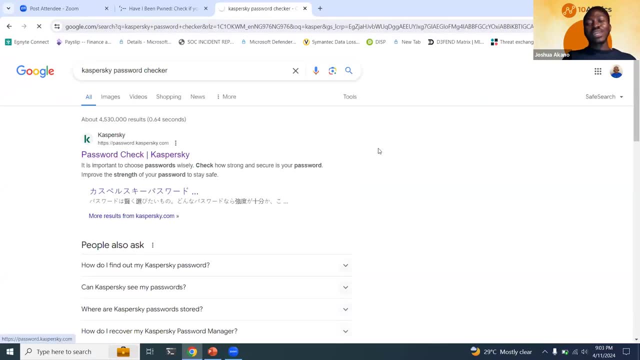 on your email and all the websites. So let me just give us this bonus: You can check this on our own, privately. So I want to encourage you to put a password on the chat So I will help you check. You understand. So you can just check the kind of the strength of your 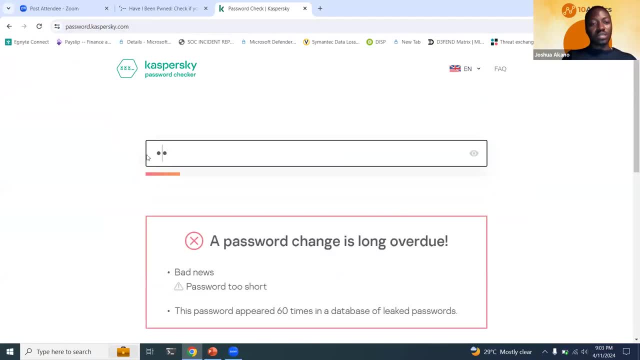 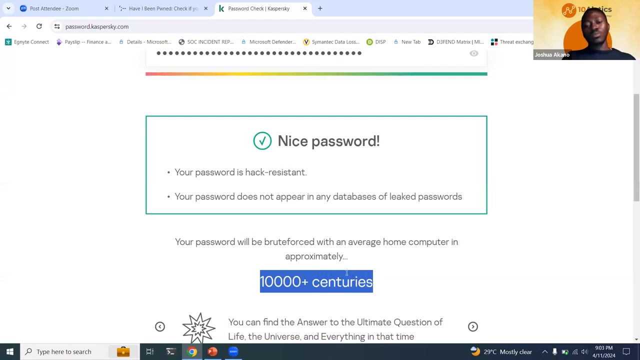 password on this. So this site is good, You understand. So let me just put an example of a password. okay, so let me just stop here. oh, nice password. see the years it will take for it to be cracked. can you see? 10 000 plus centuries? you know that that's not, uh, possible, you understand. so this can. 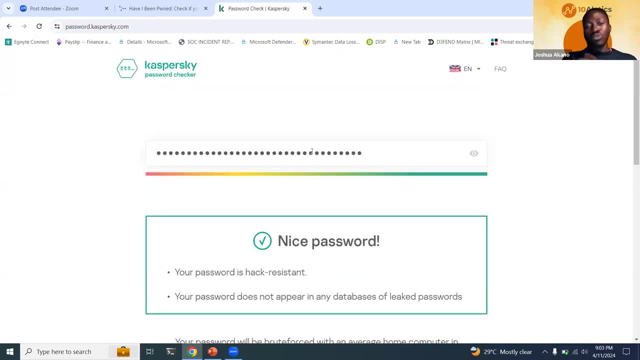 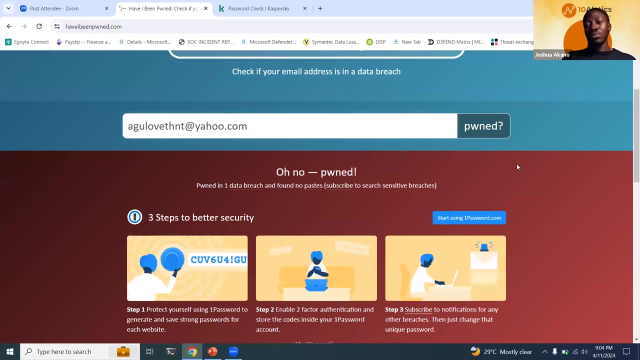 just give you an hint on how uh password complexity works, so you can just let me drop the url. maybe at your free time you can just check it up, look it up and you know we'll be getting more of that in uh trainings and all of these best security practices that can help us. yeah, so i think uh. 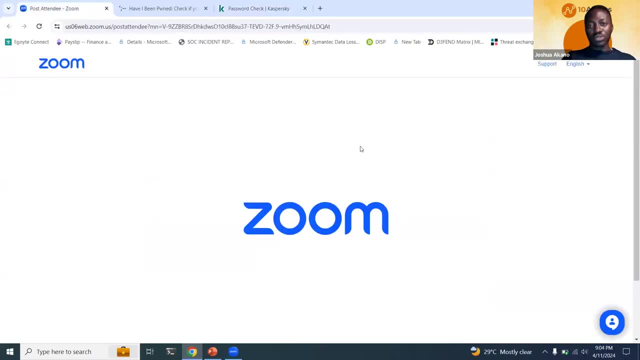 that's that from me, thank you very much. okay, all right, thank you so much, joshua. thank you so much, joshua. please confirm that you can still hear me. joshua, can you hear me? yes, yes, perfect, perfect, absolutely, all right, amazing, amazing. if you are still with us up to up to this stage, it means that there is 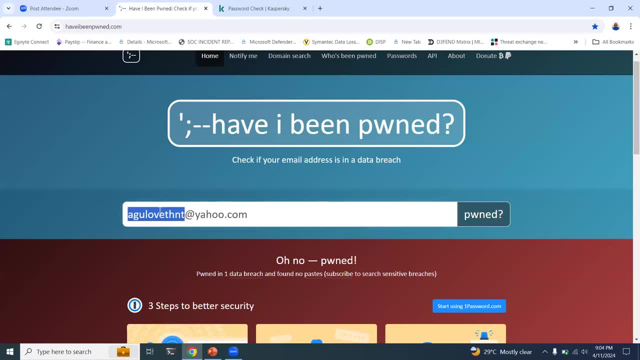 something amazing that you are getting. we've briefly touched on how to check whether you've been pawned, whether your email has been pawned, or whether your password is something that can easily be hacked, and how long it will take it to be hacked. now we want to get into the other. 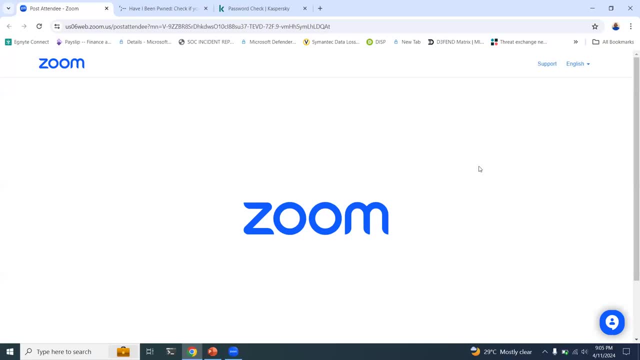 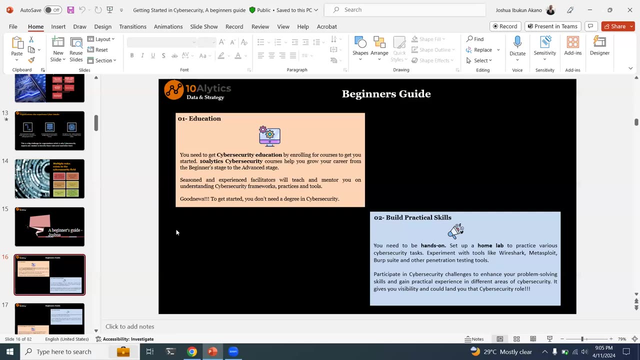 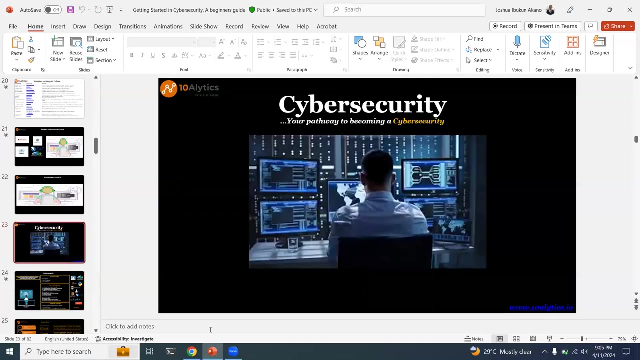 section to tell you how you can easily transition into this tech ecosystem. right, you want to get into analytics? how can you easily get into this space? hi adam, if you are still there, please allow me to share my screen. hi, adam, please allow my second device to share my screen. all right, joshua. um, i don't know. 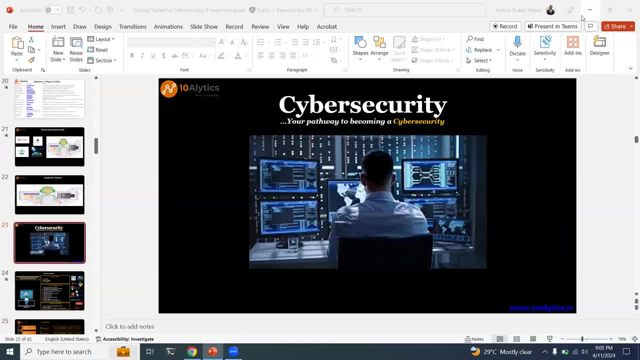 you can keep on why adam gives me the host privilege also. okay, okay, absolutely all right. so, um, basically, we want to walk you through the pathway to becoming a cyber security expert. right, what can you do for you to become a cyber security expert? all right, so, um, joshua has. 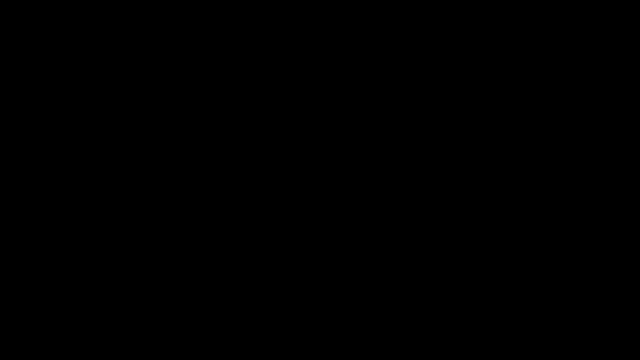 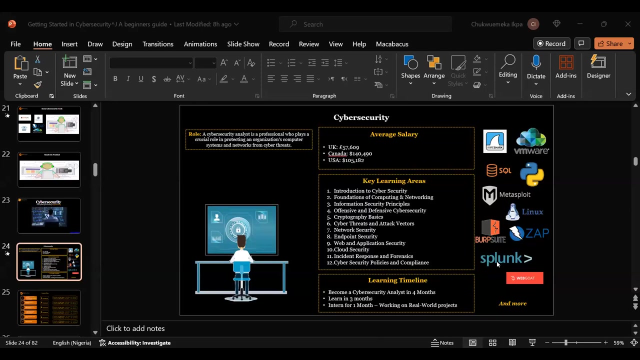 touched on a lot of things that we need to know right. he's touched on basically two sites that we can use for some of the tools that cyber security analysts use on a day-to-day basics, and i walk us through the other area of how we can get started with these um tools: how do we? 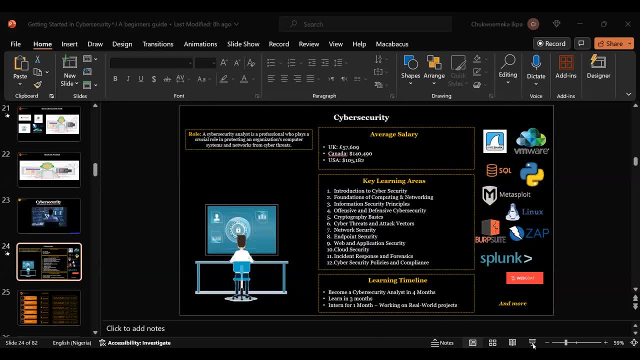 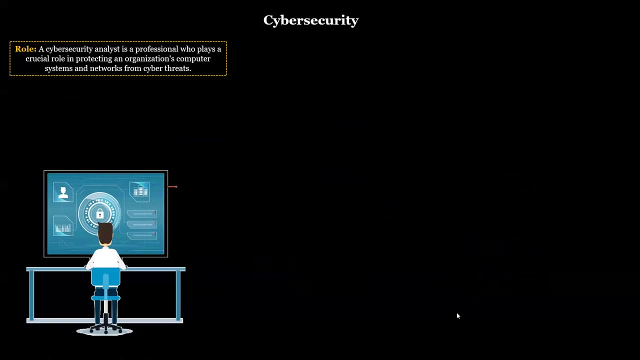 get started as a cyber security expert in this exact terrain. what and what do we need to do to be able to say, okay, comfortably: i am a cyber security analyst, i don't need to- um, i don't need to explain who a cyber security analyst is anymore, because i believe we all understand who i. 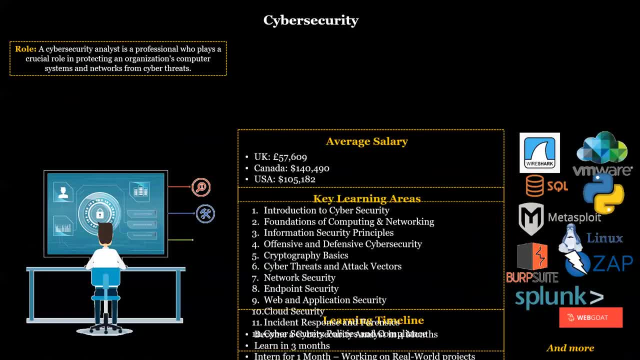 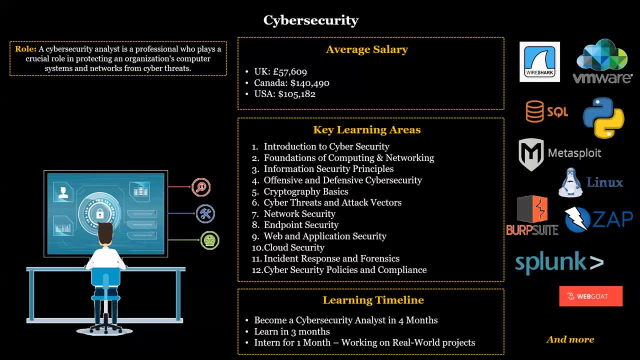 They are from everything that we've talked about today, right? So, basically, in analytics, there are key areas that we are going to walk you through, right, And it starts with your introduction to cybersecurity, right So, even if you have zero knowledge about cybersecurity, like Joshua mentioned, the first level for you to the first beginner's guide for you is to have education. 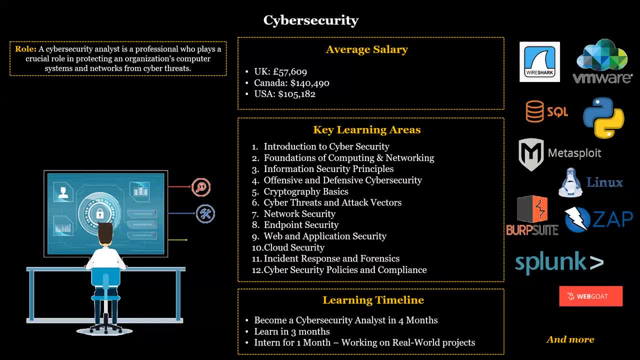 And the next one is to have hands-on practicals, And these are things that we get to offer you here at Analytics, starting with introduction to cybersecurity. So, even if you have zero knowledge of who cybersecurity is or what are the cybersecurity principles, we get to introduce you to this right. 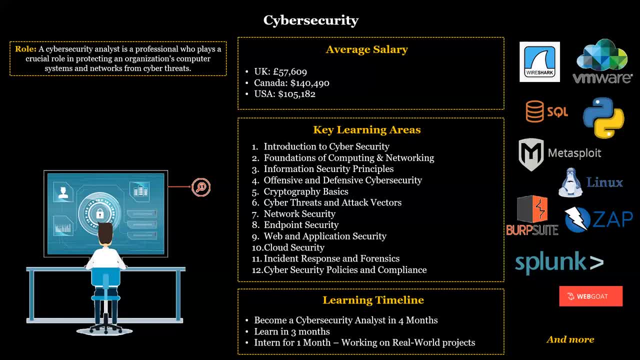 So you also get that theoretical knowledge and also get the practical knowledge so that you can defend yourself anywhere you find yourself. So from that introduction to cybersecurity, we'll walk you through foundations of computing and networking where you get to understand, okay, what is LAN, what is WAN, and then we'll move you to information security principles. 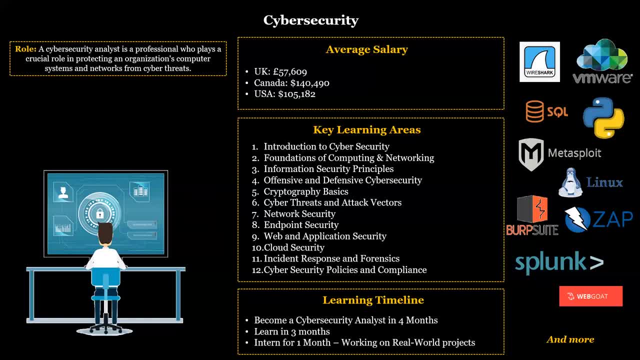 Basically for you to be an information security expert, what are the principles that you need to know? What are the CIA triad, which is basically confidentiality, integrity and availability of information right. This is basically the triad. It's like the foundation on which all the principles that you get. 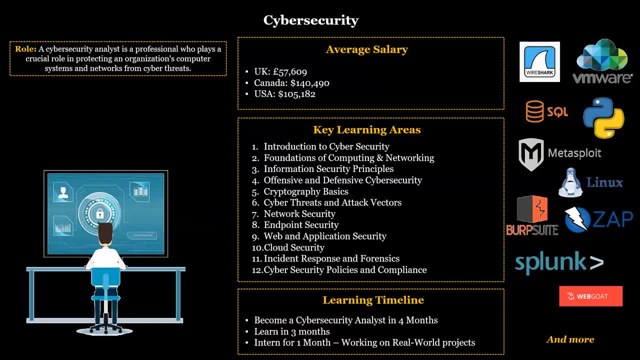 And cybersecurity is built on. So you get to understand the basic principles of cybersecurity before you now move into offensive and defensive cybersecurity Offensive in the lifestyle you want to start practicing as a penetration text expert. That means you need to be texting maybe the website that we built or application to see if they are vulnerable to attacks. 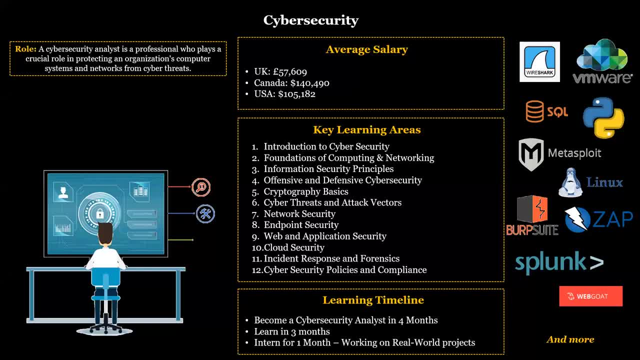 That is what. in the secular words, we call them hackers. But for you, as an information security expert, you need to understand the principles of cybersecurity before you now move into offensive and defensive cybersecurity And information security expert, because you're only. you will not be from the front of ethical hacking right. 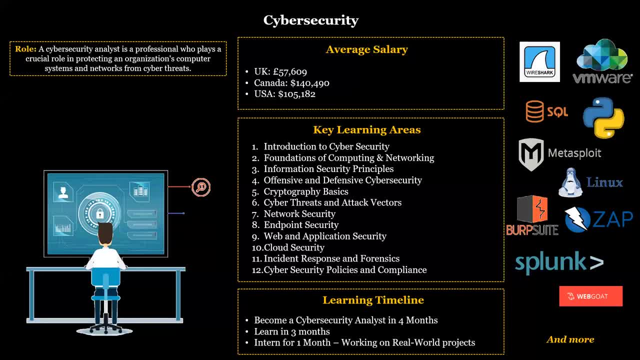 You are going to be trying to practice. if your company's website, your company's application- whether they are prone to you know being hacked, Then you also have aspects of defensive cybersecurity right Where you get to you know. build control and security models around your company so that people cannot be able to hack your company. 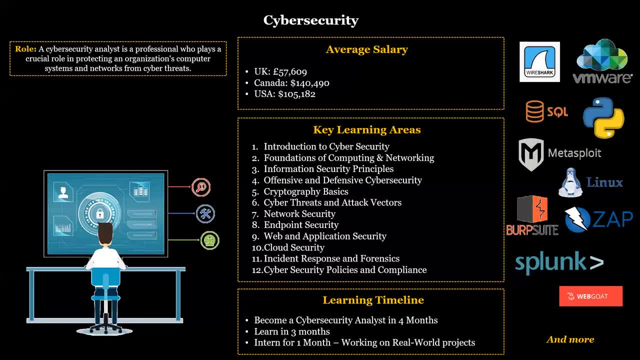 We now move you to cryptographic basics, Cyber threats and attack vectors, network security, endpoints, web application security, cloud security, incident security and forensic. and then cybersecurity policies and compliance, where you get to learn the likes of ISO 27001, NDPR or GDPR, depending on the location that you are joining us from. 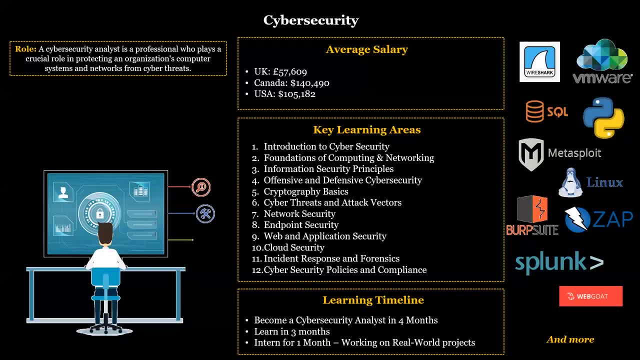 So basically what this means is that our curriculum is fully packed that will get to walk you from ground zero To the expert level, right? So if you are scared that, okay. I have zero knowledge about cybersecurity. will I be able to survive here? 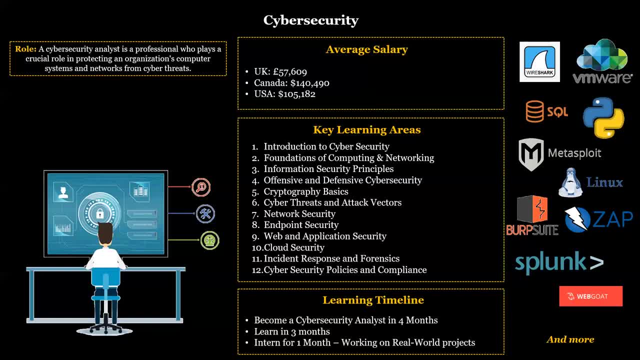 You are rest assured that you are going to climb gradually from the ground zero to the expert level And all these things. they are all practical based scenarios. right, We are going to teach you based on practical right. There is one testimony that somebody was saying, and what the lady said is that she didn't have any technical background. 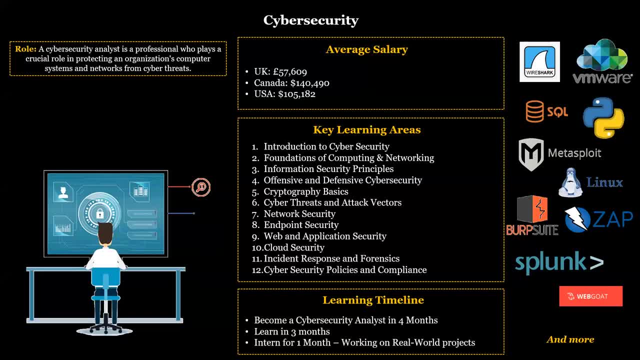 She didn't study information secrets, that analytics was the education that she needed for her to be able to transition, And that's because we've tailored our curriculum to fit industry standard right. Our learning timeline is basically four months, where you learn in three months and then you intern for one month. 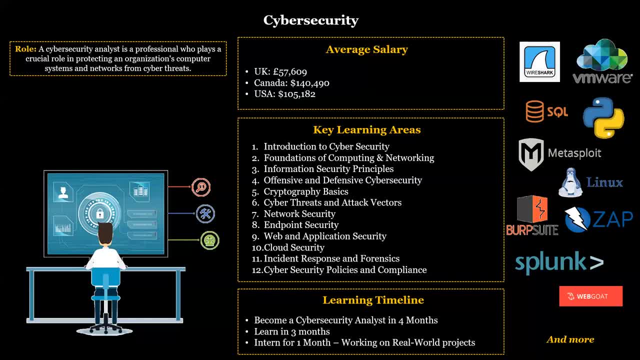 What it means is that you get to also work one month with us and work with real life Based data that we are going to give you, So you don't have anything to be worried about. You are going to be working with tools like VMware, Metasploit, Zap, Bobsuit and Wireshark. 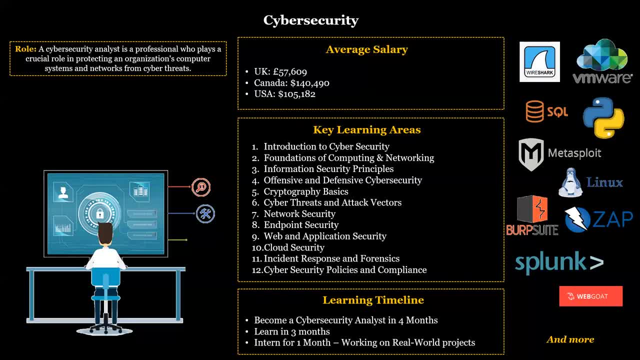 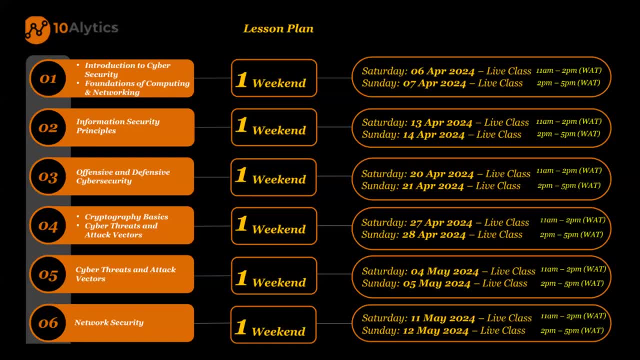 And all these things will fully packed to make sure that we give you the necessary skill and tools for you to succeed. So, if you can still see my screen, basically this is just like a roadmap: the journey to what you will be having you will be doing in a class. 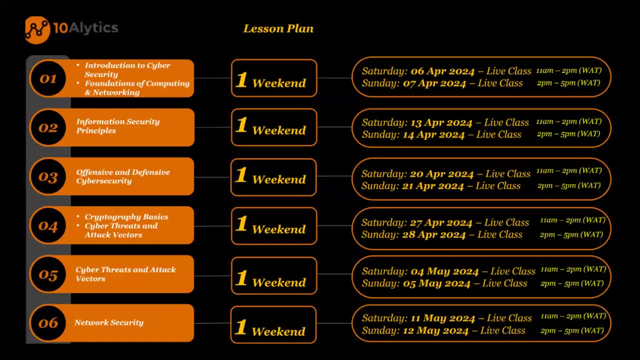 First we do, We will be doing- cyber security, like I mentioned, foundations of computing and networking. Second week, you walk into information security principles and so on and so forth. So this is just like the what the people in class currently are doing. 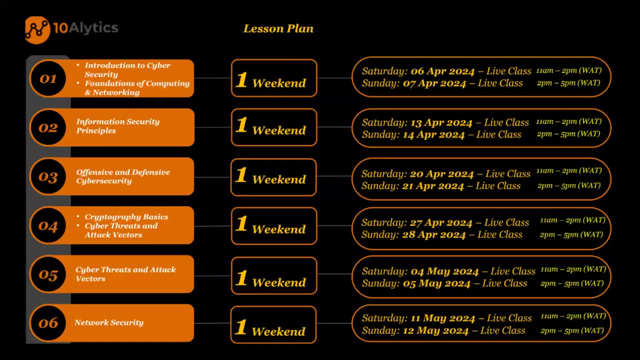 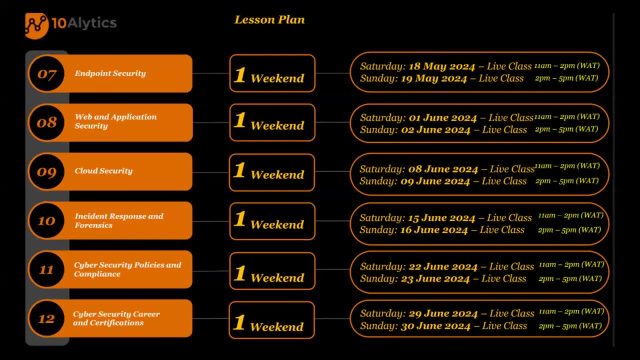 People that joined in April. this is their own lesson plan, And that's how we've also designed the lesson plan for a 13 weeks program for you. So what are you still waiting for? Why should you Exactly Train with us, right? 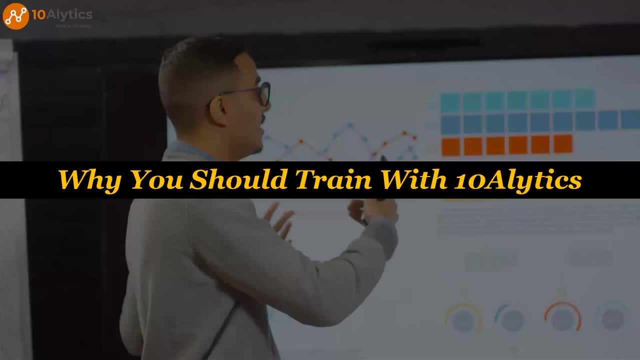 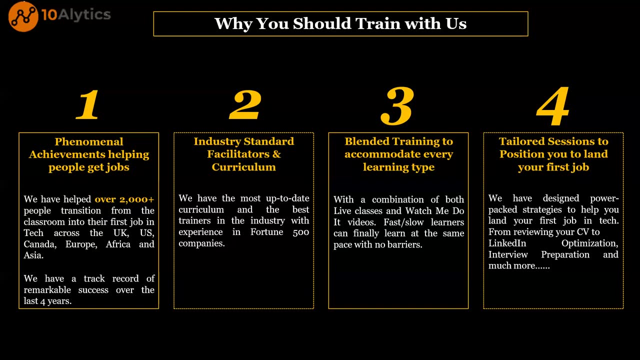 Why should you train with us Basically? over the couple of years, we've had achievements that transcends and it's echoes in industry. right, We have phenomenal achievements that we've helped over 2000 people from classroom into their first job across the globe right. 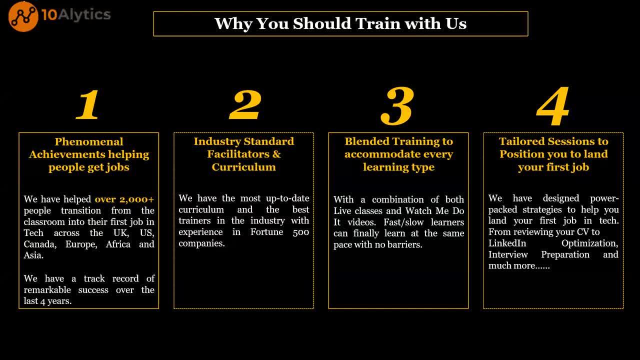 This is in UK, in US, Canada, Europe, Africa, of course, and Asia. This is a track record of minted Over the past four years that we have been operating And, like I also mentioned, we have industry standard facilitators that come from diverse places. 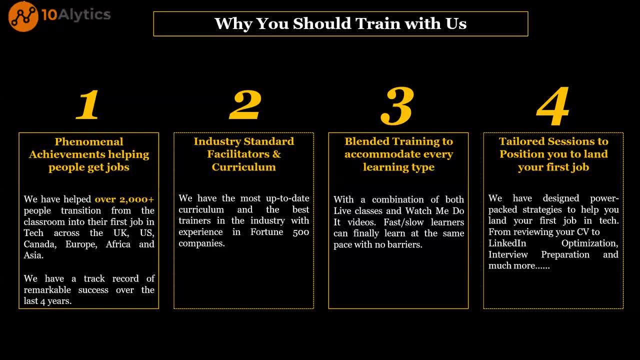 You have people coming from people like Joshua coming from assets bank, people coming from from Deloitte, from coming from KPMG, who are coming from interest, which people coming from all manners of, like all the basic companies that you know right. 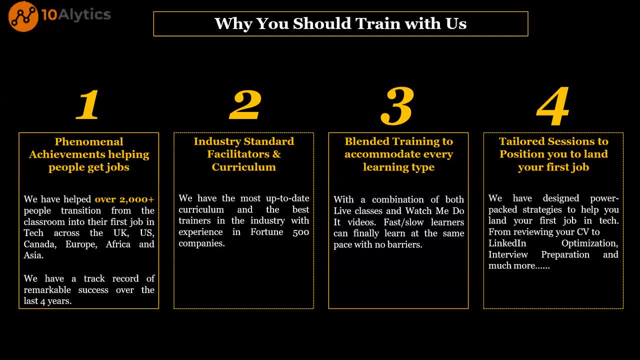 People that offer core value, And these are who that also design our curriculum to fit into What is obtainable out there in the real world, which means you don't have anything to worry about with that You will be reading books. No, they are all based on real life case studies of what these people experience in their own roles. 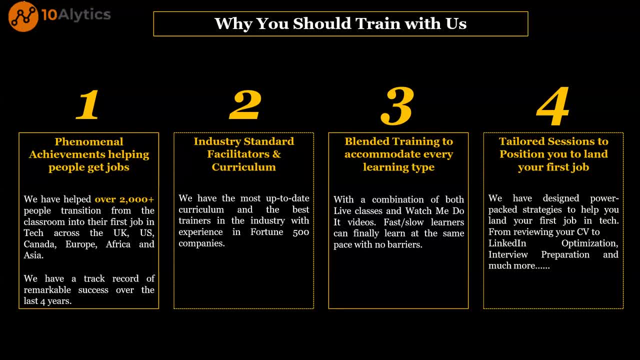 Right, And we have a blended training model that accommodates your learning type. What do I mean by this? Our learning model is structured in a way that it is a life class. The way you are interacting with us right now, That is the way you are going to interact with your facilitator on your classes, right? 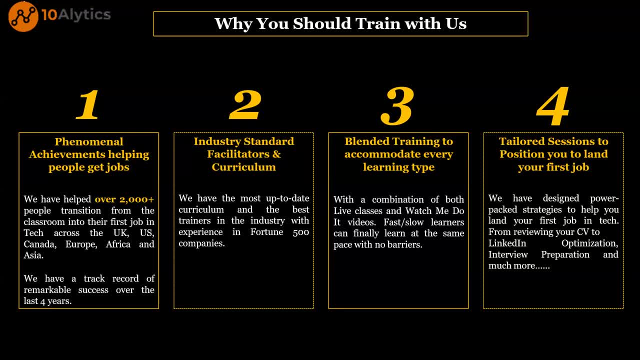 You are going to be interacting with them one-on-one, And then these classes are also recorded- that, even if you miss any session, you have lifetime access to the Google Classroom, And what it means is that you have the course to always go back to the Google Classroom to watch the video. 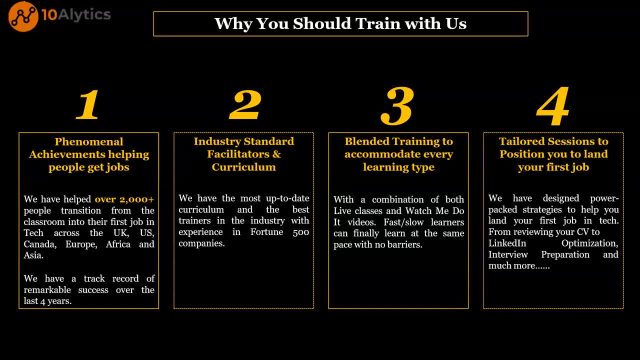 The way this session is recorded and is going to be sent to you after the classes. That's how our normal classes are also recorded: That even if you have any core reason why you miss classes, you get to have the video to watch so that you can also come up to speed and prep for next class. 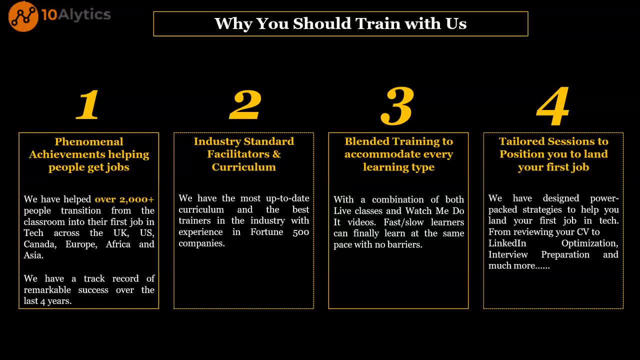 Right. We also have tailored sessions to tailor you for your first job Right. We've designed power pack strategies to help you to land your first job, which I'm going to talk more in our employability services. This is not all Right. 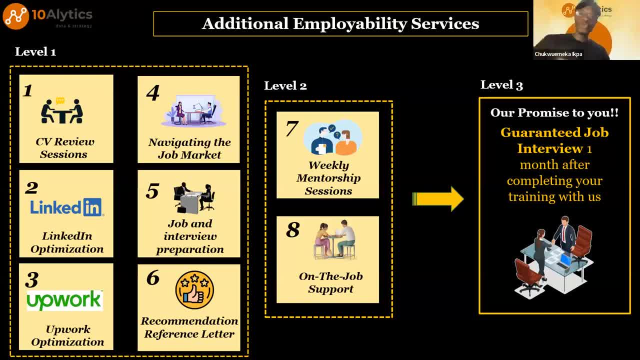 We also have other things that we've provided for you. So, under three basic approach to ensure that you get the job that is out there, Right? We have the level one, which is basically the CV review sessions, Right? So these are sessions where we get to look at your CV and make sure that it's tailored to the job that you are applying. 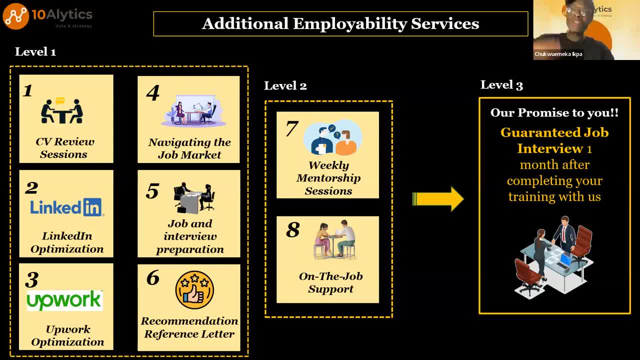 Right. So we have CV review sessions to teach you how do I apply to jobs Right, And the truth is that people have trivialized job application These days. that and that's part of the reason why we are not getting jobs, because we've made it like um, it's just a game- boots LinkedIn. click on easy apply- easy apply- easy apply. 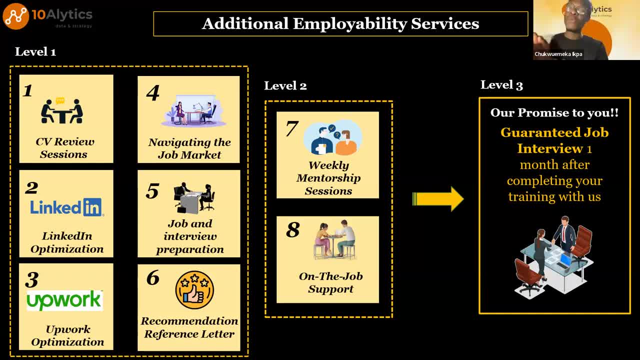 No, if we continue to do it that way, we are doing something wrong. We have to tell our CV to fit the job that we are applying for. For example, you have cyber cybersecurity skills and you- um, you have SQL knowledge and maybe the job application is saying that, okay, we need someone that has. 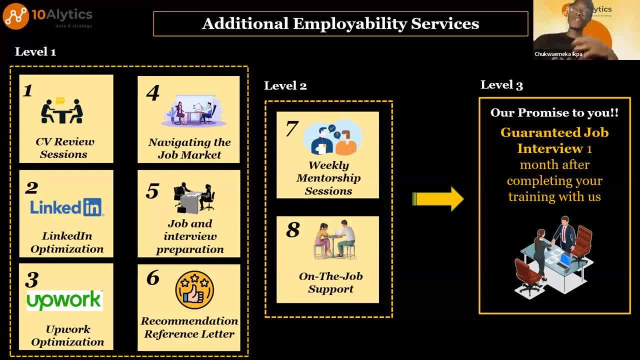 Yeah, You have post-grad knowledge and in your own CV you wrote: you wrote SQL, right? You've not tailored your CV to fit what they are looking for, even though it is the same tool, but the communication is different. 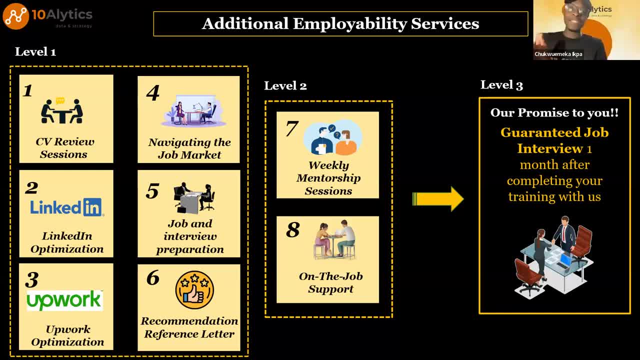 And once it is passed through the applicant's tracking system, HCS, is going to come out as failed because you do not have post-grad skills. So what we tend to do is also teach people: how do I tailor my CV to match all the jobs I am applying for? 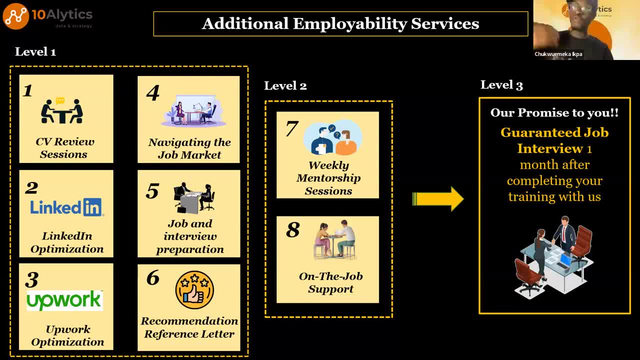 It is not. It is not an easy task, but it is something that is necessary for you to be able to get there. Remember, your CV, just like a walking signboard of you, is going to get there first, before you can now come physically to represent yourself. 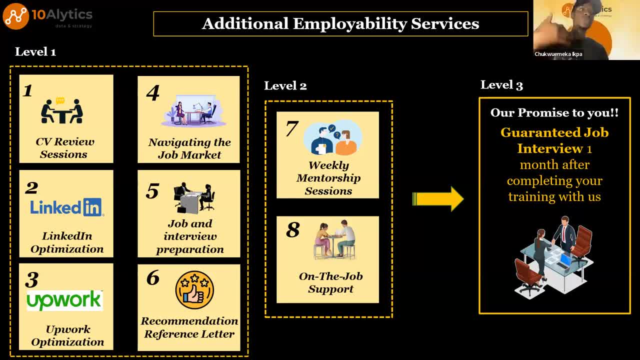 Number two, we have LinkedIn optimization sessions where we get to teach you How do I optimize my LinkedIn. The last session that we organized, I think a friend of mine that is in one of the sessions immediately after the session and she applied everything that she learned. 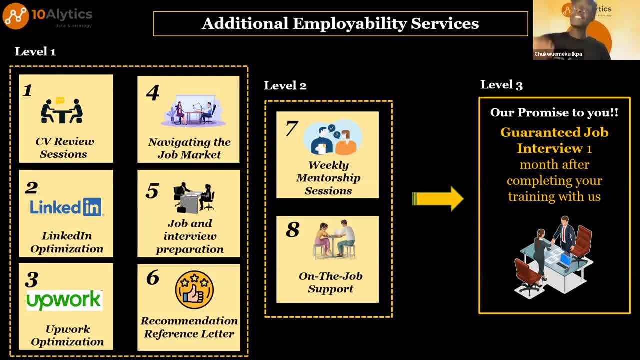 A recruiter reached After her position. she's in the UK and she got the role right, But she wasn't able to take it because she's still in class and she can't work above 20 hours because of the limitations in the UK. 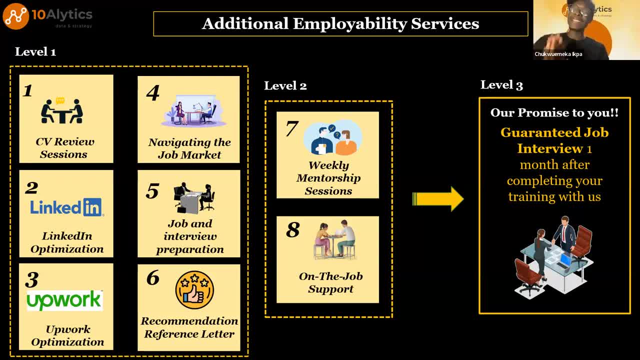 So these are things that we get to put you through aside the normal skill and competence training that we are going to give to you. Number three is the Upwork optimization. These days is the era of freelance right. It can be in Nigeria and you're working for a company in the US. you're working for a company in Canada. 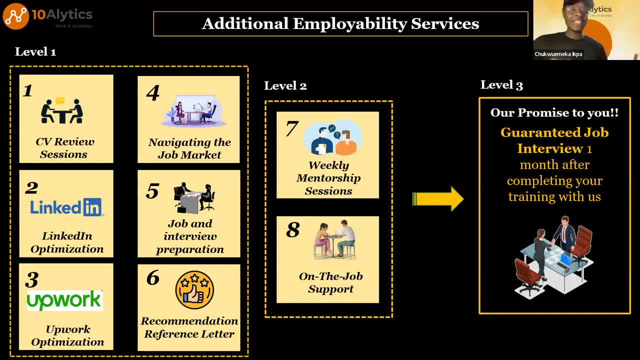 Just as we all are here, some people in reality, some are in Canada, some are in UK, some are in Nigeria, some are in Rwanda. we are across the entire globe, right, And this is the beauty of what Upwork can do for you. 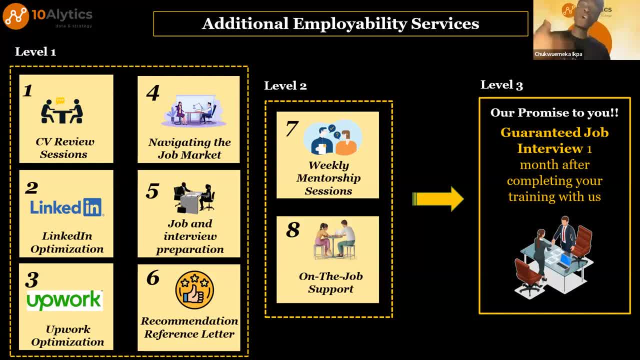 So we have sessions to also teach you how you can leverage Upwork to serve as contractor in all this area and get remote roles. We also teach you how do you navigate the job market right. How do you navigate the job market? We have job. 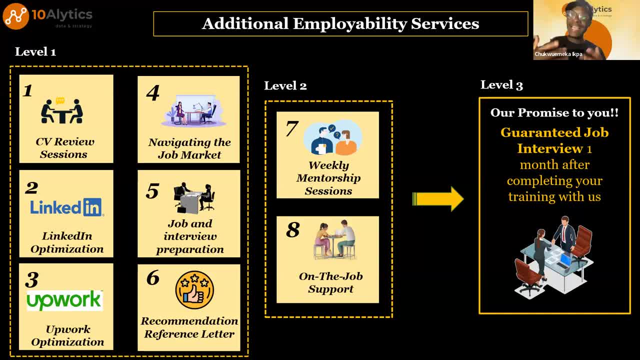 We have job and interview prep sessions where, if you get an interview invite you get to book a session with us and we teach you. we have a prep session with you to teach you and let you know things that you are going to expect in that interview, right? 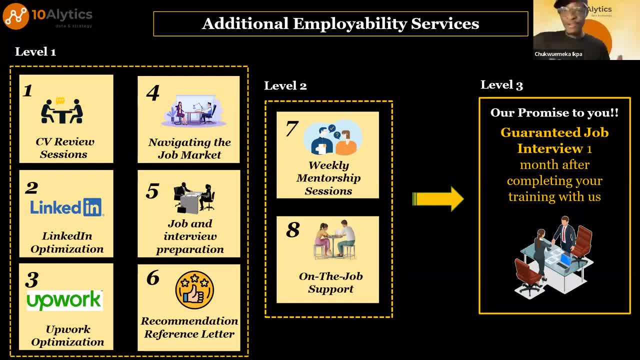 How do you even answer the question of tell me about yourself? Are you using the SIT framework to basically show and present yourself based on situation achievement? Are you using the SIT framework to basically show and present yourself based on situation achievement? 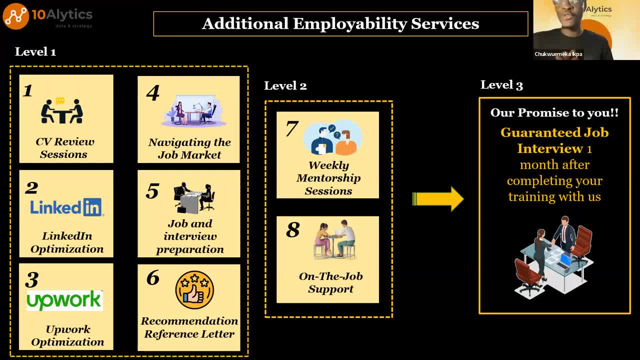 And the type of person that you are? or if they ask you who are you, Are you just going to say: oh, my name is Chukwe Meka, I have 12 kids. I'm married to 10 wives. No recruiter wants to hear that. 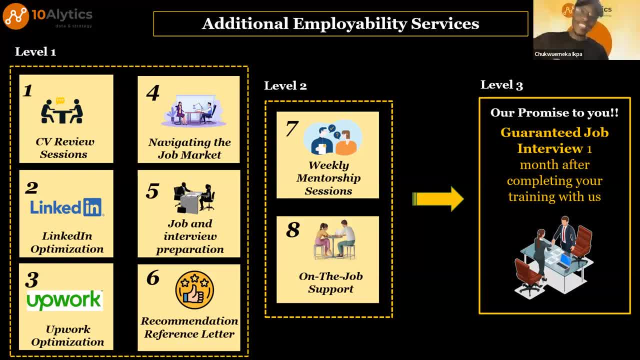 So they want to hear who you are, based on the SIT framework right. And then we also provide recommendation and reference letters if, in the future, somewhere you want to apply to, or maybe the embassy, or any of the tech career. you know these days the era of people trying to do the job right. 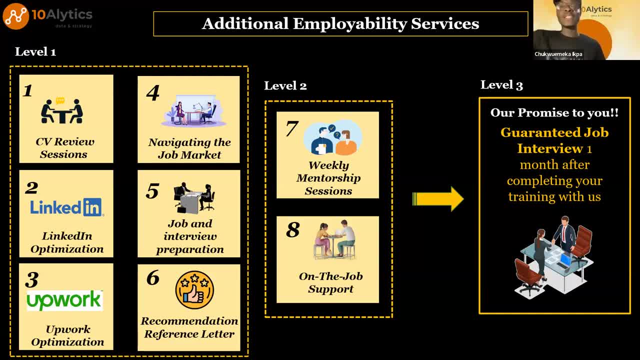 So you know if you have a position you want to get a job, right country if any of them requires it, we also present recommendation and reference letters. number two level is our weekly mentorship sessions. right, so we have mentorship sessions where we get to bring. 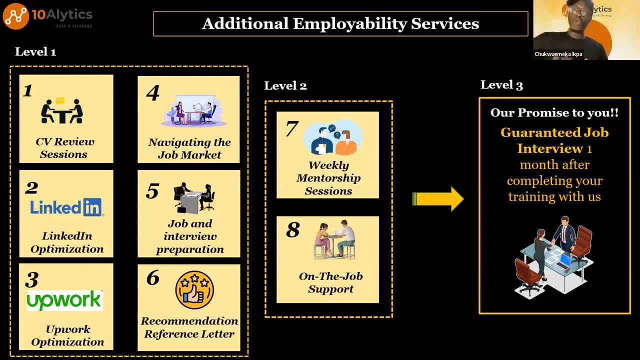 people into the class to actually talk to you based on your own field. for example, if you are in the cyber security class, you'll be getting facilitators from cyber security field come into class to tell you, okay, which area of cyber security is even better for you to specialize in. 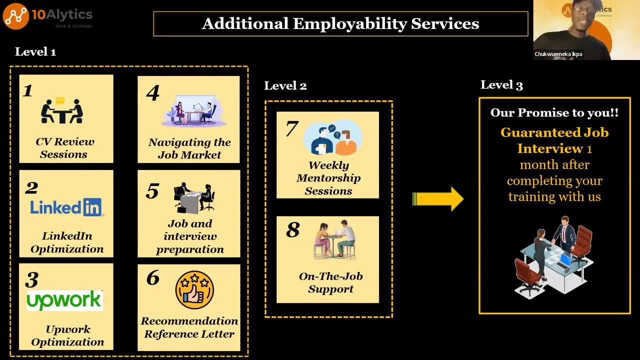 is in network security, is in application security, is it in um website security, is it in grc. that's governance, risk and control. compliance is in the aspect of incidence report. so these things are things that our weekly mentorship session also offers, and we also bring in people that have 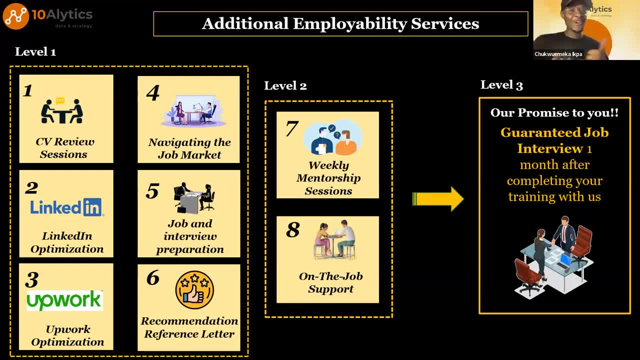 worked the work right, people that have people that have worked the work- that's a nice acronym, you right, we get to bring in people that work the work right to tell you: okay, they were in class before you. this is what i did, this is what i did not do and this is what helped me to land jobs. 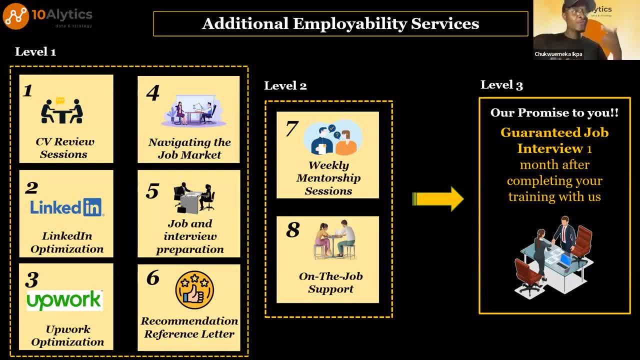 and also provide on the job support. so if you get jobs- and you are still now, you know- if you get jobs and you are struggling to, um, you know, stand firm on that exact rule, we also get to give you one more support until you can cost, and easily. 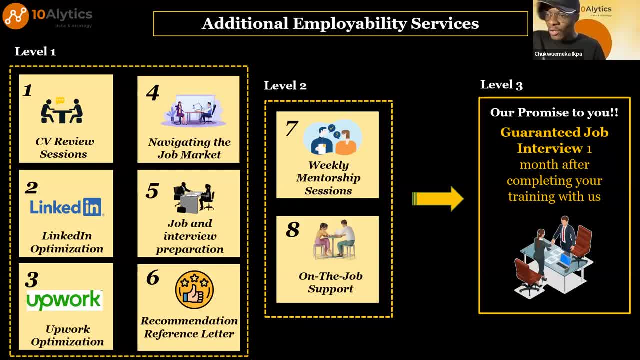 stand, i think i'm getting a question from evie. true, i'm so confused on the part of cyber critical focus on fantastic evie. so these are things that we also offer on the mentorship sessions right, where we bring in experts to also talk you through the various aspects of these. 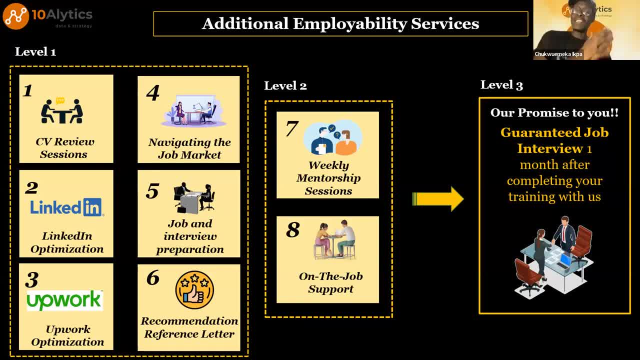 things that exist out there and how you can easily specialize. so number three aspect of it is our promise to you, right, if you confidently and comfortably do these things, that we are going to provide for you attend classes, and if you are not going to provide for you attend classes and 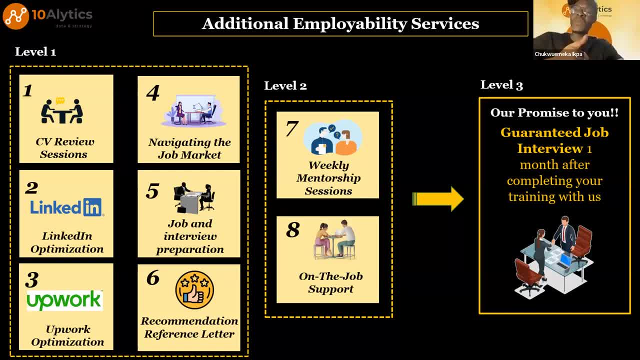 attend CV review sessions, attend mentorship sessions. We guarantee you one job interview one month after you are done training with us right, And we can comfortably say these things because of what we offer and because of the people that have partnered with us. 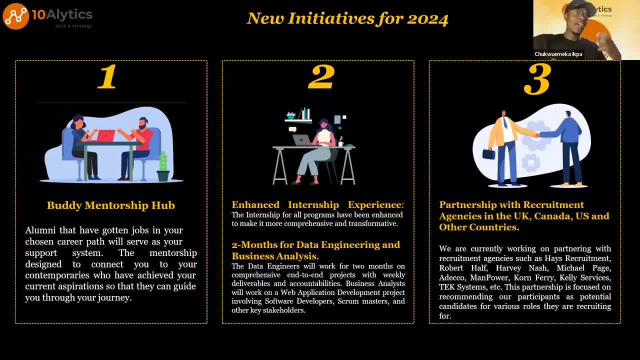 So we have the likes of Robert Half, Harvey Nash and Adeco that have partnered with us for us to be able to provide them with some of our students right. What it means is that after you are done with us, you are also placed in a pool, right. 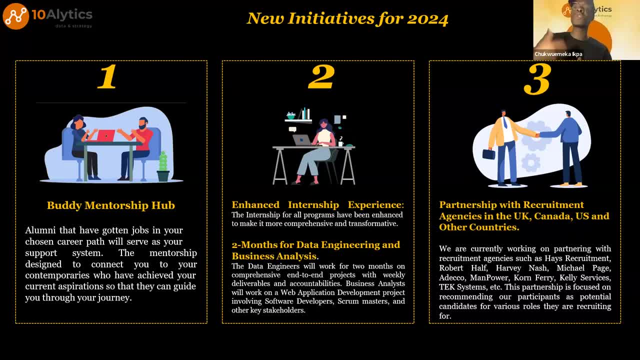 And once these recruiters come to us and say, okay, it's analytics, we need two cybersecurity experts. Can you guys provide these guys for us? We are good to provide people that have comfortably completed this program, comfortably done everything that we needed them to do. 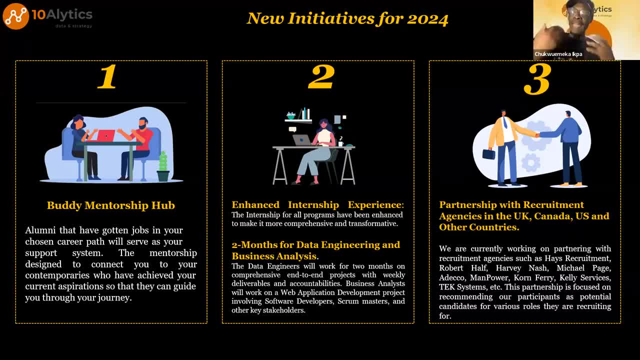 to our partners so that they can be interviewed and they can also get job placements. And number two thing that we also offer this 2024 is our body mentorship call. Like I mentioned before, now we have people that have worked their work. 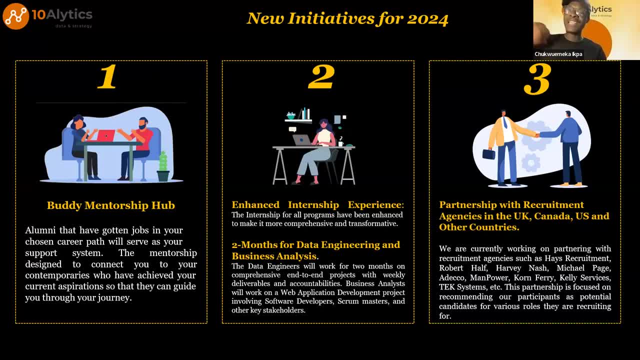 We bring them back to class. that's the alumni that have done that, have passed through what they are currently passing through, so that they get to also serve as body mentors to you. They get to explain to you. okay, I faced this challenge during my own time. 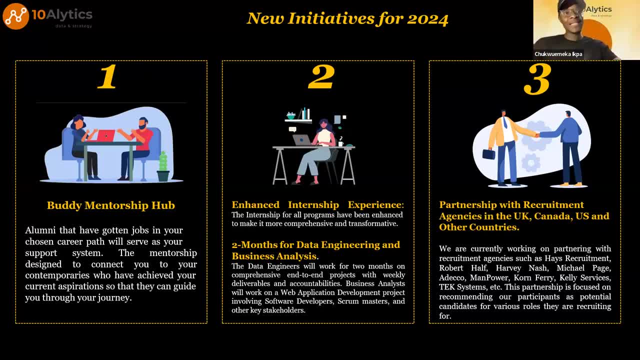 This is how I navigated it right. Once we get to this right, This exact end point, you are going to see this problem. take your right or take your left, You know. the truth is that most of us, we struggled in this tech ecosystem. 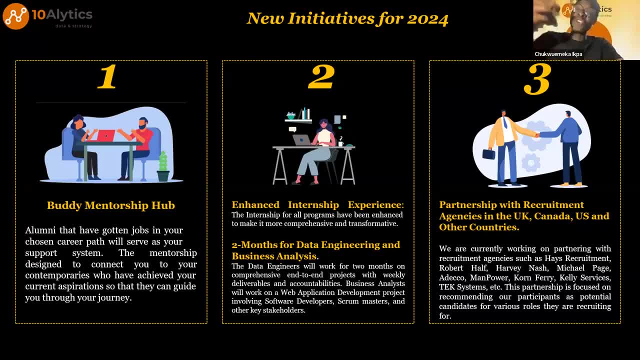 because we never had mentors right. So if you do self transition or self-study, most times you get to study everything that exists out there. You don't really get to see the exact pivoted points to transition through, And that's what our body mentors are there for. 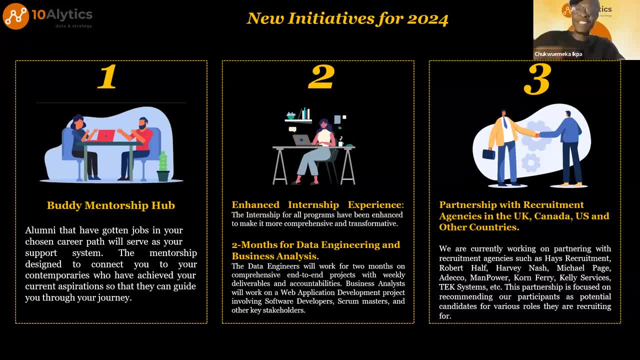 So of course we are struggling for two years doing courses just trying to get into tech ecosystem, And that's what our body mentors are there for. So of course we are struggling for two years doing courses just trying to get into tech ecosystem. 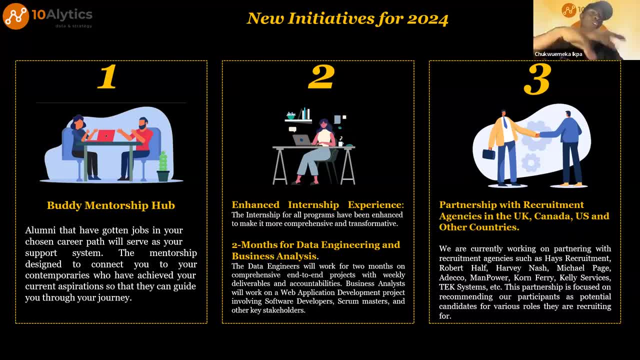 And that's what our body mentors are there for. So of course, we are struggling for two years doing courses, just trying to get into tech ecosystem, But Hadibi will have someone that held our hand to say: okay, Chukwu Emeka, learn Power BI. 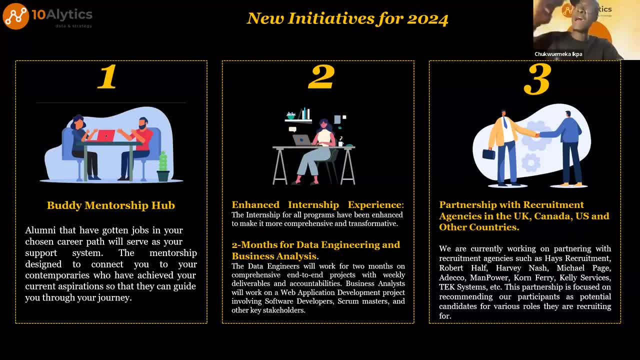 learn SQL, learn Python, transition to tech. We won't go ahead to be learning MongoDB, learning Looker, Anyone that comes out. we are jumping to learn. but then is it what the company, is it what they are practicing with on daily basics? 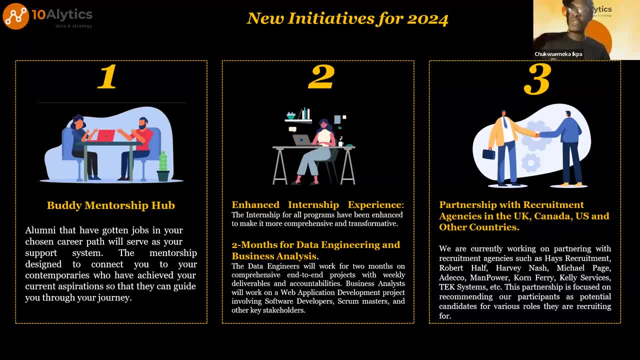 So these are things that body mentors come back to the class to give us to understand And, like I mentioned, we also have enhanced internship experience where, once you are done training with us, you get to join our internship program, where you are, first of all, reminded- 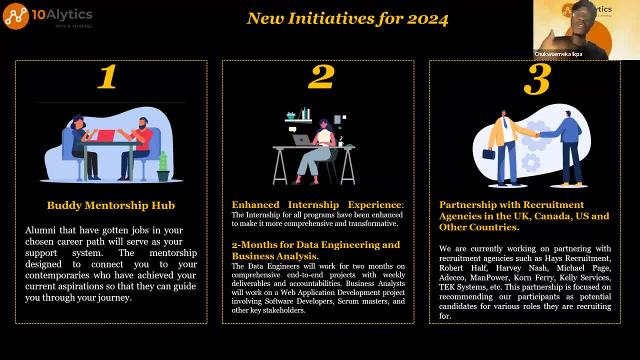 how to position your portfolio. So if your portfolio is not yet built while you are in class, the internship program is going to help you. first of all, make sure that you set up your portfolio And then you start also working on projects that you can place in your portfolio. 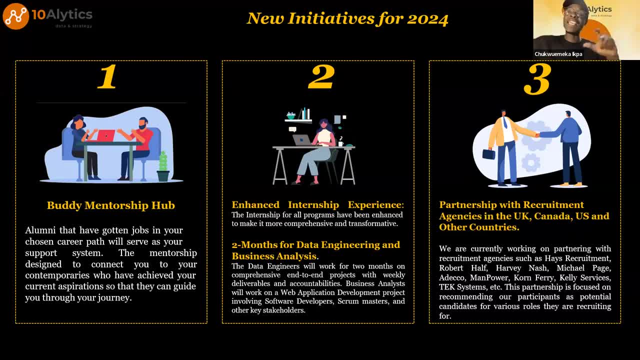 Let's remember: there is no tech employment, tech interview that you can do in your portfolio, So there are no technical skills that you can go for that. they're not going to have a competence assessment. They are going to test you based on your skill. 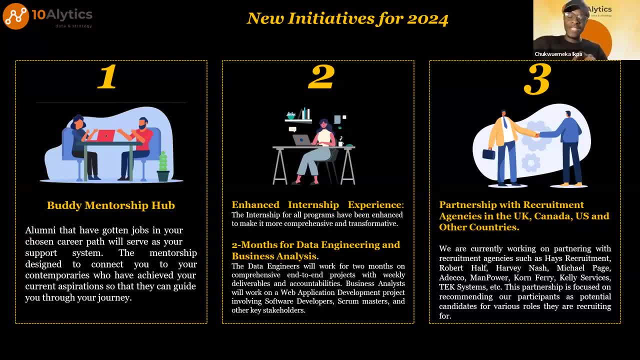 And this is one of the problem that we face while applying to jobs. We place the cart before the horse. And what does this mean? We try to get certifications before learning the skill. Maybe someone do not have any technical skill relating to cyber security. 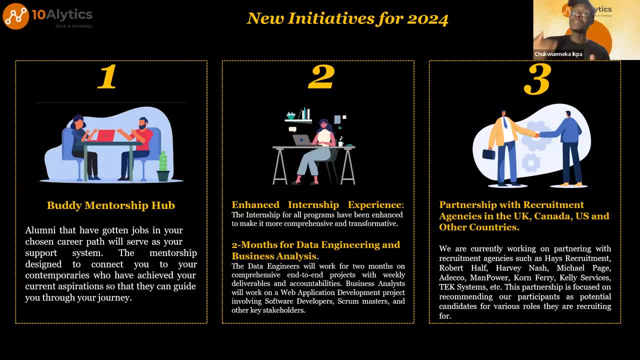 and you see the person studying to get CSAB, But this person don't understand what, what the plan is right. This is someone placing the cart before the horse. So you need to first of all get the skill and the competency. 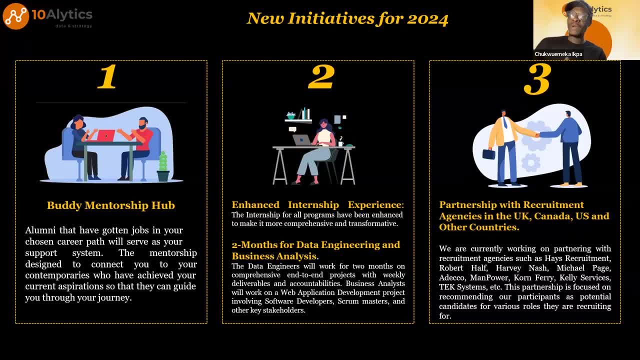 get the hands on and then get a job, And then, you know, start continuous learning where you now get to start getting all those various certification. So our internship program is going to position you for it to be able to hone your skills, for you to be able to have enough portfolios that you are. 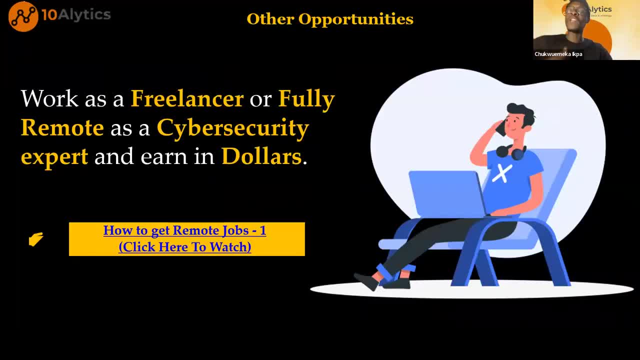 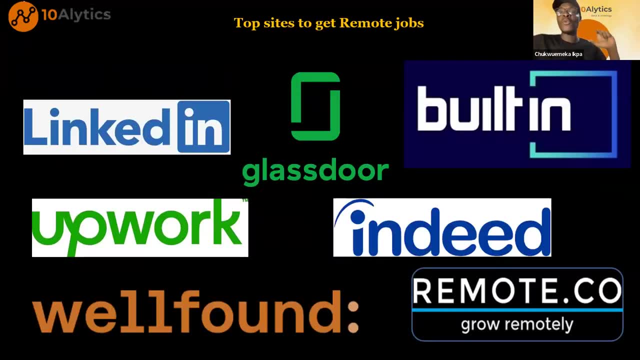 going to present to recruit us, So that any point they want to look at what you've done in the past, you can comfortably present all the projects you've worked on while in class and while in the internship program so that you can easily prove to them that you have. 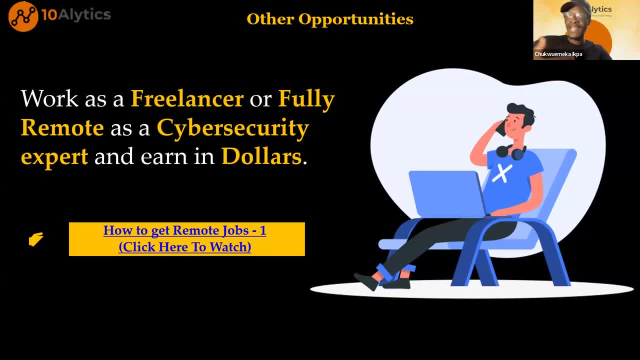 the experience that they are looking for. Now we also have, like I mentioned, the freelance aspect, where you get to work as a remote person. So, once you get this slide, don't forget to please fill the attendance form So that, once we finish this call, 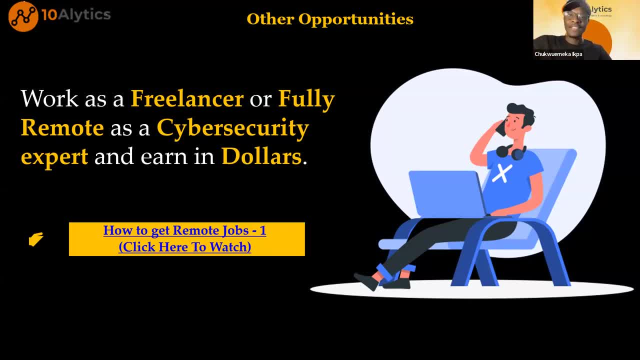 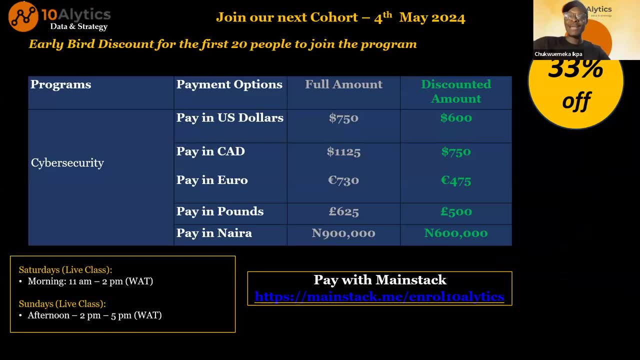 you are going to get the recording of this session and also this slide, Okay. So all these things that I've been saying, how can you get into it? Remember I mentioned that there is level four things that we're going to do today. 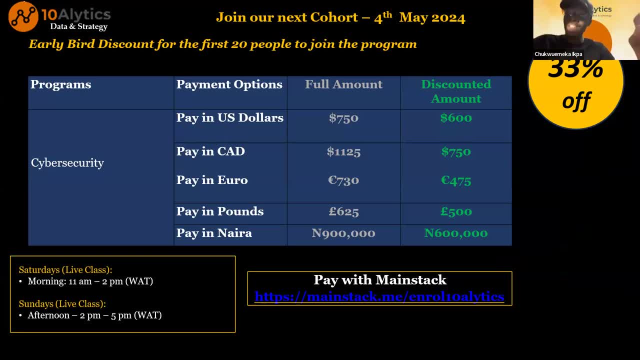 And we are in the fourth part, which is basically what is my offer to you. So at the moment, we are giving you a 33% discount right, And this is an early bird discount for the first 20 people to join the program right. 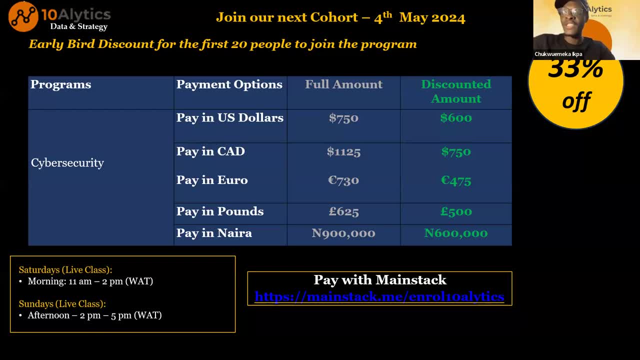 So naturally the cost goes for $750, or 1,125 Canadian dollars, several and 30 Euro, 625 pounds and 900,000 Naira. But because you've been on this call till now, we have a 33% discount for the first 20 people. 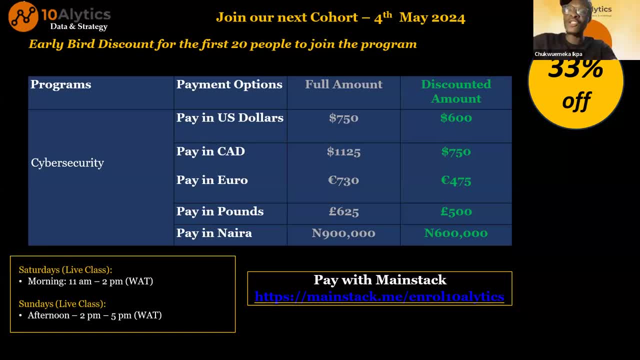 that is going to register. That means you are getting to pay $600, 750 Canadian dollars, 475 Euro, 500 pounds or 600,000 Naira. What I always advise people to do is to take advantage of this to get into the tech ecosystem. 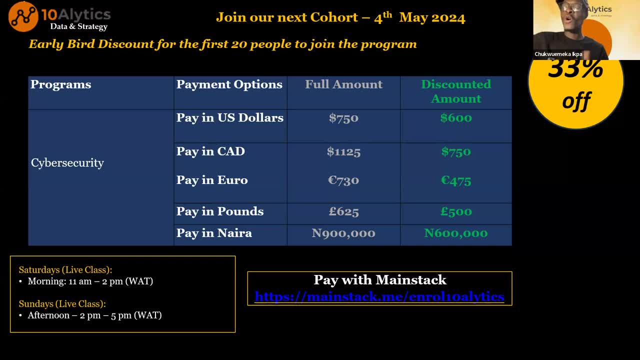 Let me tell you a story. Last month we offered what we called International Women's Day Discounts, And that was a 50% discount. Some people didn't register. They said, Oh, I don't have money, I want to register in April. 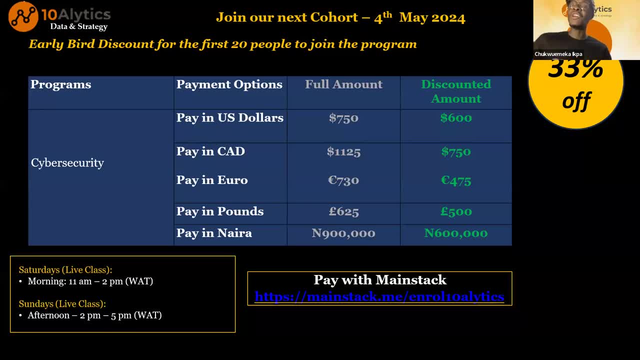 Now, coming into April, that discount is entirely off. It is now just a 33% off right, And that is why I'm telling you to take this opportunity to get into the tech ecosystem. How do you make payments? So it's very simple. 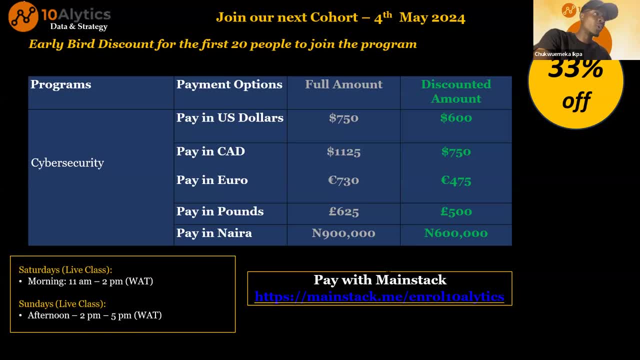 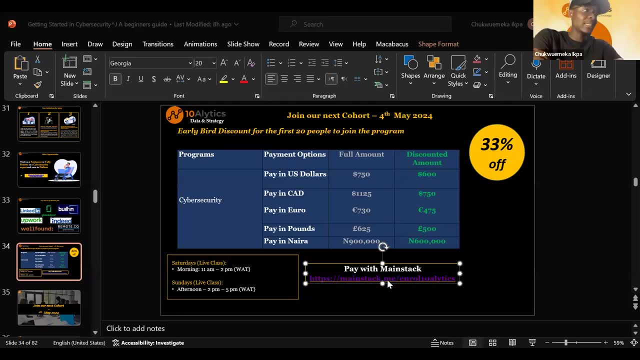 My colleague is going to drop the link in the chat box. Once you click on the mainstack link, that is provided. once you click on the mainstack link, that is provided provided. i'm trying to share my screen so that we also get to see how we can navigate this exact. 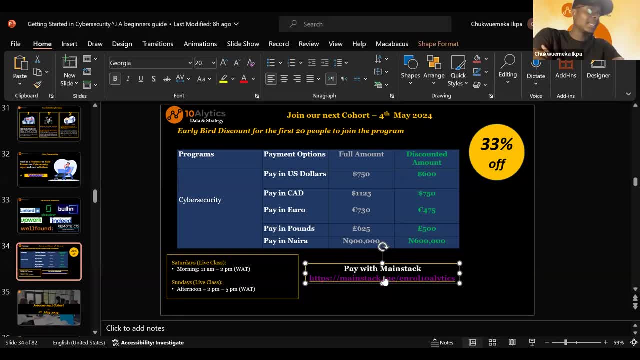 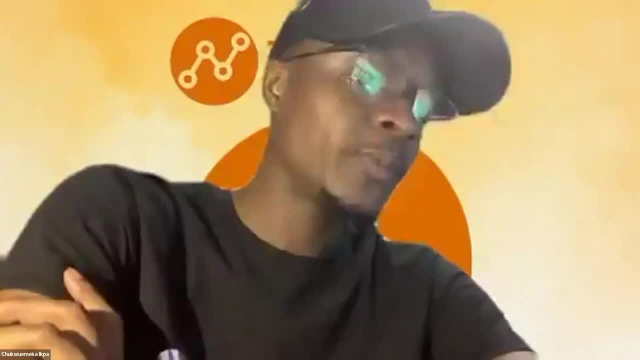 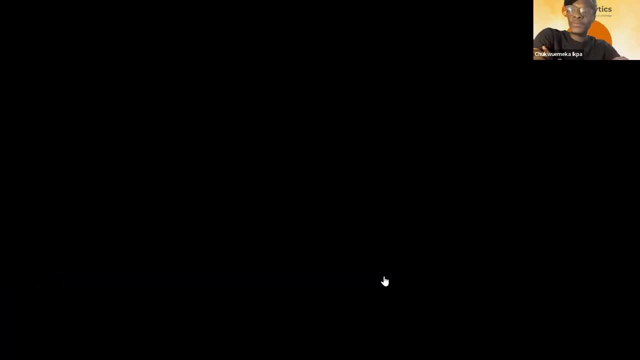 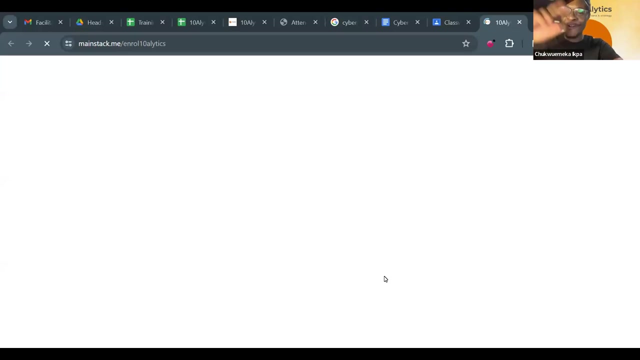 area. so once you click on the link that is provided, you are going to be all right. my screen is coming up. okay, it's coming up. i hope we are still following. please, if you're still with me up to this moment, just drop a yeah, yeah or anything in the chat box so that i will know that. 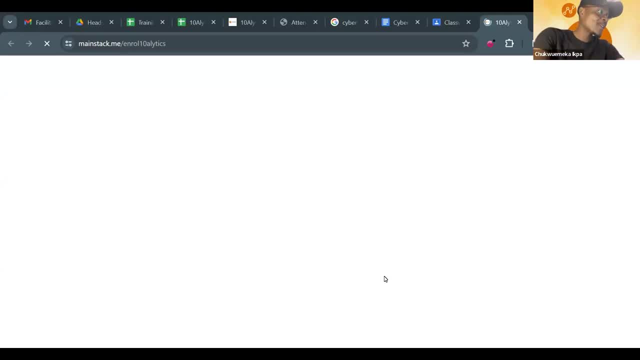 you people are still with me till this time. okay, if you are still with me, please drop a yeah, okay, confirm, elvis, confirm, uh, how do you pronounce this? 3w 2009? oh, fantastic. i think it's the name of the phone also amazing. so once you click on the link, it's going to bring you to this exact. 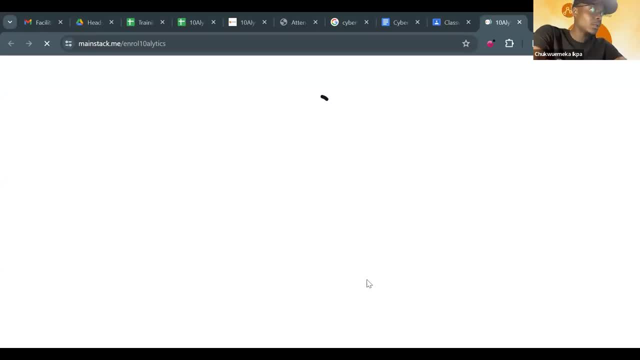 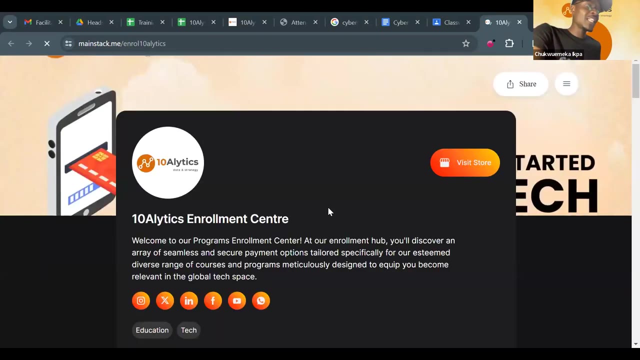 payment option. i think my network is slow still coming up. it's just a minute, just a minute. you can also try it with me so that, once i'm showing you how to do it, you can be trying it from your own side and be making payments um easily. so is. 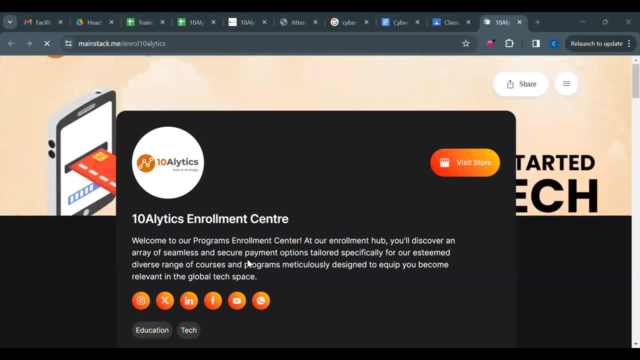 someone speaking. okay, so it's good. sorry, someone is interfering. um, adam, please do you mind um blocking iphone? okay, i've muted iphone, all right, so going on, it's going to bring you to this enrollment center, right? so what you're going to do is just scroll down, scroll down. 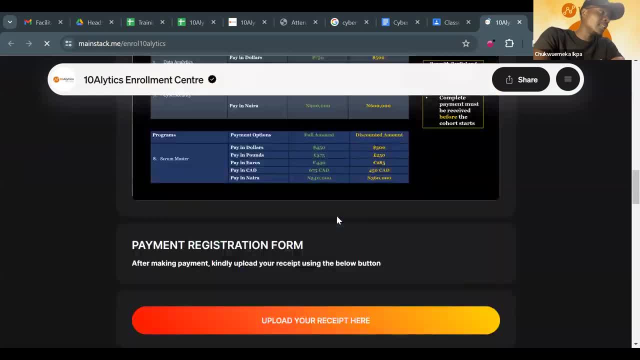 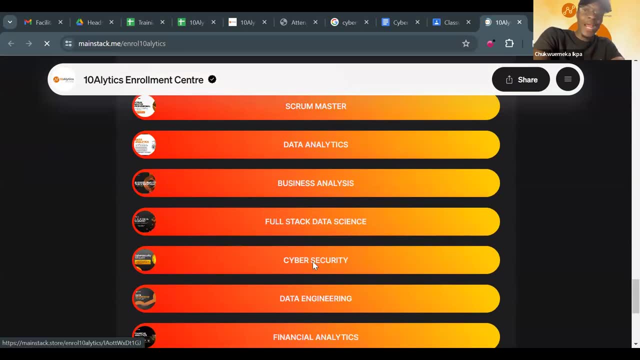 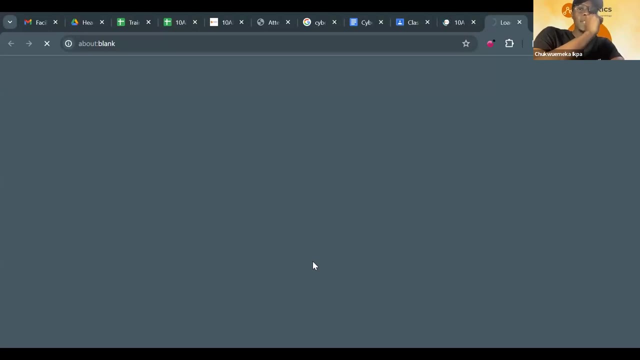 scroll down and just look for the um cyber security. right, look for cyber security. once you get that cyber security, you click on it and then it is going to bring you up to where you can make payments. so, depending on the country that you are joining us from, is going to bring up the currency of that region. so if you're joining, 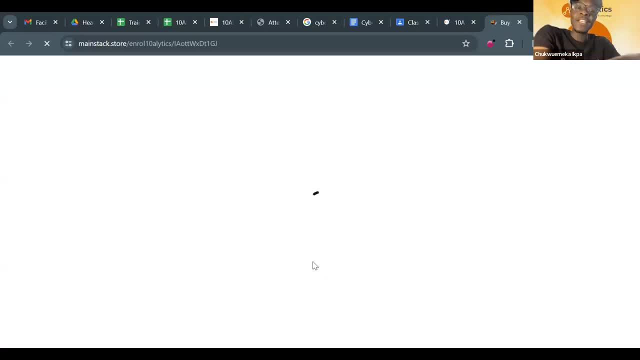 us from nigeria and trying to make payments. you are definitely going to get the naira option to make payments right. if you are joining us from uk, you are going to get the pounds option. if you're joining us from the us, you are going to get the kind of card um. you are going to get the card um. 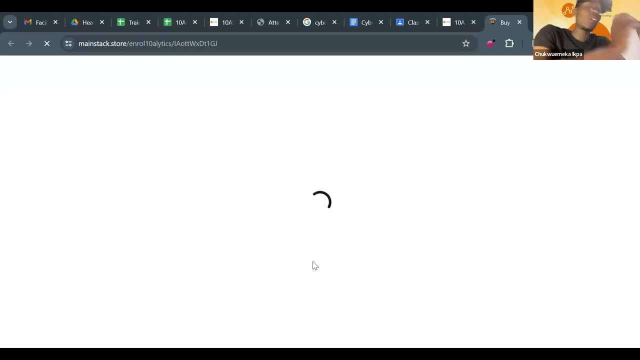 dollar option. if you are joining us from canada, you are going to get the canadian option. so, depending on your location, is going to automatically pick the currency of that location and ask you to use that currency. okay, i think i'm someone is asking instrumental plan. all right, um. 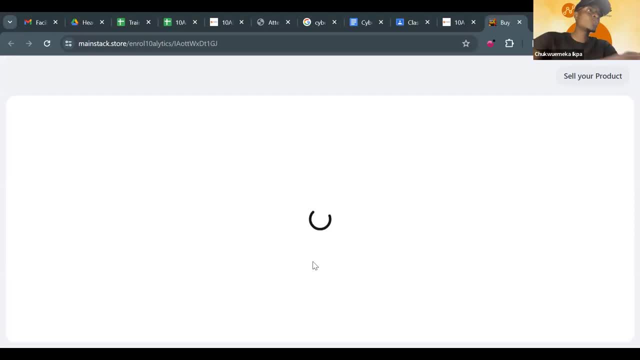 i'll still get to there. yeah, but there's also an instrumental plan. you can decide to make the first payment to reserve your spot, but the expectation is that before you get um, before default of me- at the classes starts, you will make the complete payments, right, so, um ariremo, what it means is 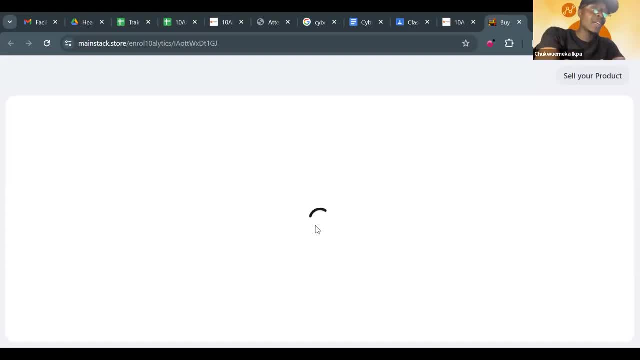 that you can decide to make 450 000 naira now to reserve your spot, but before default of me, you are expected to make the remaining 150 000 naira to complete your payment. right? what if i'm joining from uk with an english vpn on elvis? every smile alright, amazing, amazing. 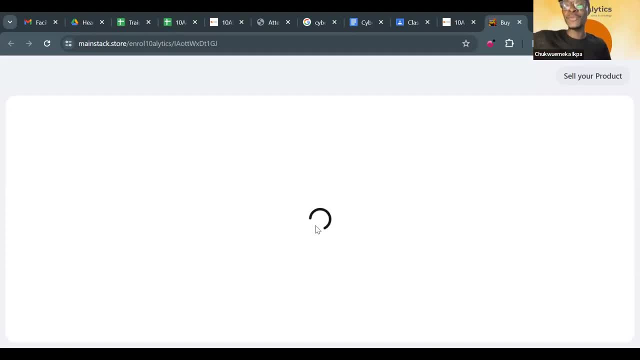 So definitely, we all know how VPN works. It's automatically going to pick your IP as if you're in Nigeria, So it means that you know your way around what you're talking about, So we won't get into that. 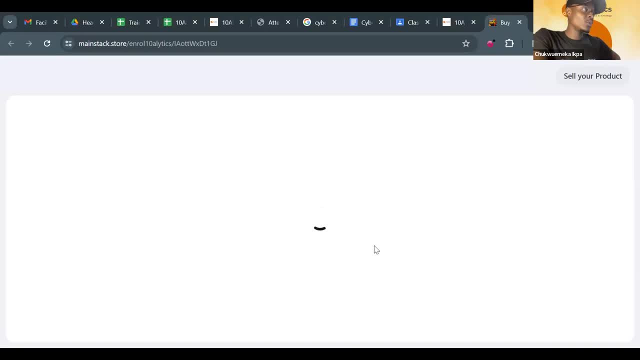 But once it comes up, I don't know why my network is so so slow. It's so so slow. Once it comes up, you automatically just click on the option to put in your details. Let me try and change my internet. 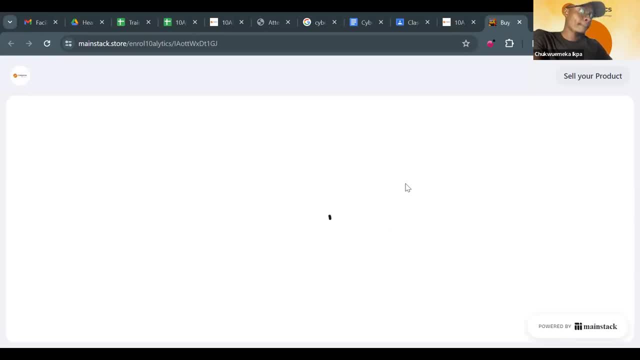 Please, one second. One second please. Okay, like I always tell people, try and take advantage of sessions like this. Remember, we said that it is only for the first 20 people to join these classes. right, And as we are speaking, people are already taking advantage of this exact first 20.. 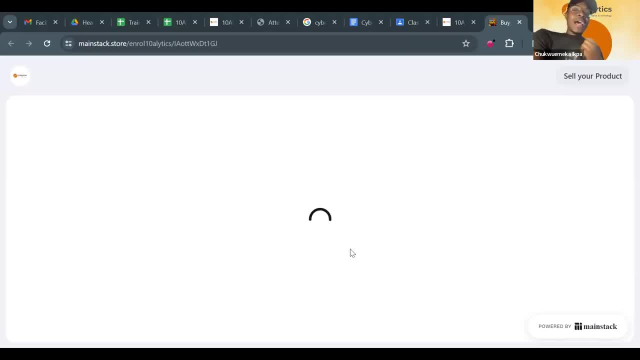 So try and take advantage of it also And be able to get into the class with others. Okay, So once you've clicked on that option of cybersecurity, it's going to bring you to this spot. Okay, I think this is taking a while to start. 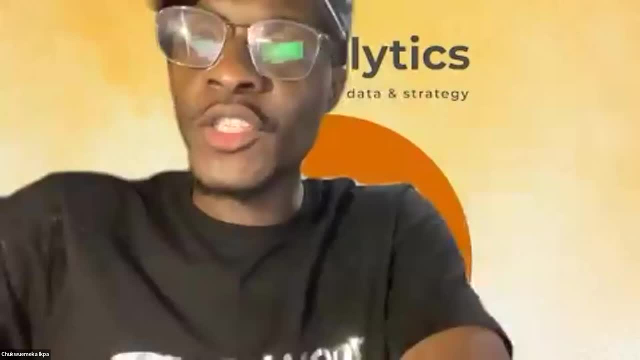 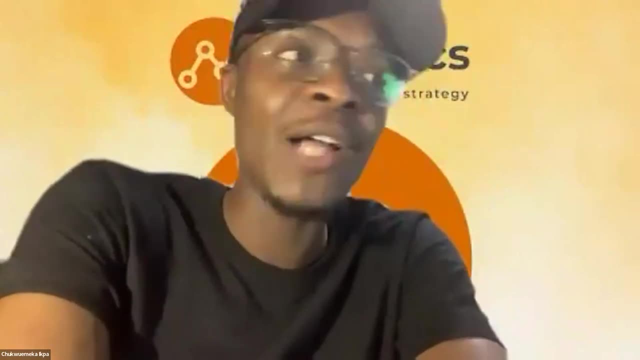 So I'm going to continue. So, generally, at that spot, you're just going to put the amount you are meant to pay, right, Okay, Okay, Okay, Okay. You are going to put the expected amount you are meant to pay. 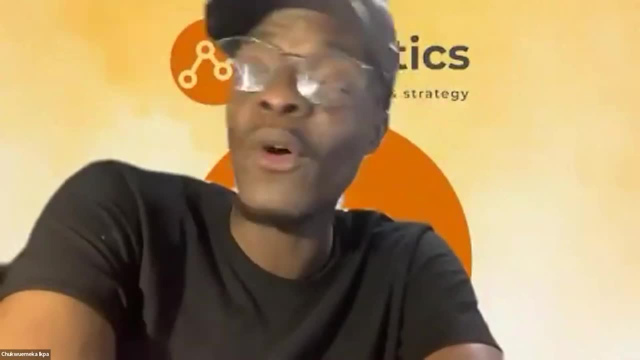 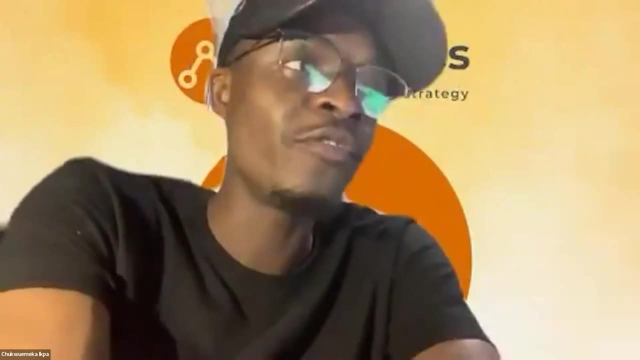 Remember I said you can pay the minimum deposit there, which is 150,000 Naira or so, depending on the currency you are making payments with, And then, before the 4th of May, you are also expected to make the complete payment. 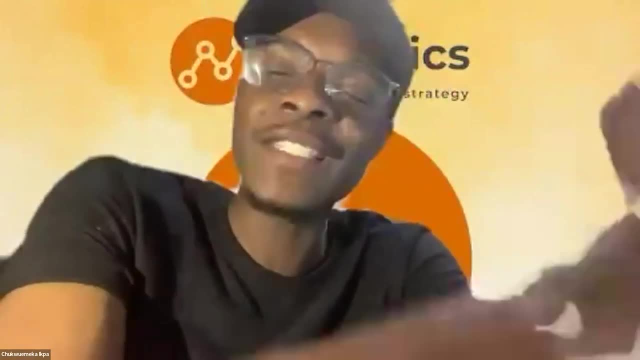 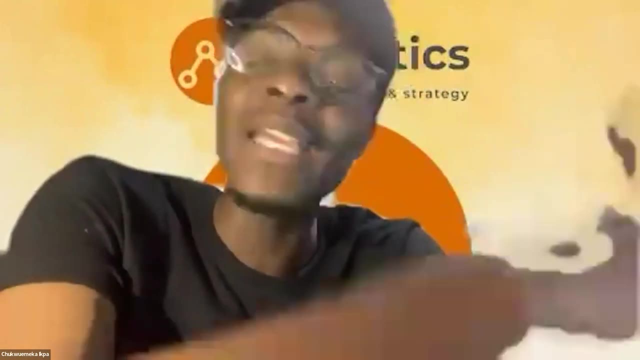 Before the class is over, I'm going to play a couple of videos for us to see what the past students have to say, For us to be able to know. okay, this is what people that have passed through the system, their testimonials and so on. And then, before the class is over, I'm going to play a couple of videos for us to see what the past students have to say, For us to be able to know. okay, this is what people that have passed through the system, their testimonials and so on. 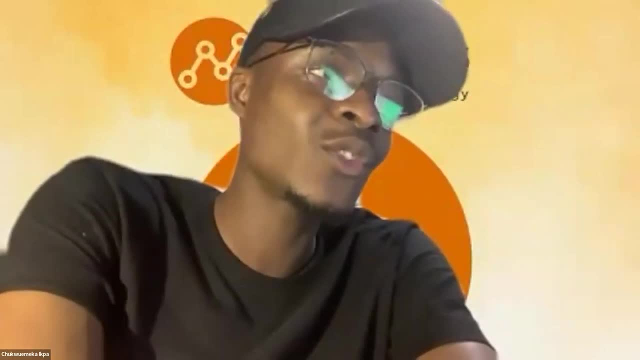 And then, before the class is over, I'm going to play a couple of videos for us to see what the past students have to say, So that we get to understand what they saw and so we can know that it is not just us speaking. 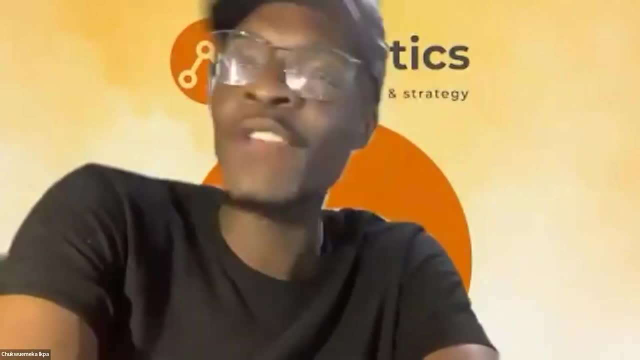 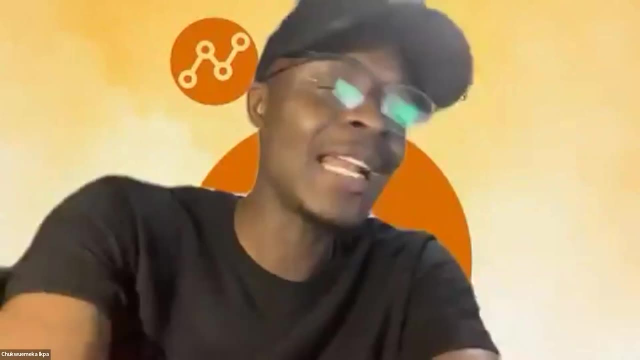 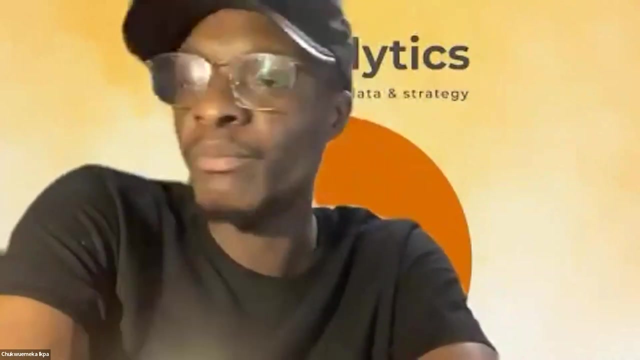 Okay, Fantastic. So if you have any questions at this point, you are free to use the raise hand icon to ask your question and I'll ask you to speak. or you are also free to drop your question in the chat box and I will pick it from there. Okay, So I think I've done it. I've answered at the most personal of the installment plan, where you also, if you want to make installment payments, you can use the first option of making the flat fee of possibly $450,000, then, before the 4th of May, you make the complete payment. 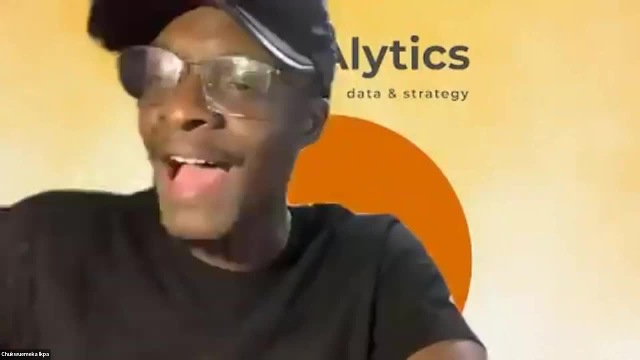 Okay, All right. So please, if you have any questions, just use the raise hand icon. Okay, Elvis, I'm going to call on you first. I've asked you to unmute. I have the floor. I'm going to call on you first, Elvis. 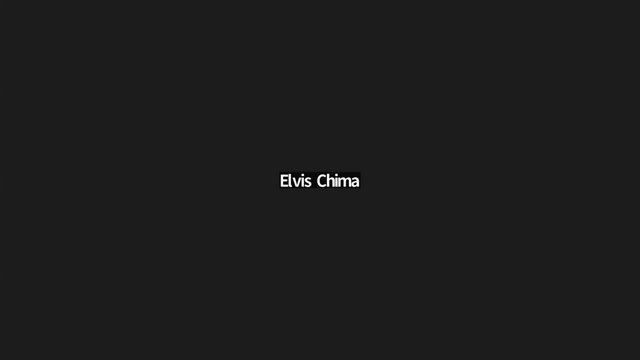 Yeah, Good evening everyone. Can you hear me? Yes, please, We can hear you. Okay, So I wanted to ask. you said this internship was going to be for three months. I would have loved to know, because I'm currently doing my master's, currently in the UK, in cybersecurity. 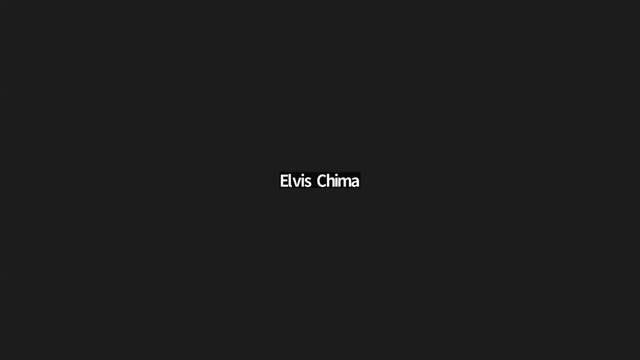 Okay, So my first degree was just computer science. So when I got here I realized that all my thoughts of cybersecurity was totally different from what it is in the real world. It was when I got here that I realized cybersecurity has different aspects. 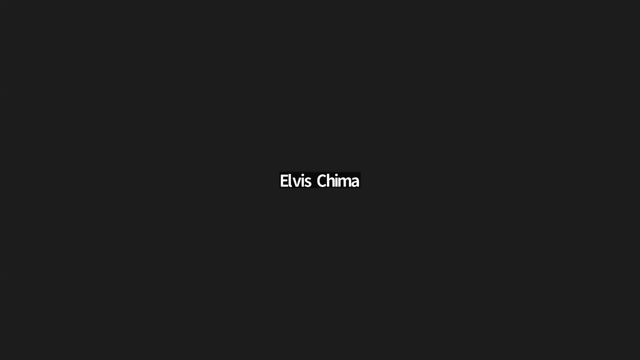 I thought it's just you want something like the way you have like a software engineer. So most of the things you mentioned here they've actually taught us in school. We've used some tools, like we've used TryHatMe, We've used Wireshark. 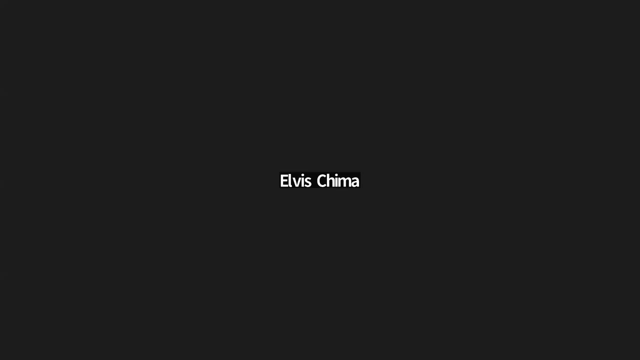 We are currently using Kali right now for Bobfield, Nmap and the rest, But then you know the way school is now. After the teaching class, it's expected that you should just go and still develop yourself, And I've not really been able to understand. 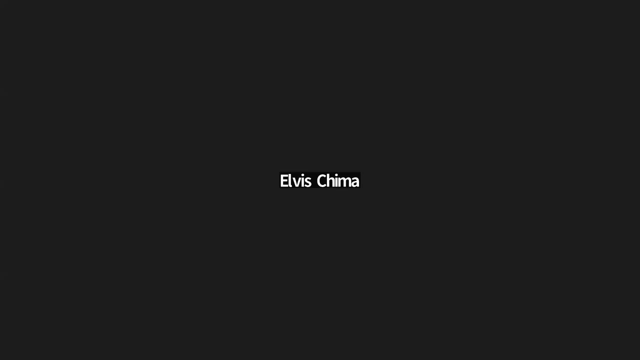 And that's why I'm looking for like internship where I could gain more practical knowledge on it, Because, like I said, I'm still new into the system. But most of the things you guys covered here are things I already know from from my last semester and this semester. 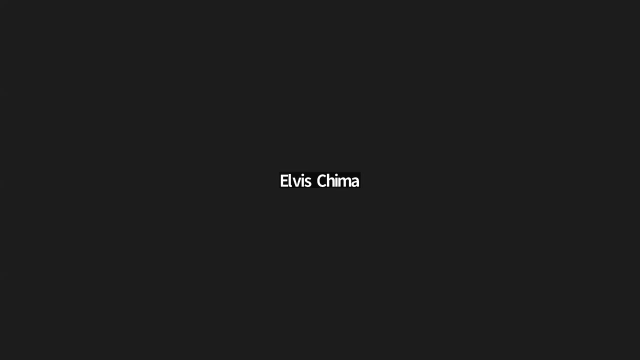 So I want to know what exactly are we covering in the space of these three months, Because what we covered last semester and this semester they are like 70% practical and just few. Sorry, they are like 70% theoretical and just few that are practical-based. 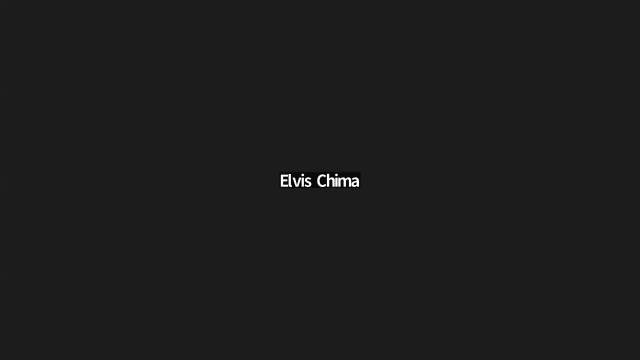 So if I'm to pay 500 pounds, I want to know a couple of the fact that in UK here now, you can't get a job. You can't just finish school. You can't just finish school. You can't just finish school and get a cyber security job, because they said you have to get one clearance stuff. 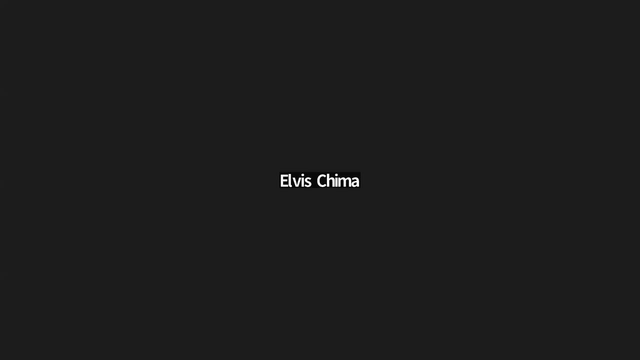 They will tell you you must have stayed at least three years in the UK before you can dive into the cyber security sector. That's why I know most of my colleagues said I finished before me. I came in last year. I knew a couple of people that came in two, three years before I came. 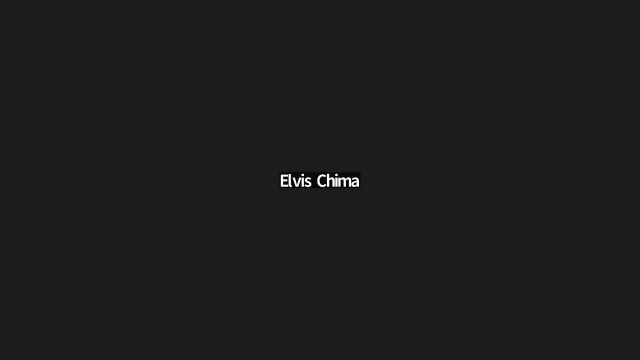 And they told me on how they had to start with. what is it called? they had to start with IT support jobs. Yeah, because it's a normal policy in the UK. They don't give jobs to new people Like you must have been here for like three years and you get one. 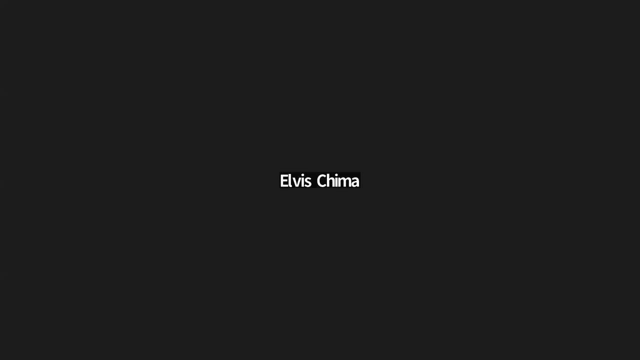 Is it police clearance? I can't remember what they call it, but it's the clearance you get before you could start working. So, from what you said, you said, if you guys brought someone, if we do everything that you teach us and we follow all your rules, 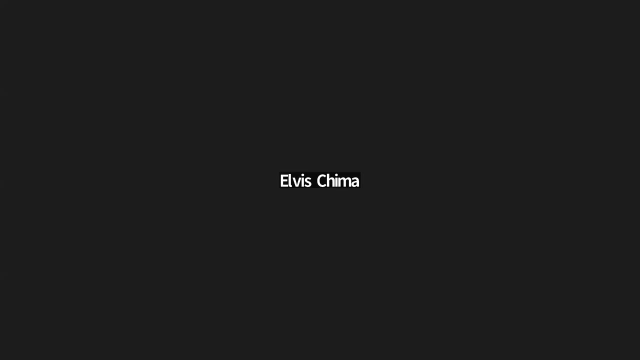 that you'll be able to get us jobs. So I want to be sure. I want to be sure because When I came into the UK newly, I think I saw Adiazar Suleiman. I saw him either September or October last year when I spoke with him. 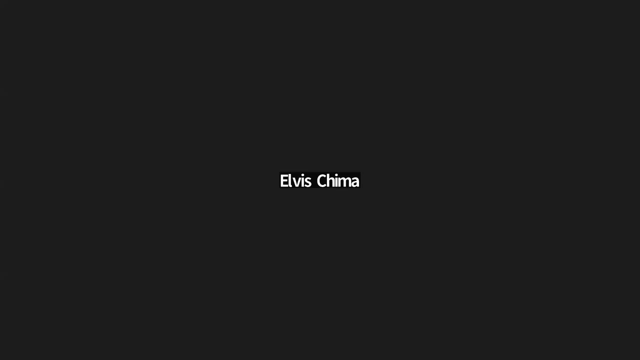 He said: you guys, in 10 analytics, you guys are not doing cyber security internships. He told me about data analysis. Yeah, so it was just like last week that I got to and you guys said there was an opening now for cyber security. 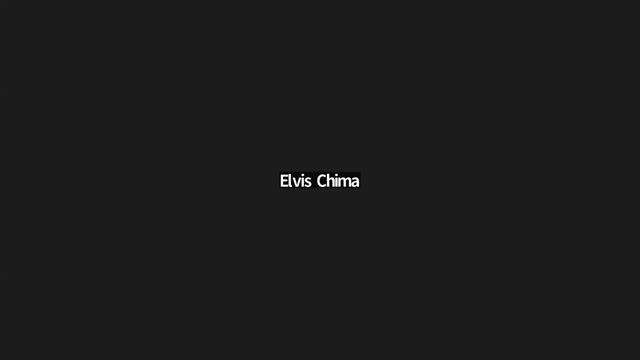 So I want to know now: Are you guys assuring us of getting jobs? Are you guys assuring us of getting jobs? Are you guys assuring us of getting jobs based on the results you have with other internships you've held? 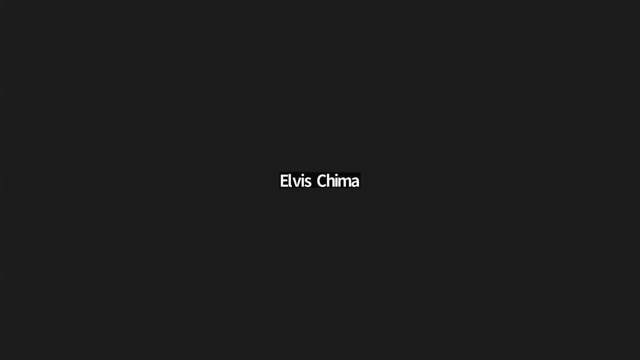 in other sectors Because I know when I came newly I was looking for where to just attach. Let me just be gaining some practical knowledge, because in school obviously it's not everything you gain in school. There are things you can gain in internships that you can't learn in the classroom. 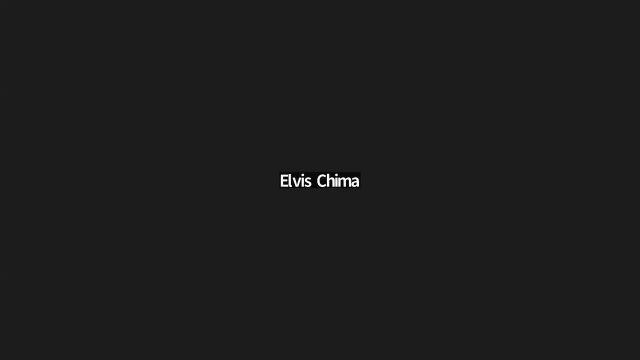 Like CV review, preparation for CV review, preparation for interviews. Your lecturer has to teach you that, So I want to know now if the job and your previous students you have are actually people in cybersecurity too that you've actually gotten jobs for, or 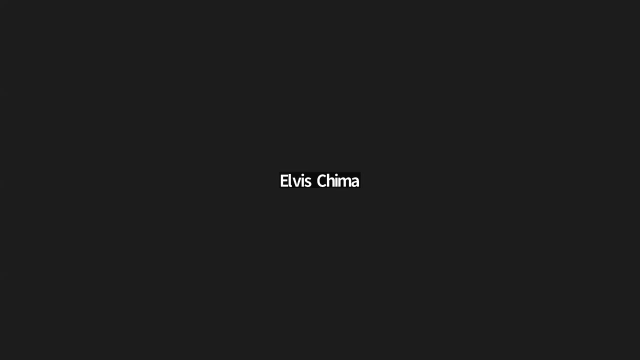 you are saying this is based on your experience you have with students. you've actually trained in other aspects like data analytics. So that's my question. I want to be sure on what I'm doing before I get into it, because I've had many people. 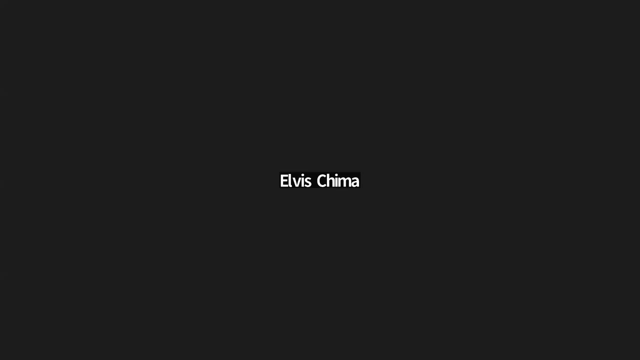 say they've studied cybersecurity. We even say, if they have known they would have studied project management or something easier- Cybersecurity. now you need to do a lot of trainings, a lot of certifications and all of that. So I want to be sure 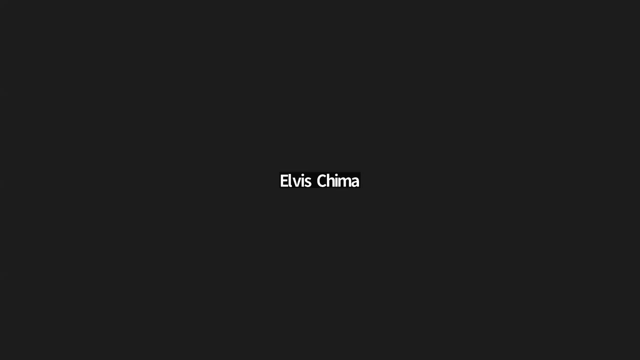 of what I'm getting into, because £500 is actually a huge amount of money. It won't be huge compared to the training and other benefits that you're offering. So I need to be sure first before I know if I'm going to proceed with this or if 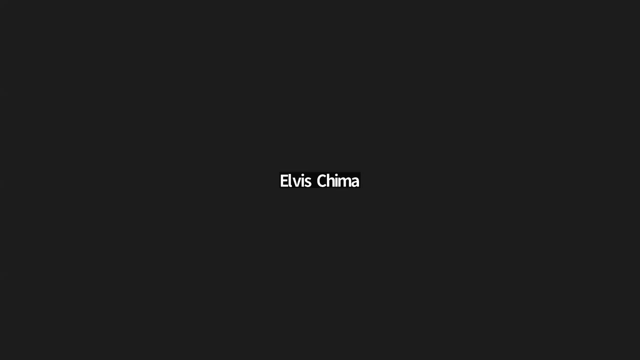 I'm going to be backing out. Thank you, That's my question. All right, Thank you so much for that, Elvis. Please confirm that you can hear me. Yeah, I can hear you. So your question. I love the fact that you mentioned that. 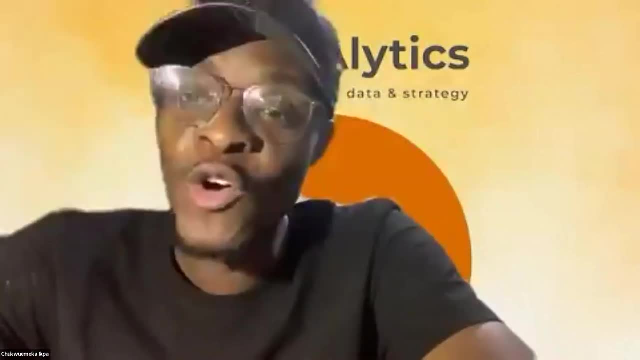 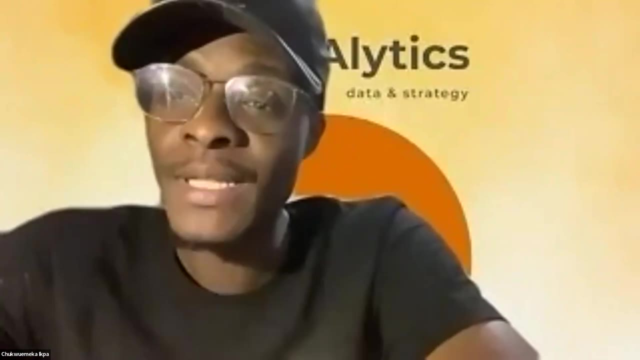 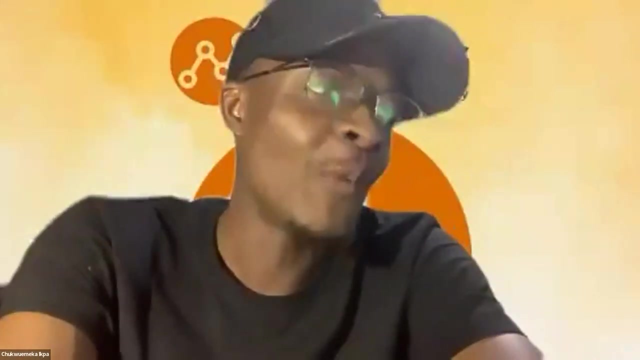 you've checked in before now and you noticed that we're not offering cybersecurity. So cybersecurity is just a course that we started recently. It should be in February that we started the first cohort. Okay, And we don't jump into areas without first understanding. 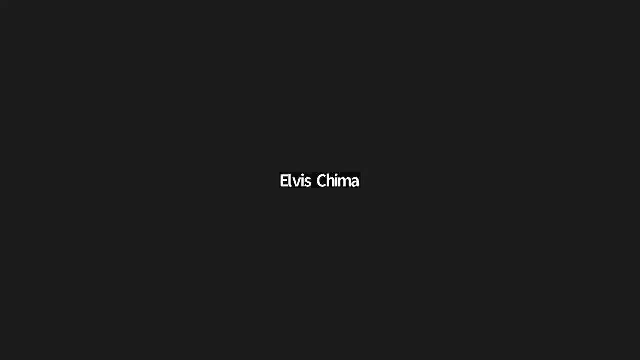 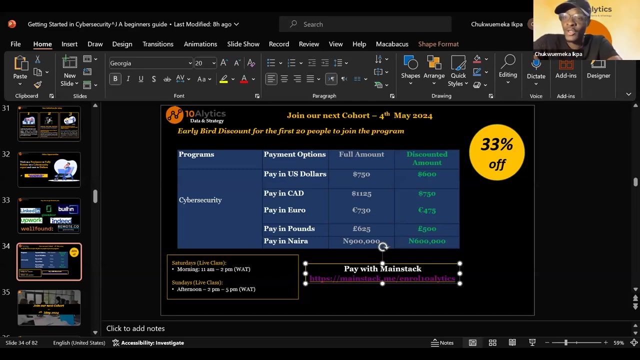 what we are trying to get ourselves into. So I'm going to paint some scenarios for you. I have a friend that transitioned directly into cybersecurity from Nigeria straight to UK And this friend of mine- he was in Nigeria when he started doing some of these remote 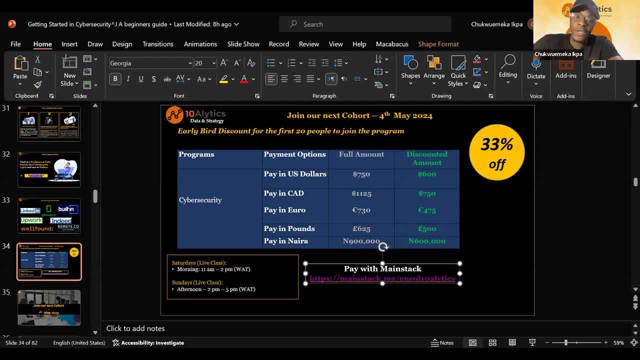 jobs for companies Outside there, And all these things stems from the quality that you are bringing in and the experience level that you are also going to showcase to them. So, at the moment, though we have our first, At the moment, though, that we still 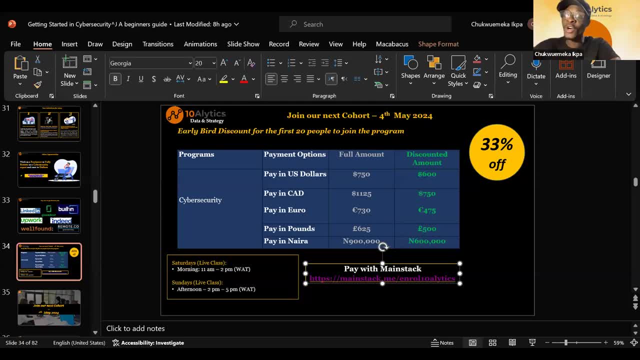 have our first cohort in class, but I'm telling you from prior experience that you can get jobs in UK depending on your skill level as at that point in time. So you know companies can give you leverage when they know what you are bringing on board. 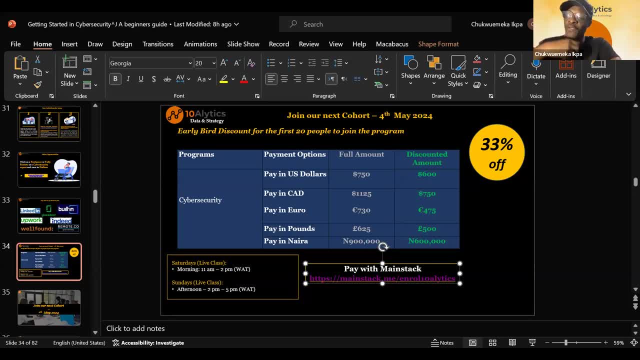 But they may not be willing to do all those things for you. if you are coming to get the job and you have zero knowledge of how to be practical in the aspect of cybersecurity, You are coming to cybersecurity and not understand what networking is all about. 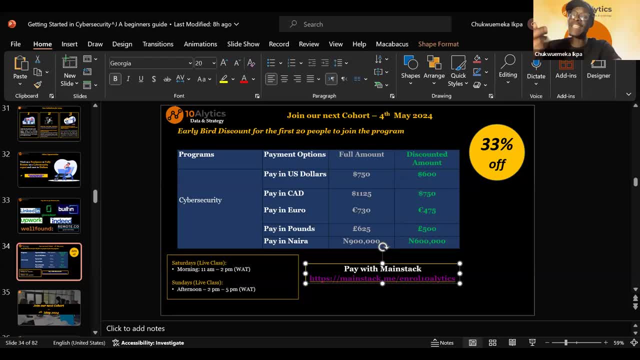 They are going to feel like, oh, this person is just going to take us a lot of time And that's why Phonam told you that you need to have all those long period of time. Yeah, even though we have testimonials, we have newsletters, we have 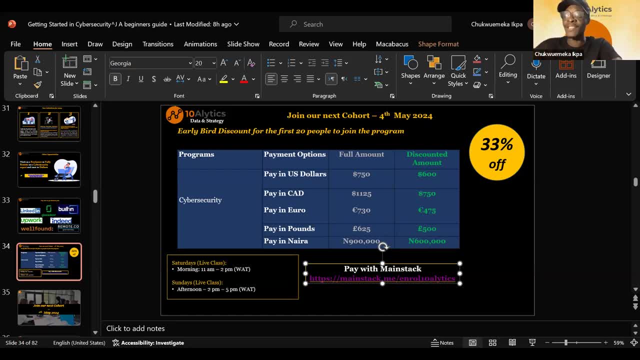 newsletters already trickling in in other programs. At the moment, our first sets in cybersecurity are still in class. We have close 30 people, close to 50 people, currently in class Right. So they are currently undergoing training And you know, cybersecurity is not an area. 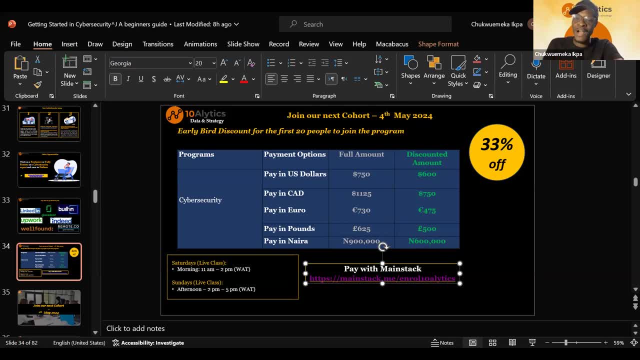 where you just learn cyber security and you can easily get the job. No, it's not. It doesn't function that way. So cybersecurity actually is an area where you get to. you know, have that full training, learn the basics from the basics to client, to client, to client. 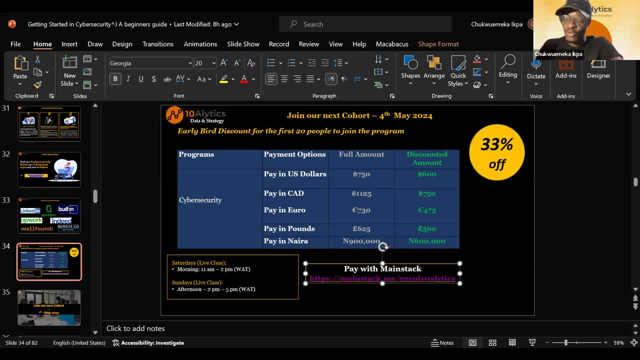 to the midpoint and then learn how to use necessary tools. like you mentioned, learn how to use Wireshark, Boxsuit and Zap to be able to intercept and prevent threats. So, at the point that you are fully skilled in all this area, I know for. 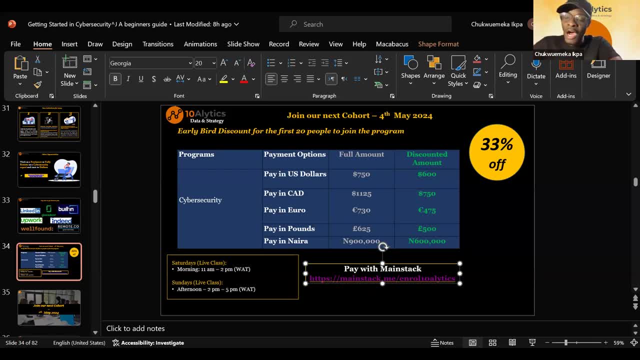 Canada. for Canada there is no request for police reports, But for UK I can't confirm that at this point- whether that police report is actually what is very, very necessary or whether it is what is used to deter people from getting into that ecosystem. 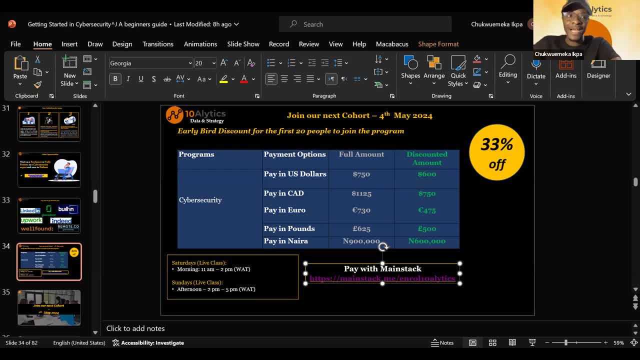 Just like what people always tell you, that this needs to exist, that for you to get a job in UK, you need UK job experience, Or for you to get a job in Canada, you need Canadian job experience. That is just a myth. 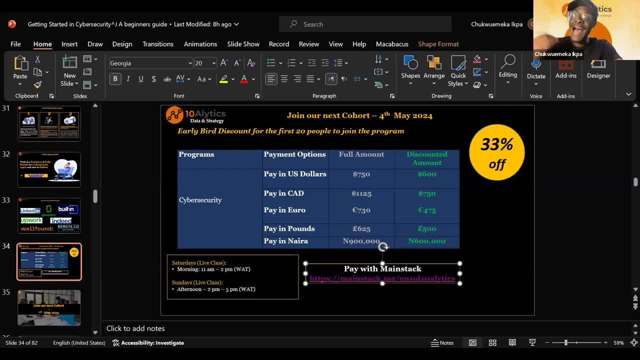 Right, It is just a myth. So for us, you can have evidence to show that you have all these areas, that you worked in the areas of cyber security, and that is what we are offering you, Because our courses are not just theoretical like normal. 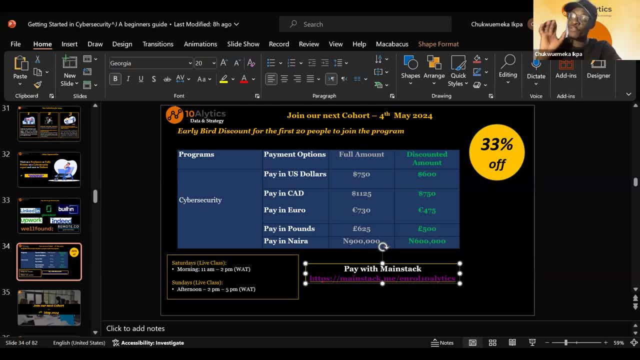 master's program or PhD class. They are fully practical where on each day you come to class you are working on a case study, And that means by the time you are done with your three-month program and your one-month internship, you have close to five to. 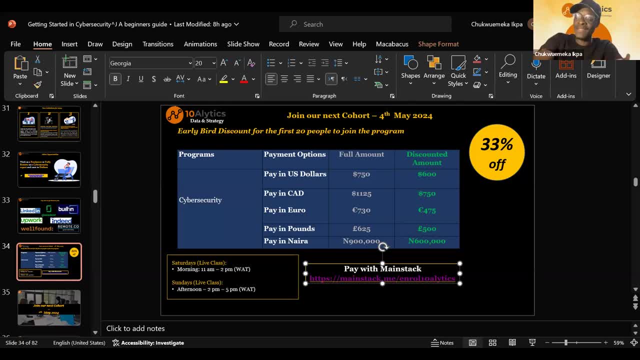 ten projects that you've worked on relating to cyber security. So all these things, they are what recruiters are going to look at and say, okay, Elvis is our original and experienced cyber security person. Because you have this, you have that Right. So we provide you case studies. 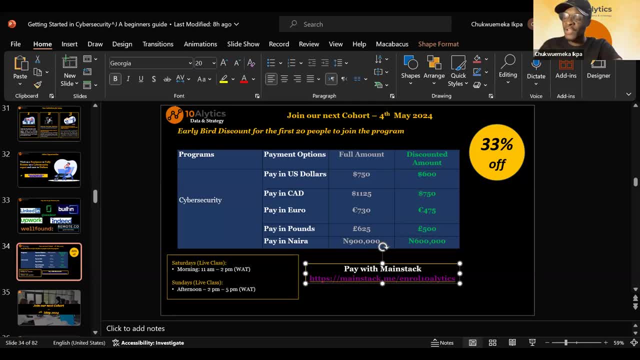 from the financial sector, case studies from health, case studies from energy, where you get to practice them. So it's as good as saying that you, Elvis, has worked in the energy sector. Right, Because you have that data from the energy sector. 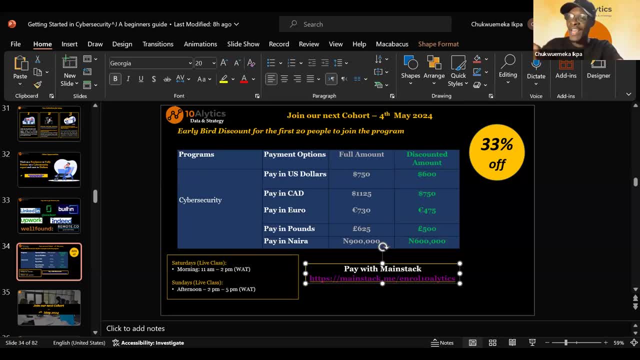 that you have worked in. So basically these are things that will help you to build up and put in your portfolio so that will make sure that at any point any recruiter is trying to have conversations with you can confidently defend and you know answer. 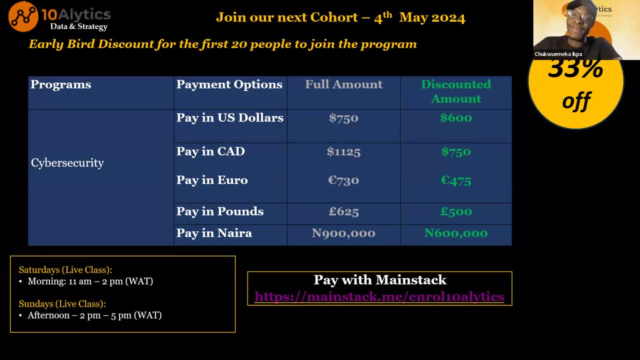 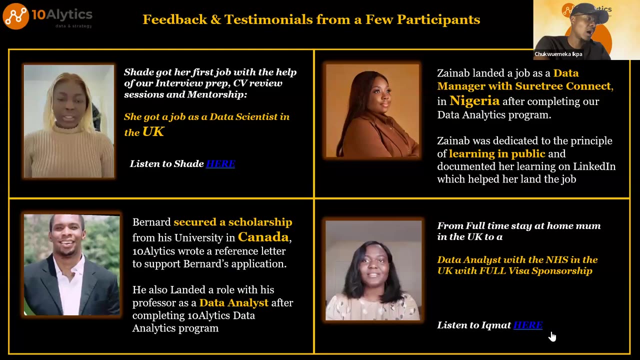 yourself. So, at this point, our first set in cyber security. they are still in class, but we have numerous other programs where we have amazing testimonials, So I'm going to play a video from someone so that we can better understand this. I'm going to play a video from: 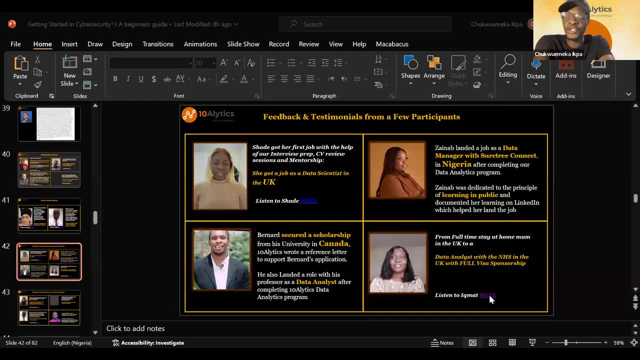 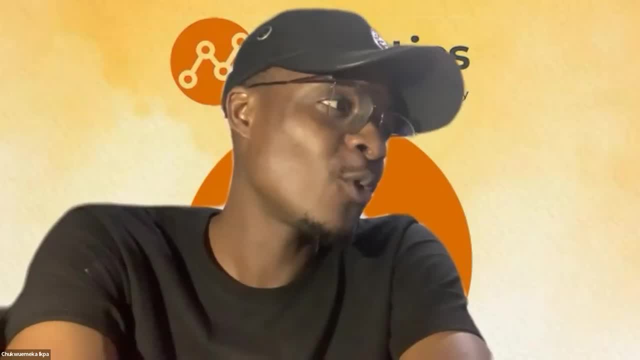 Iqmat. So Iqmat was able to transition as a full-time housewife into the tech ecosystem Right. So I am going to share my screen- It is coming up right now- so that we also get to understand that these things. 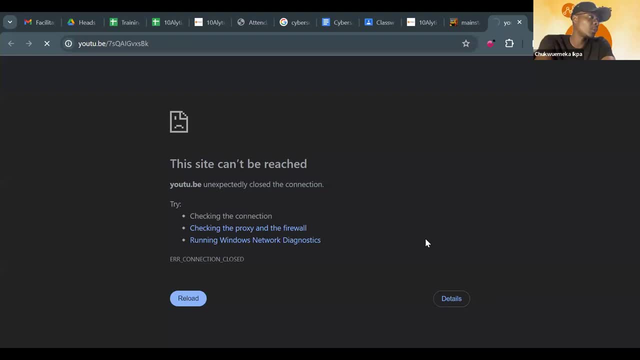 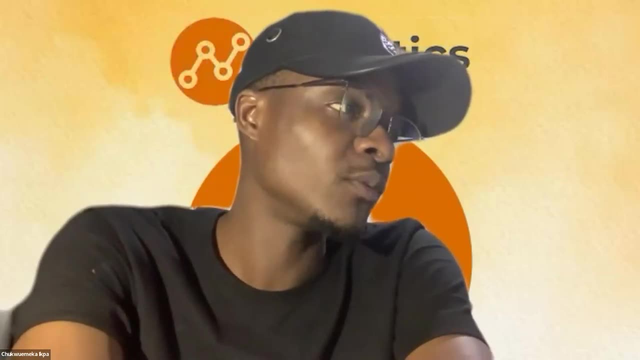 are possible. Oh, internet is interrupted. Okay, It is still coming up, please. But, Elvis, I don't know if I answered your question. Hi, Elvis, are you there? Yeah, I'm here, I'm still here. 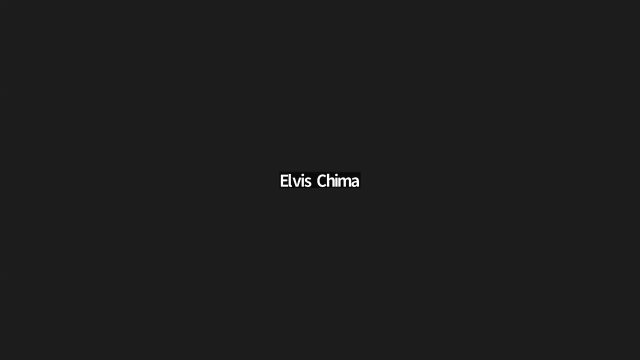 You've not really answered me directly because first semester I did three months. Three months is roughly 12 weeks you get. But the knowledge I gained in the three months of my first semester is not what I could use to go to any employer right now. 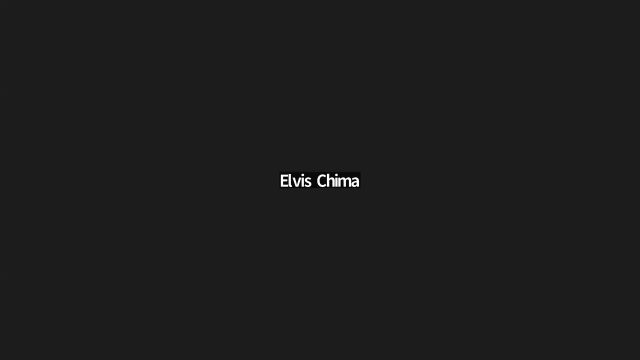 You get my point. So if you're also offering me three weeks, I paid about 19K to study cyber security here, But then in what they've taught me in two semesters I'm not still fully ready, Like at times I feel like I. 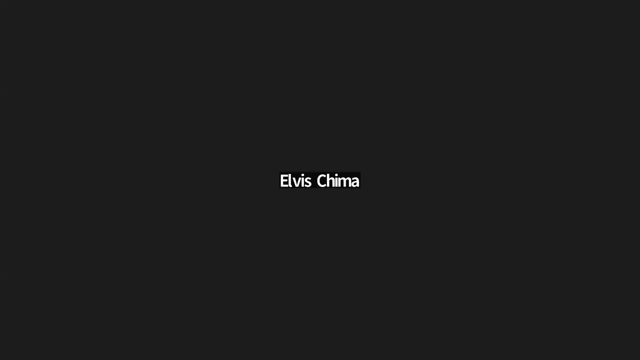 wasted money you get. So paying 19K on first semester one of the courses they were teaching us about wireless networks. They taught us about all these intrusion devices, honeypots, all of that. So you get, but that's not what. 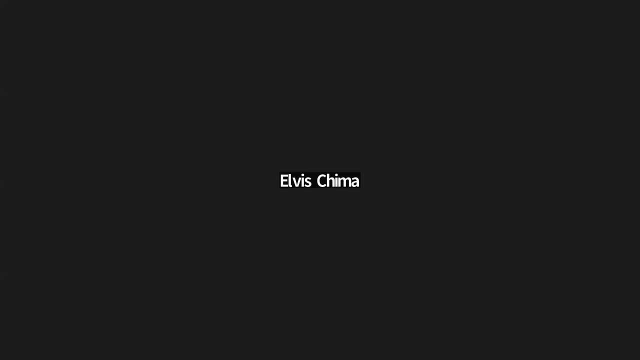 if you go for an interview, that's not what. nobody will ask you what is honeypots in an interview? Most times it's normal, real case, life-based scenarios you get. So if I'm doing, I did like two semesters, Two semesters. 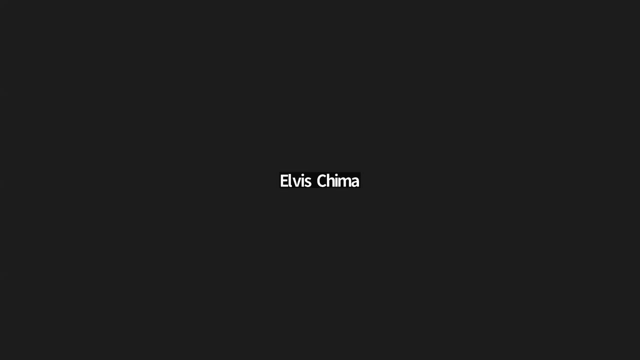 about six months roughly. Yeah, I'll be finishing my second semester next week and then, from now till September, I'll be doing my dissertation, and that's why I saw this opportunity as a great one for me to still study while I'm doing my dissertation. 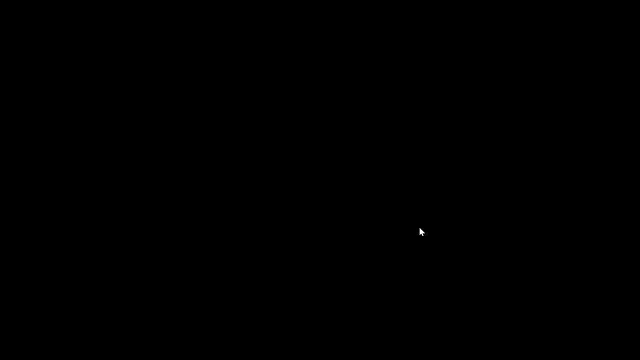 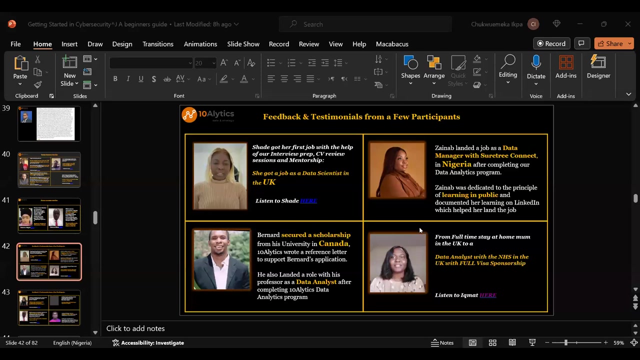 So my point is: if in Can you still hear me? It's like I can hear you, obviously, Okay. so my point is now: if in six months, six months of lecture, or in one year of studying, I'm still not well equipped, 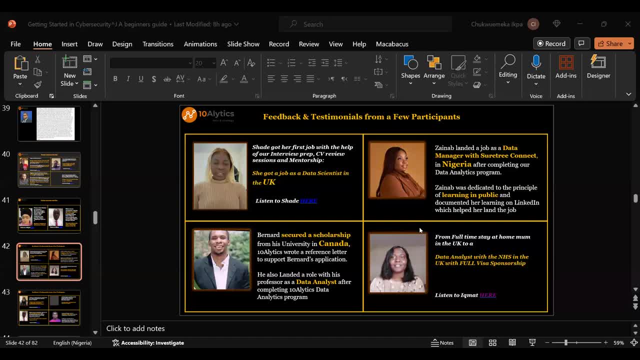 So I want to know what are those things now because, like I told you, they already introduced us to Wireshark. Currently, in this second semester I'm in. now we are doing a course because it's ethical hacking. Ethical hacking, that's what they taught. 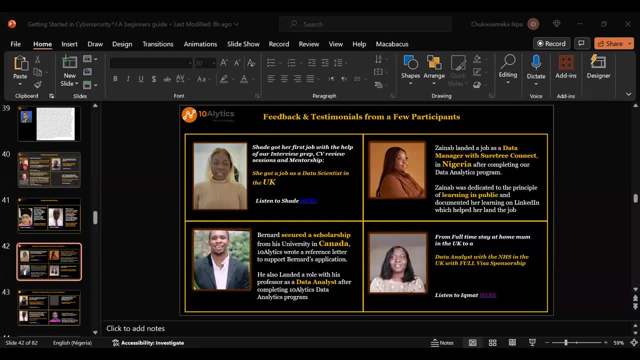 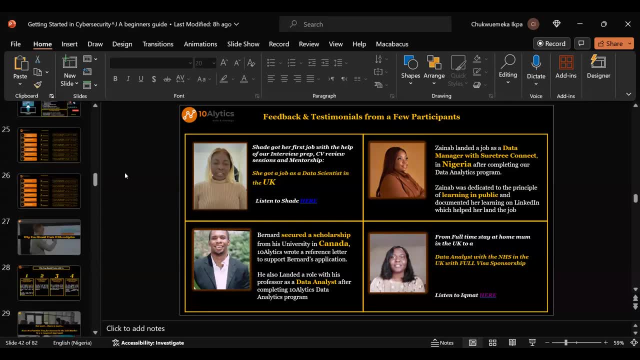 us how to use ZAP Bobfield, how to use Nmap and the rest of that. We use it in Kali. We also use VMware, So that's why I said most of these things you guys said are things that I'm already kind of familiar. 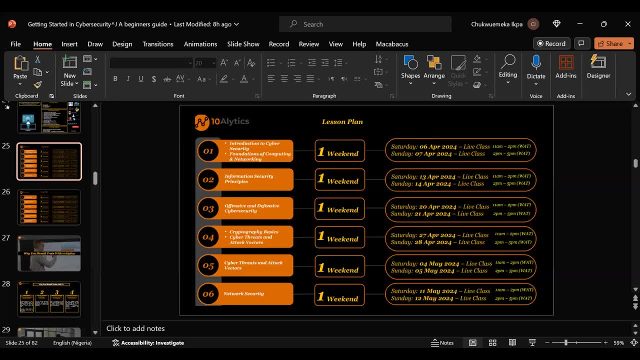 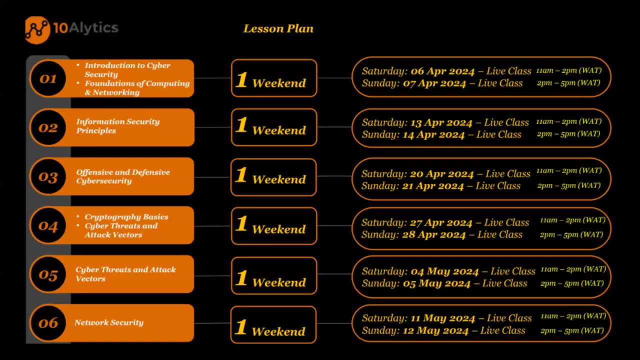 with. So that will not say I'm strong, but you are not really new terms, Like they are not really new words to me. I am already familiar with most of these things you guys said. So I want to know now: what exactly are your? 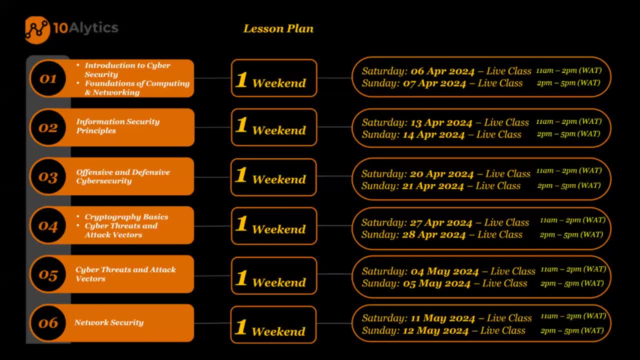 Is it, at the end of it, you have recruiters that will come in, and you have recruiters that will come in and, at the end of the day, you help us get a job. or Because let's say, for instance, now if you have partnership, 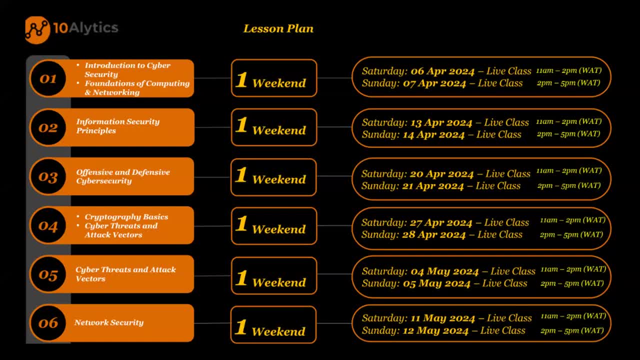 with any company that from time to time, like you said, like from time to time, they can come and ask. because, From my experience, I was even thinking. I was even thinking of maybe going for a boot camp on data, on What is it called? 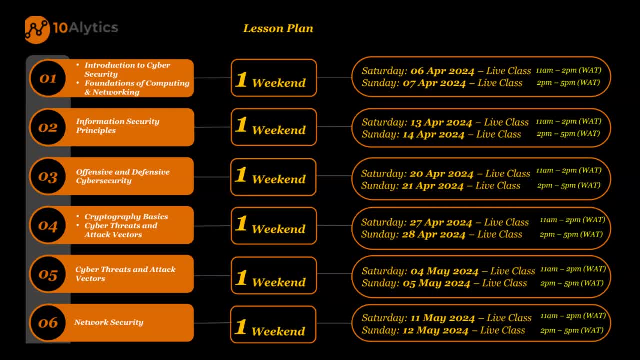 This Data analytics or two. I was thinking of going to a boot camp on that or a boot camp in project management, just so I can stay for three years and build and work, earn money. Then in that three years, practically learning, going for certifications, building my 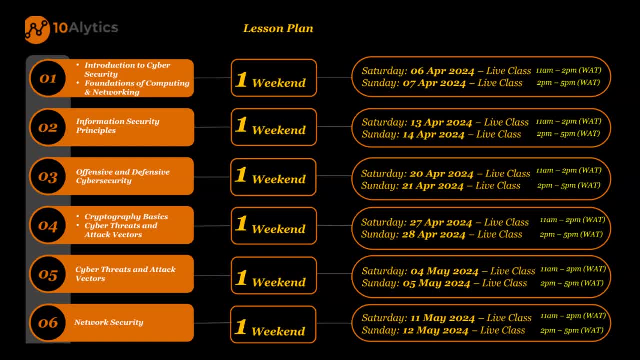 CV and still diving deep into the cyber security field. So is it that if we finish this internship now, you will help us get a job or you will just give us hands on training? then we'll develop ourselves and we'll fall back to going to apply for jobs. 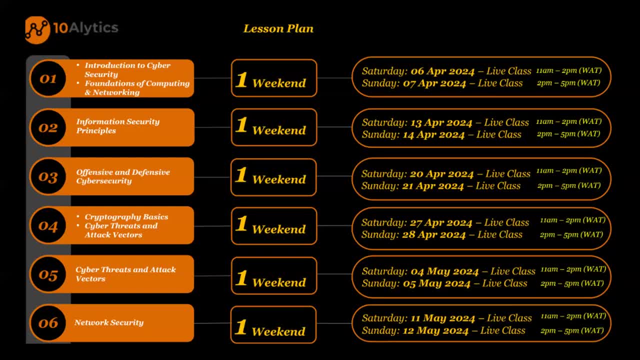 again and see here in stuff like, okay, you can't get because I've applied in many places. Hi, my name is and I was with the March Corps intern and it's and joining. that's not supposed to play now. Sorry about that. 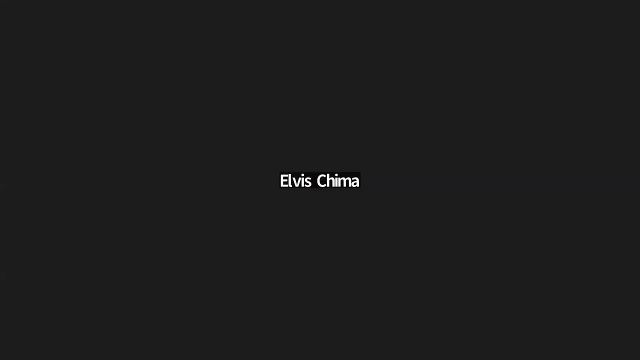 You know, for me someone coming from a background of Okay. so, like I was saying, is it that you're going to help us get a job? Do you have recruiters? Do you have people in cyber security that you can say, okay, we can beat you under our chest? 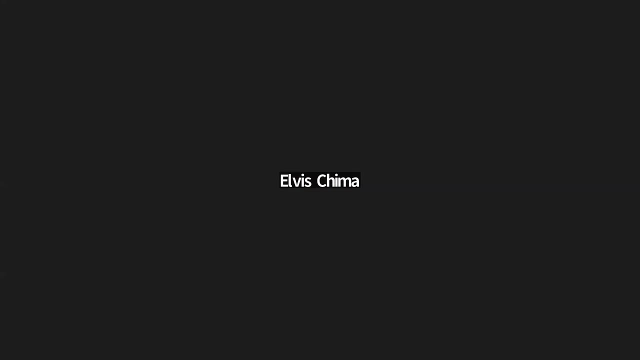 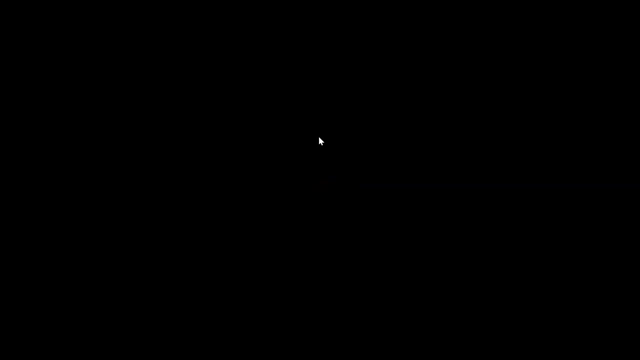 and see if you learn 90 or 95 percent of what we're going to be teaching you, if we help you review your CV, if we prepare you for all these interviews. are you assuring us that we'll get jobs or you're just? 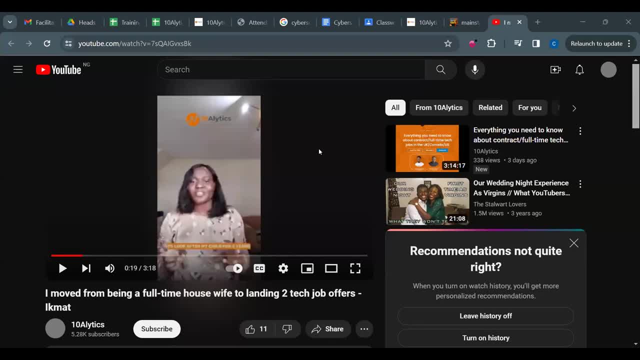 helping us gain more knowledge on cyber security, and we'll still fall back to having to wait for three years, Because I don't see any reason why I would want to finish my school and I'll go into internship if I'm not certain that I'll be getting a job. 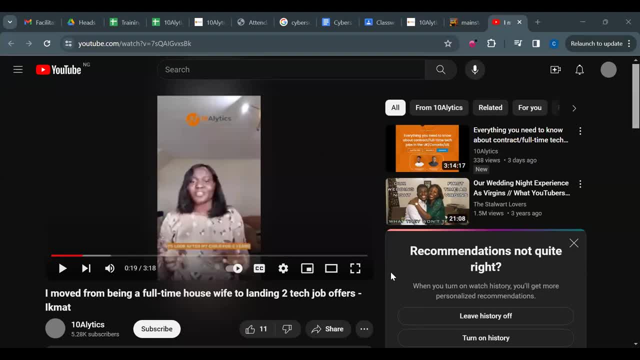 after that: Yeah, because it's a job factor. I told you in UK- I don't know about Canada or US- In UK here nobody will give you a role in cyber security. I have people that came in like two, three. years before me, All of them. now they're into project management, they're into IT supports. Most of them work with NHS and because you know, at the end of the day you still need to get a sponsored job to remain in the UK. So 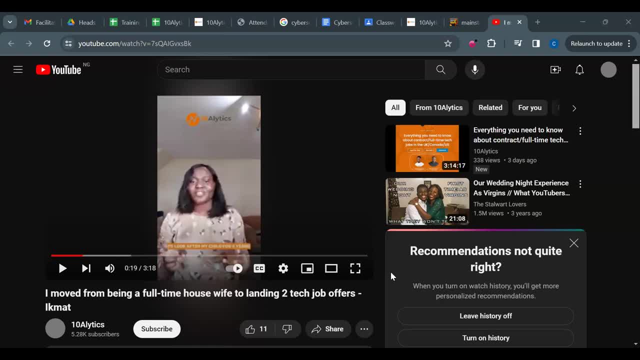 all these things are what I want to try to understand. Let's not be that okay, we'll just pay the money. Maybe people in Nigeria, now, US or Canada, they might not face it, But me, I'm staying from the aspect of me living. 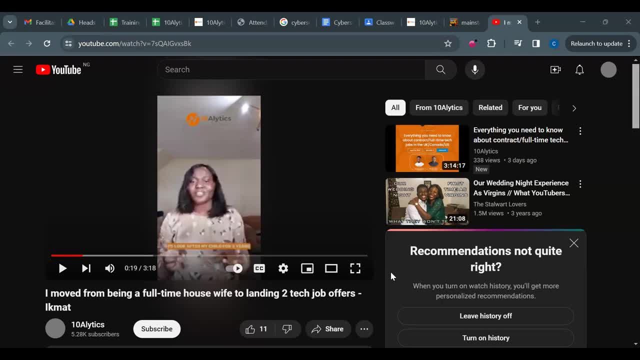 in the UK. So I want to know what exactly are you offering us? Is it that after your training we'll just be there on God hoping to get a job one day, or you actually are showing us that you actually have partnership with some companies that will come to you? 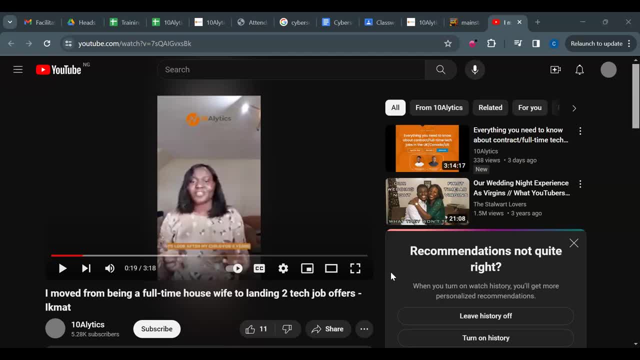 and say, okay, you just finished your May cohort. Do you have good people here that you can recommend to us to come for interviews? Are you going to be offering that as well, Or you're not sure for now, since your first cohort. 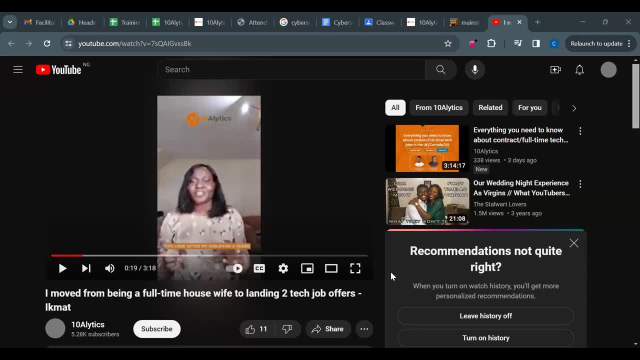 in February. they are still in class, All right. Thank you so much for that, Elvis. So one assurance that we have partnership with recruiters that come to us from time to time to ask for specific role-based people, right? So we've not positioned ourselves. 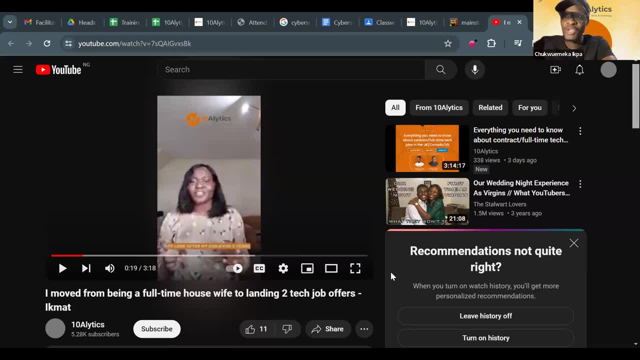 in respect to bringing our cyber security to them, because we are still having our first cyber security guys still in training. But our assurance that I'm giving you is also that once this training is completed, we have also positioned ourselves to be able to provide people from in-house. 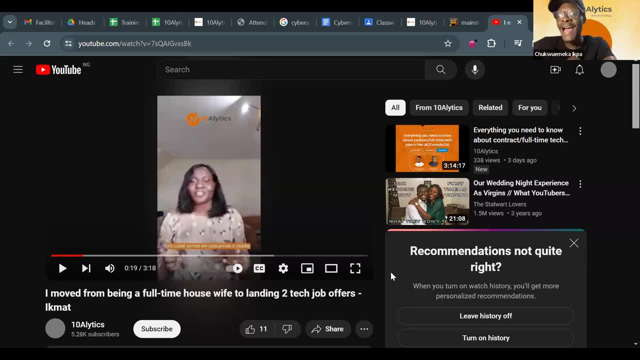 to them for job interviews. Now you're asking for specific job. specific assurance is now you pushing- I don't know how to put it- an entire hand, because this is just like saying you need assurance to someone that helped you come into UK. 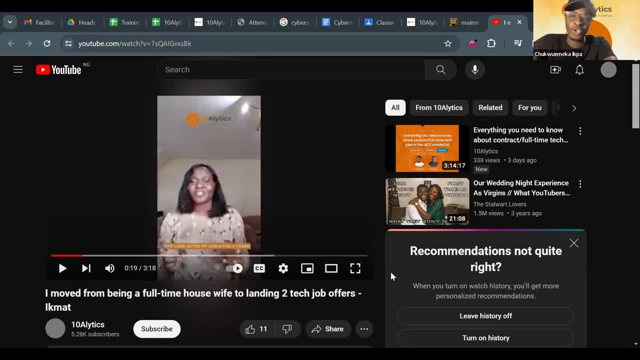 that once you are done with your master, they are going to get a sponsored jobs. right Now these things exist. For example, now our data engineering, data analysts. we give these assurances for people that do not get these jobs- yes, People that get. 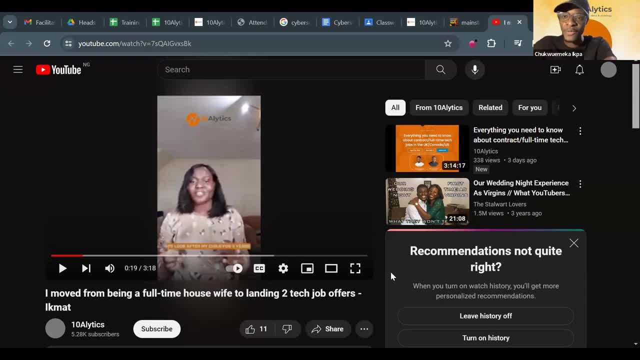 it, yes, And it boils down to individuals most time, because we have job application trackers where we have even told people that we've trained on a weekly basis. you have to apply to up to 100 or 20 or 100 jobs every week. 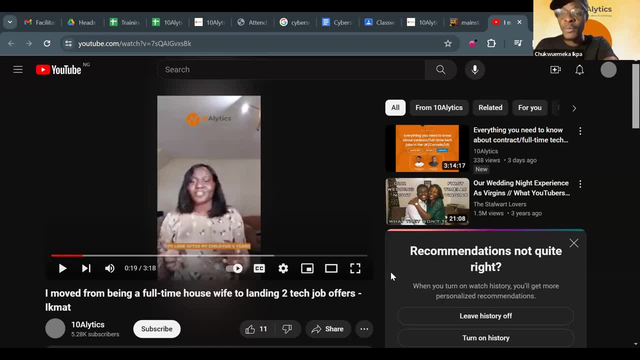 But you end up seeing people apply to just five jobs in a week and they expect things to happen. So from data that I've reviewed, from what Economic Forum reports, these things is not just applied to three jobs in a week and then you get. 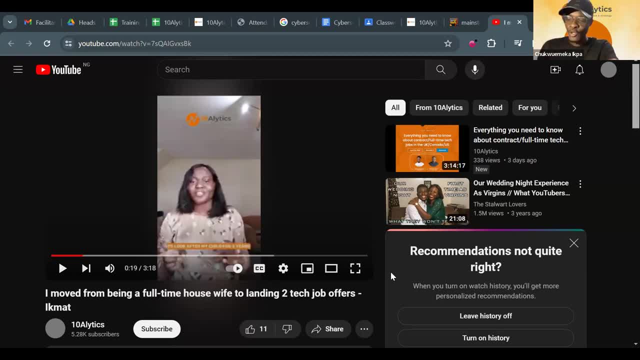 a job. We know the economy that we are constantly in. So, on day-to-day basis, people are expected to at least apply to 10 to 20 jobs every day. 10 to 20 jobs, And an assurance that we are giving you is that. 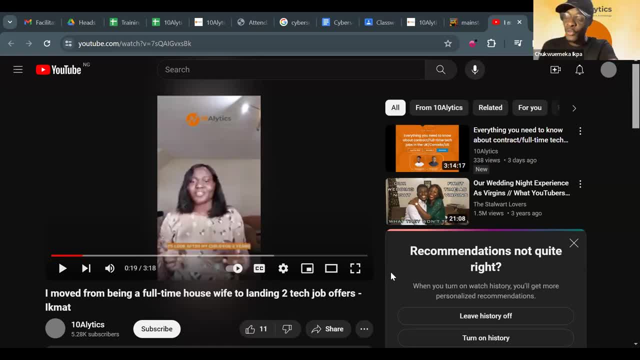 if you do all these things- that we are going to walk you through the mentorship session, the CV review session, the job application session- is that you are going to get one job interview after you are done training with us. It is a full assurance because 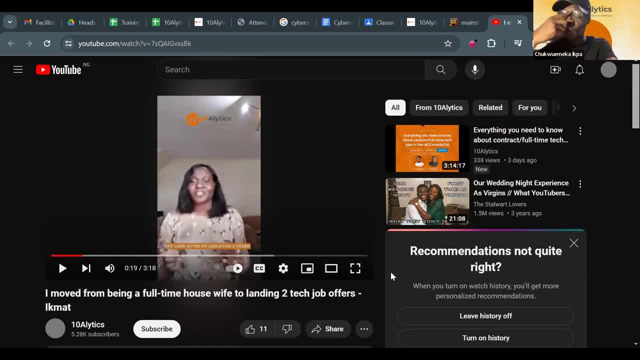 it's something that we have constantly experienced over the past four years, But the problem is this: now We have students that in a week they've not done any job application. If recruiters reach out to us, we are definitely going to position people that we've seen. 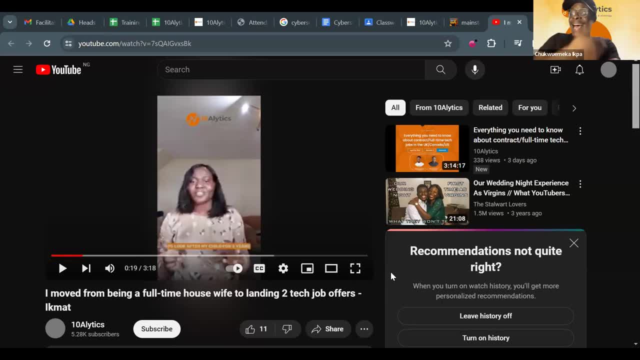 that are applying to this And those other people that are not applying to jobs and sitting down will now come and say: oh, I finished, I did not get any interview. So it still boils down to our personal push for all these things. 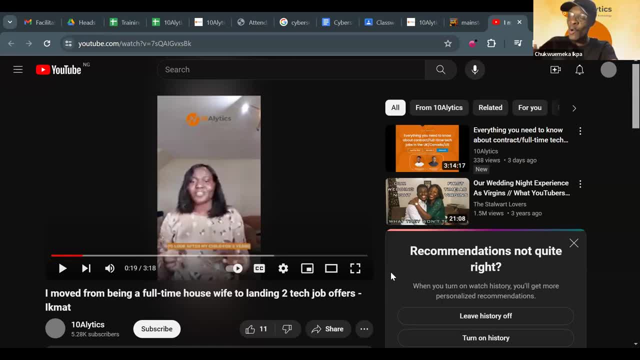 We are going to equip you with the necessary skill, competency and employability services that you need. but also there is a full expectation from your own side to be able to push for these things And not just from the angle of relax and say oh. 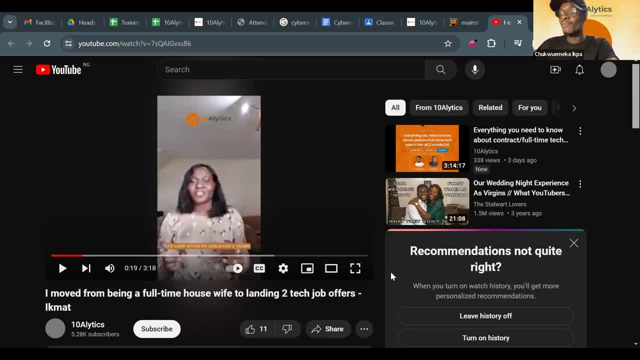 are we assuring you that you are going to be pulled from the pool to job interviews right Once you've done everything that we ask you to do? do the job applications that we ask you to do, 10 to 20 every week, every day. 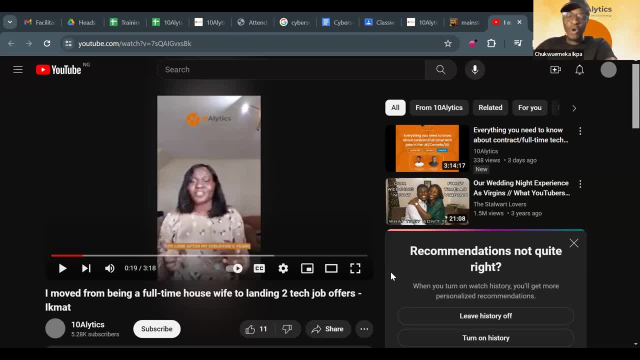 we are assuring you of one job interview once you are done training with us. So I want to play what Matt said. Okay, sorry, I have one last question. I have one last question before you play the video. Now, like I said, 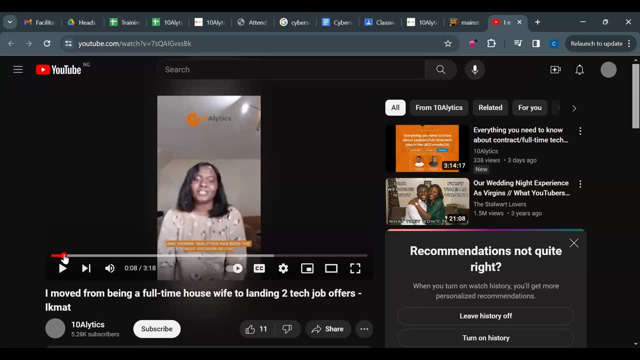 like I said in cyber security in the UK. I don't know if you've made your findings or if you still plan to make your findings, but cyber security in the UK, yeah, you need three years, Like it's part of the criteria. 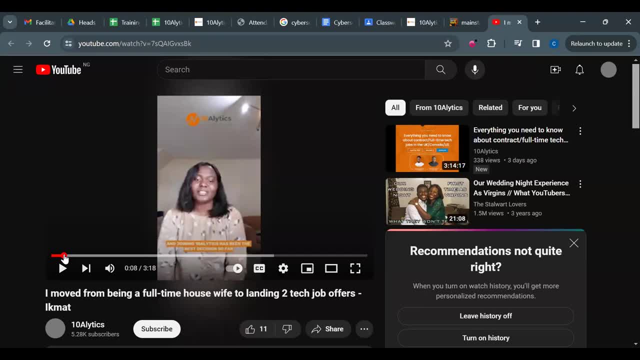 you must have lived in the UK. The same way some people tell you that you need to have UK experience, UK job experience, Some people now will tell you you need to have UK, but cyber security specifically, you must have lived there for three years. 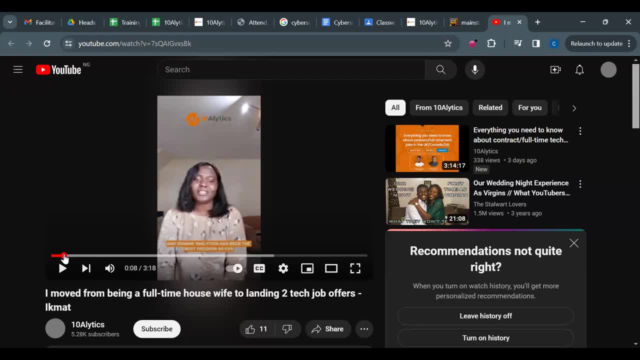 So how do I bypass that? I don't know if maybe you don't understand or if you could help me ask around just to be sure I understand you 100%. Elvis, I understand you 100%. It's just like a. 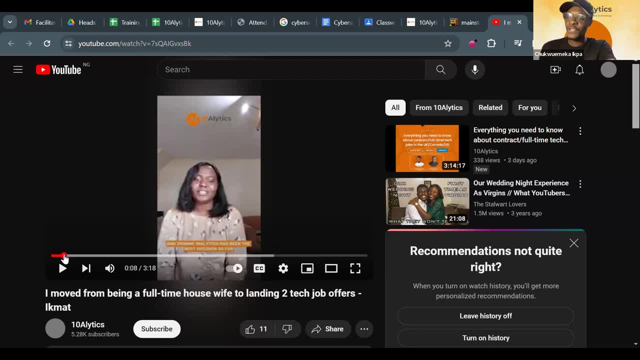 nurse moving from Nigeria to UK. When you get to UK you still have to do some necessary certification that pertains to that skilled area that you are trying to get into. There are some areas they want to get into- cyber security- and they require you to have that exact. 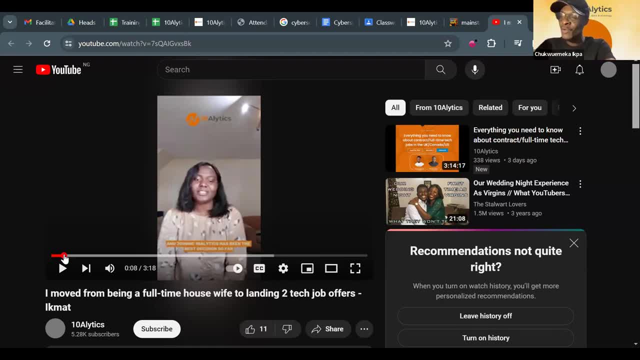 role. But for you to start off in the cyber security world, it is not a necessary position for you to have that three years, right? So there are start-up roles that exist in cyber security that you can easily start yourself up with, right. Why keep pushing? 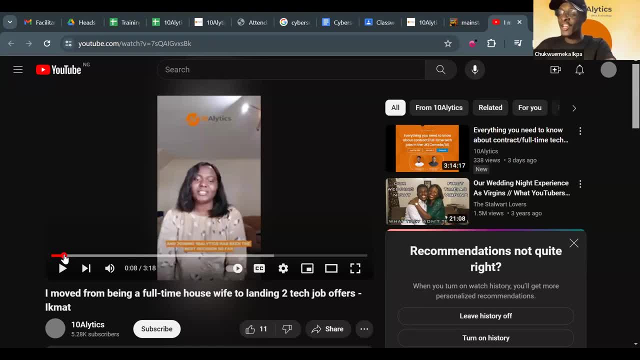 until you get the necessary timeline to get the higher areas. If someone is trying to get into things like, let's say, medicine, you can't just move from being doing housemanship to jumping to becoming a specialist. right, There are specific intervals that all these things follow. So if 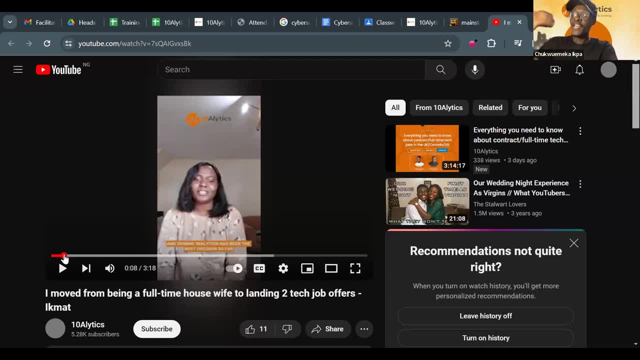 you are trying to get into the cyber security area, you're still going to start with all those lower-cadre cyber security and gradually also move up from there. right, All these you are going to achieve within that specific time. So when we say we are going to 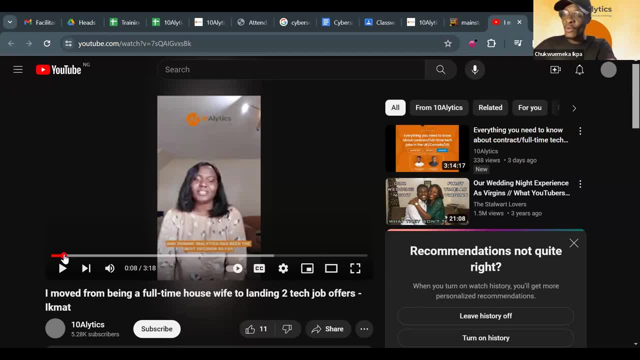 show you one interview, or one cyber security interview. it is not that you are going to be invited to be the CISO of a company, right, But definitely you are going to get roles that relate to security and cyber analysts, right, And these things. 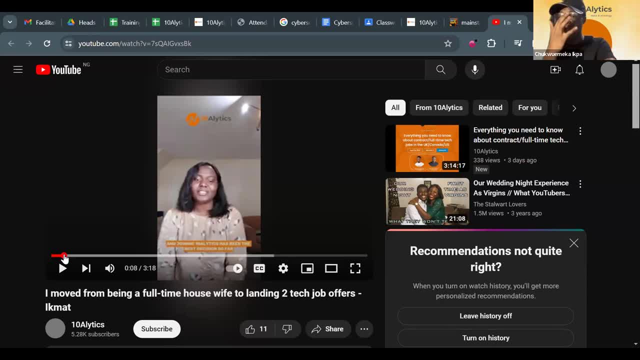 are. you know. this is also applicable to some of the things that we face in other areas where people will tell you for you to get into data analytics, you need to have two years experience in UK for you to practice. For all these needs, because for you. 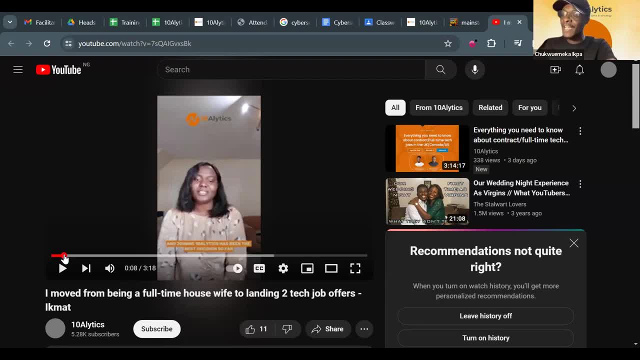 to practice. you just need the competency and skill and you will get into that exact core area and gradually climb up the ladder. Now, these are things that we also offer in our mentorship programs, where we teach about job hopping right, For example. you've got into 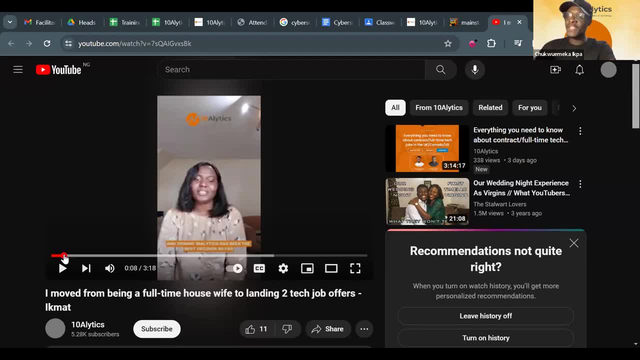 your first cyber security internship role and from there you've job, hopped into another role and gradually you've built up all those things that are needed. And all this is because we know how the terrain works out there, So we brought people that have 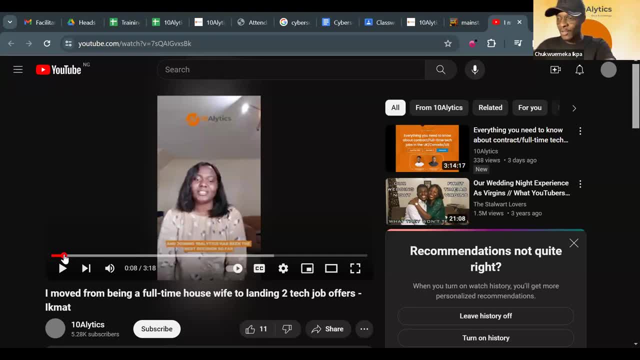 experienced this to walk people through how to do all this right. So we are assuring you, once you get into our cyber security program and you are done with everything that is needed of you, we are assuring you one job interview to get into. 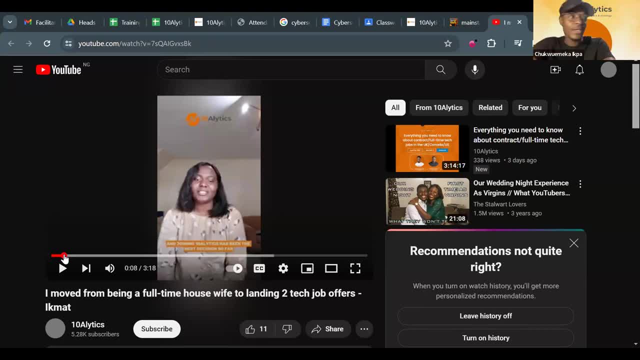 the cyber security job field out there, Hi, I don't know if that is clear. Yeah, that is clear. All right, Thank you so much, Hi, Michael. I think maybe I'll take you before we go on with others. 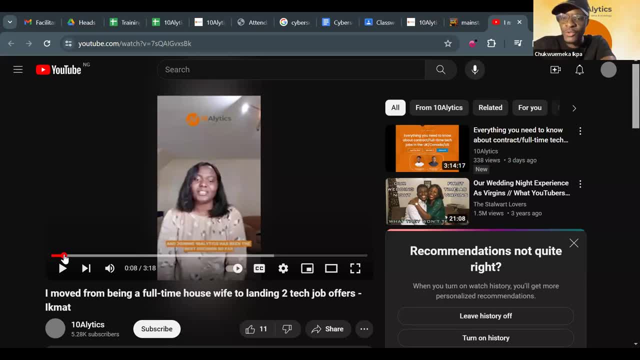 Hi Michael, We have the floor. I've asked you to unmute. Hi Michael, Are you there? Yeah, Can you hear me? Yes, please go ahead. All right, I think. thank you very much for giving us this platform to be able to. 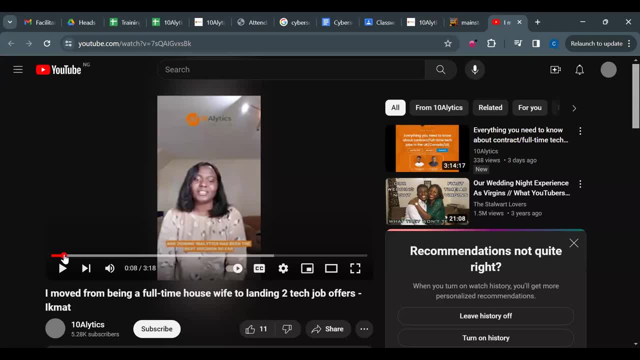 understand the cyber security aspect when it comes to joining 10 Analytics here. Previously, before now, I've done business analytics, business analysis and a bit of project management, And now I just felt okay, let me come into the cyber security aspect and see. 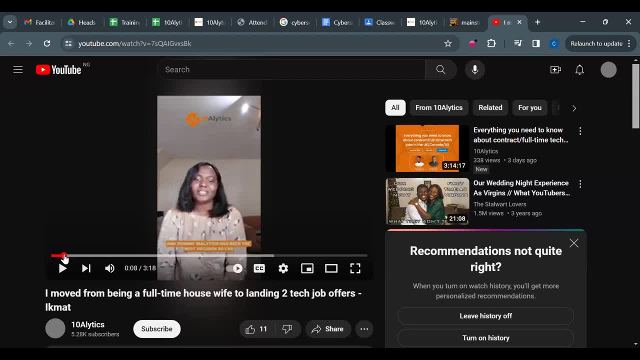 what it really entails. I'm just finding out. is there any way I could it could be linked? the cyber security business analysis, is there a link between these two fields? Or basically, are they just? is there any way it can be linked together? 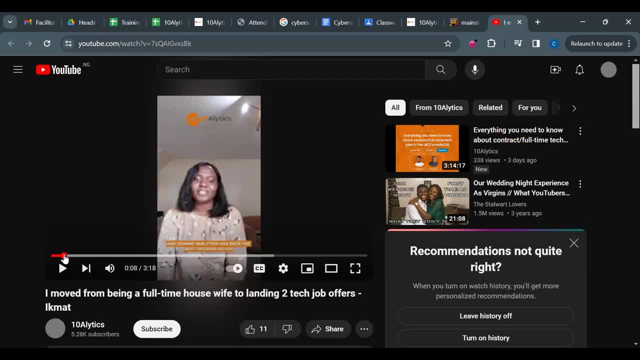 You know, using an idea you gathered from this aspect and also adding it up to what you have in cyber security, in the aspect of building up your CV and securing a job, That is where I'm trying to get my question from, So I don't know if you. 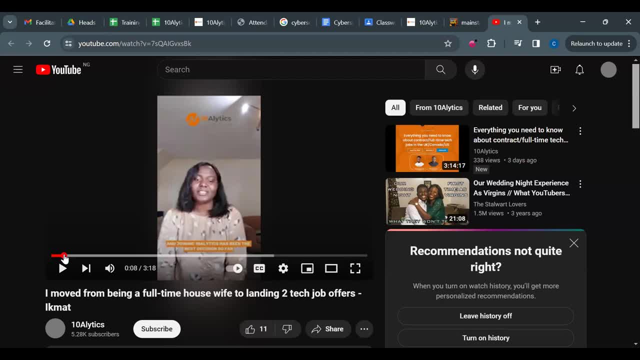 understand what I'm trying to Okay. Yes, I understand you perfectly, Michael. So your question is that: is there basically where there are transferable skills from business analysis to cyber security? Yeah, like building up your CV. now the CV. 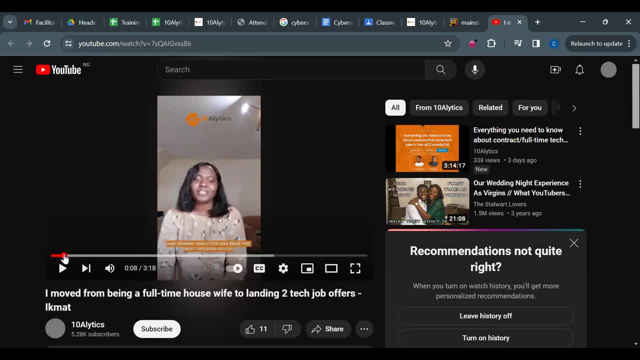 No, no, not with 10 Analytics, Not with 10 Analytics. Okay, so I can't- yeah, I can't- confidently speak on the tools that you learnt with the training institute, right, But for our own business analysis program, because we structure it in a way that it is. 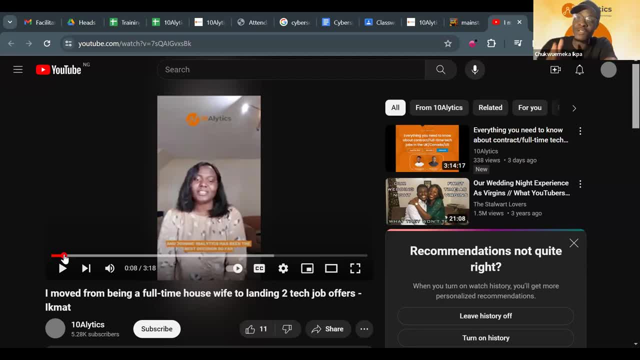 data business analysis. You get to learn Excel. you get to learn Power BI. you get to learn SQL, Like so SQL is something that SQL structured query language is something that has that little transferable language from business analysis to the other. 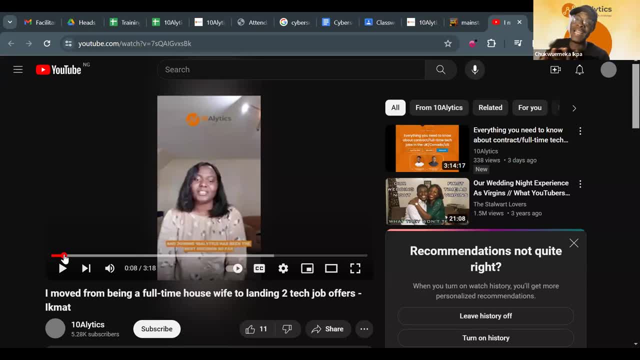 side right. So for our own business analysis, we get to learn this core data tools before you now enter into learning about Agile, learning about Scrum, learning about SWOT analysis, learning the entire business analysis. okay, elicitation method. 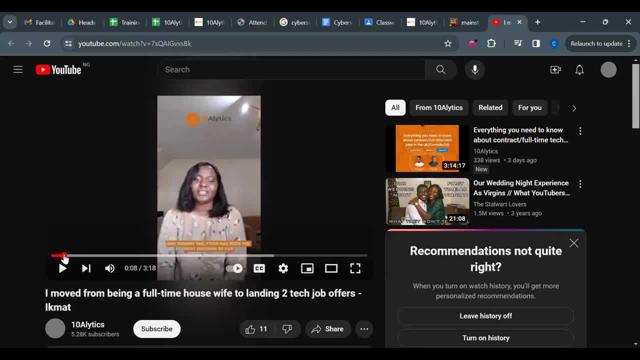 project initiation. well, we started off with learning those initial tools- Excel, Power BI and SQL. So if you have this knowledge in the place that you learnt your business analysis, then there are definitely transferable skills that you are going to move to cyber. 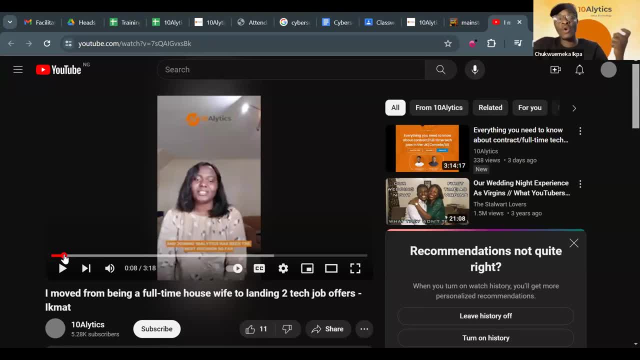 security And also for business analysis. there is what we call process mapping right. So if you learnt process mapping in business analysis, you already have that transferable skill, because in the cyber world you still have to map your processes, the process. 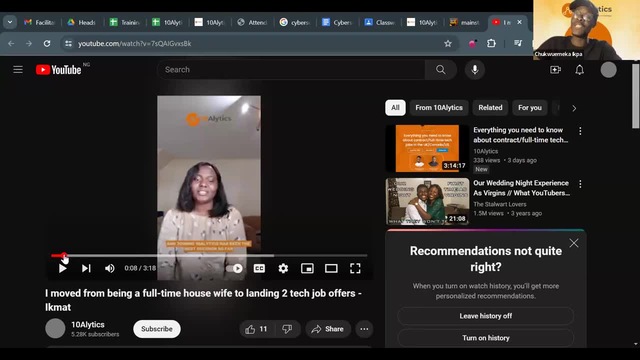 around the threat that is coming or how you want to defend an attack. You're going to still process map all this area. So these are basic transferable skills that you can move from your BA knowledge into cyber security. I don't know if that makes sense to you, Michael. 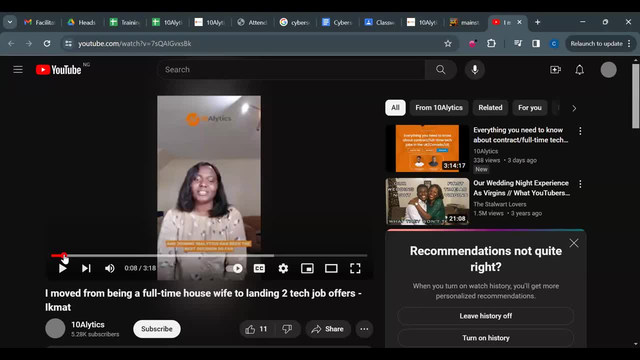 Yeah, it makes sense. Just in addition, is there, any way, the CV? okay, my CV can be built in the way that it captures both a business analyst role and a cyber security role. Is it possible? Of course, Yeah, of course. 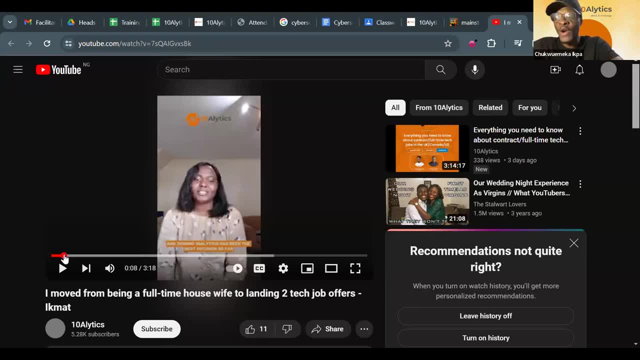 it is possible. It is possible So the way we structure our CVs, because we have people that possibly this person was in the bank and the person may be a customer service person, and now the person is trying to transition to business analysis. 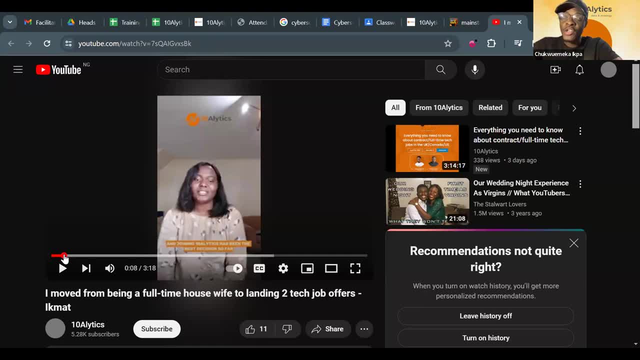 So because in the bank you get to do what we call interacting with customers, that still serves as elicitation. So instead of saying that they worked as a customer service person, you can just coin the word to be a business analyst that was eliciting information from customers. 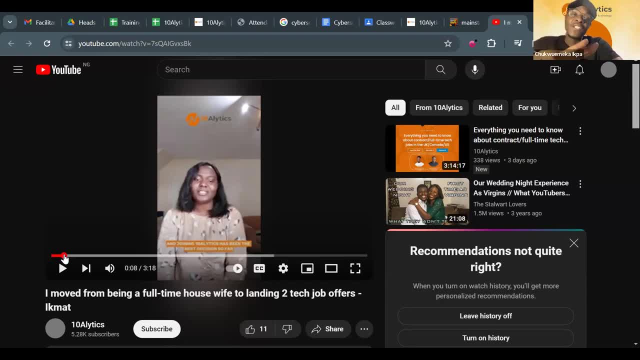 So, even though they're in the bank, we have now transitioned their CV to look like they also were serving as a business analyst while they were in that exact role. So what we do is, basically, we look at your historical background and we can now be able to teach you. 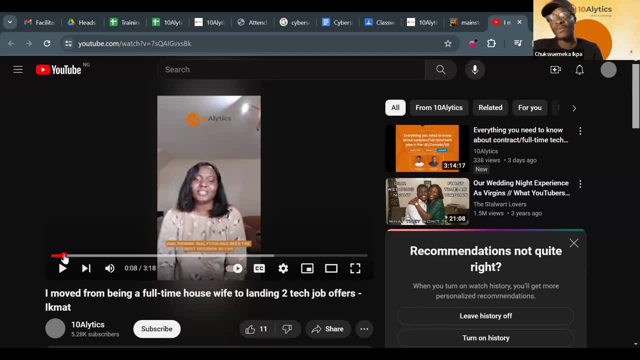 how you can now transition your CV to transfer some skills that you've learned before into the present role that you're trying to transition into. Okay, Thank you very much. Thank you All right. Thank you so much for that, Michael. All right. 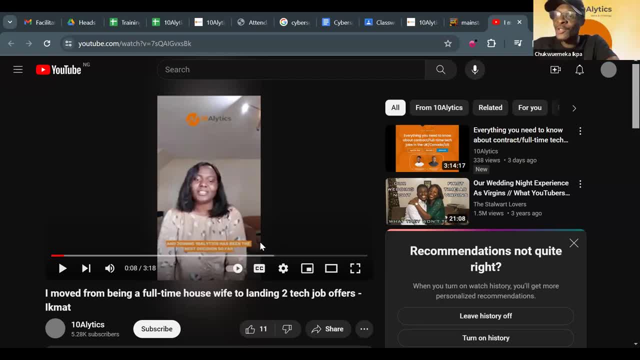 So if you are just here and you have questions, please use the raise hand icon and we are going to ask you to unmute to speak. or you can drop your question in the chat box and we are going to pick it up from there While we're waiting for that. 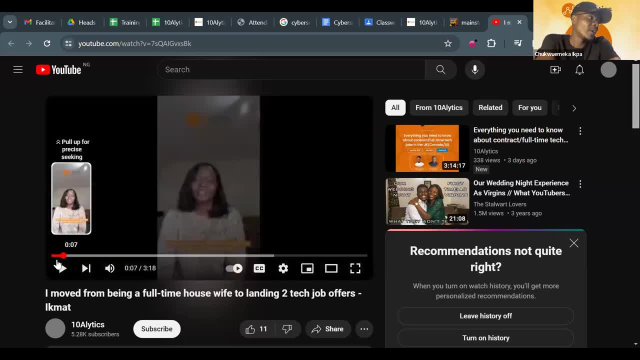 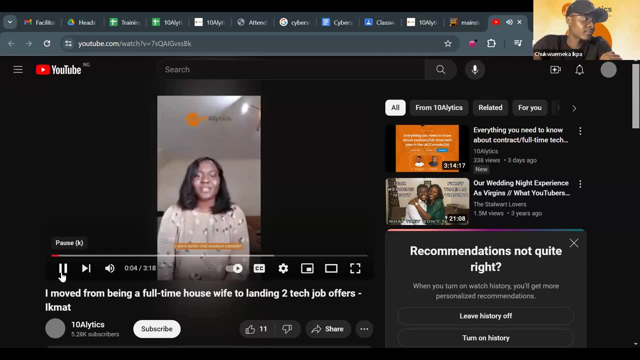 let me play this video from ICMAT so that we get understand some things that we are talking about. I was with a match called internalitics and joining internalitics has been the best decision so far, You know, for me, someone coming from a background of 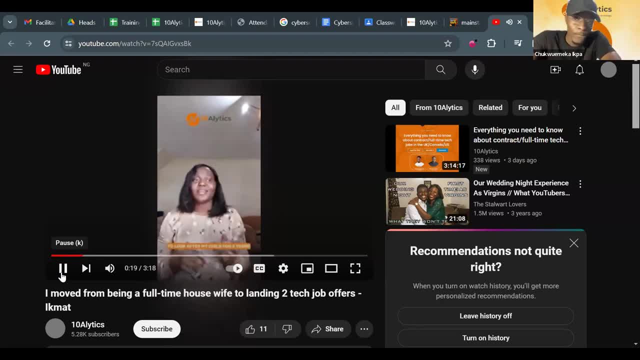 full housewife because I had to stay back home to look after my child for four years, and then wanting to break into something new, wanting to go back into the workforce, you know, wanting to place myself in the society for better job opportunities. so it was a lot. 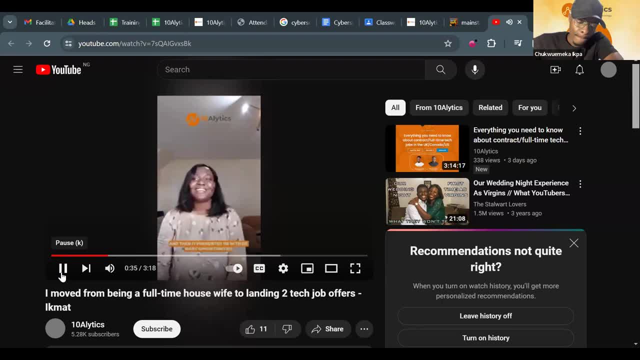 And then I'm glad that internalitics came along. and then it presented me with so many opportunities right in front of me, better opportunities, and then I'm glad I took it. And then also the advice of do not sell yourself short, that FA is always very, very valid. 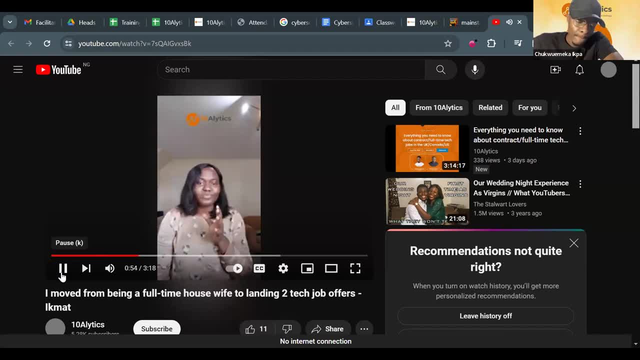 because place yourself right, don't sell yourself short. it's a very, very valid advice. Internalitics, they will hold your hands like a child. you know, through the models, you have the opportunity to go back and study. you have the opportunity to go back and 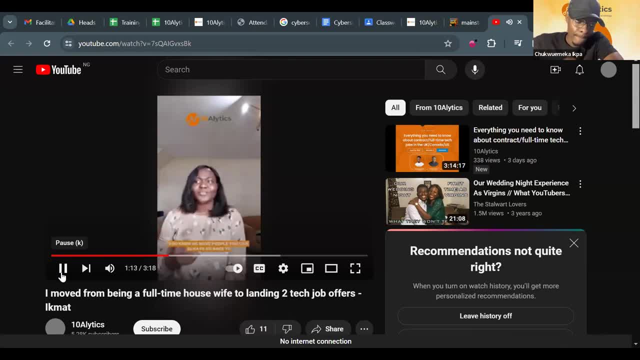 practice. you have the opportunity to ask questions. you know we have people you can always go back to, even outside of class class hours. It's the most amazing experience so far, really. And then another thing is the interview prep guys. that is another very important. 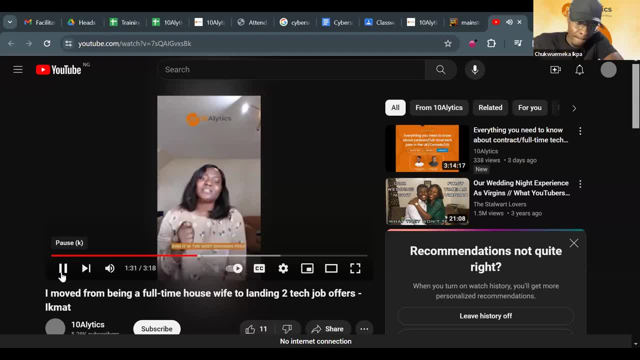 thing. I did my interview prep with Mr Muhammad and it was the best decision ever because he was like, he saw into the future. he knew what was going to be asked and I'm glad that I took. I wrote down all the things he mentioned. 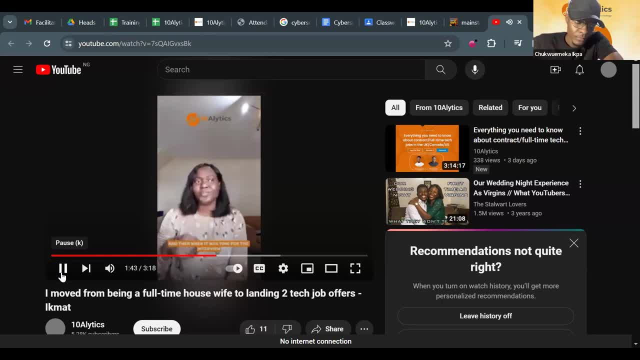 I went back to practice and then, when it was time for the interview, it was like everything he was mentioning, everything he mentioned, it was just kept on. and then when I was answering those questions, I was so confident- you know, because I already practiced- I did an excel. 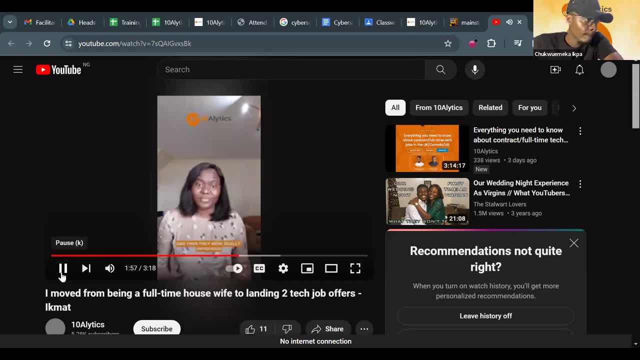 test. I did a maths test and then they were really impressed. and another thing is, guys, he may not come as fast as you expect. definitely you are going to get some no's and then you may begin to think you are not good enough. you are good enough, yes. 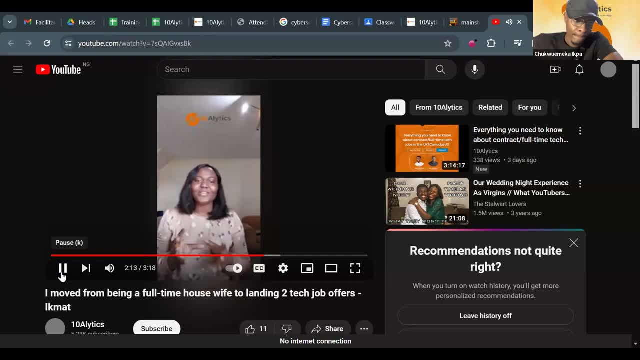 the no's will come, but always take it as a basis for learning and development, because after every interview where I got a no, I always make sure I get a personal feedback. so I work on those feedbacks for my next interviews. and yes, it worked. it really. worked for me because I got my first job 3 months into the program. my first job. I couldn't take up the job because I was a student and I was only eligible to do to work 20 hours. so I couldn't take up the job 3 months later. 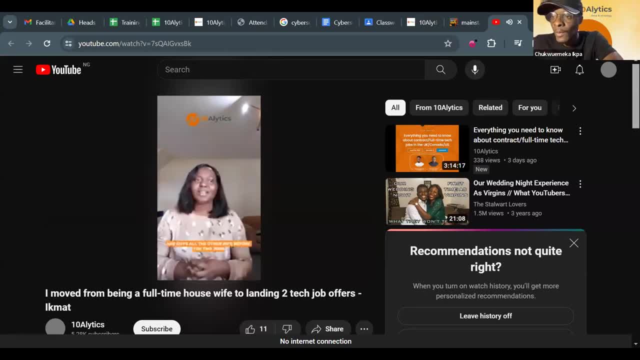 I got 2 jobs with full visa, sponsorship and guys. all the other no's before the 2 jobs. When my parents said yes, I was like: this is it. I am well prepared. I am well prepared for with the yes's I got. so, yes, the no's will come. 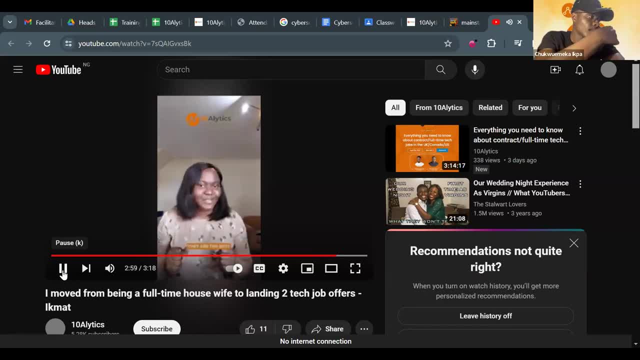 but do not give up, because you always have analytics to go back to. they are the best, best thing that has ever happened to me. and then, yes, and they are the most affordable, the most affordable you will come across so far. Yes, the analytics for the win. 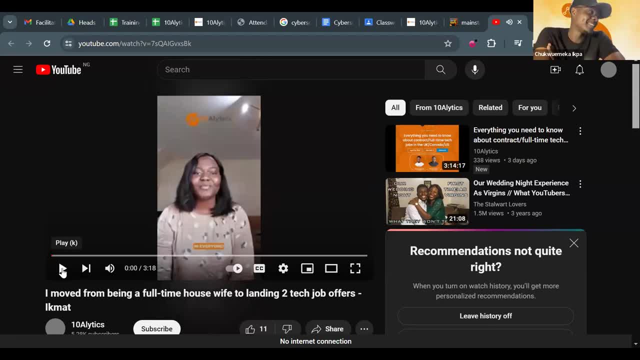 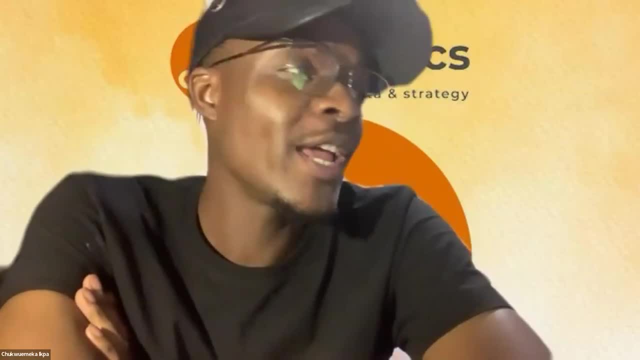 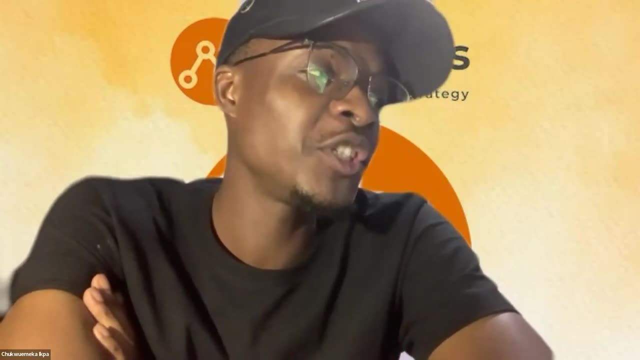 Hi everyone, All right, Amazing, amazing. So, if you heard what Iqbal said, she was able to transition from a full housewife to becoming a full-fledged tech sis And her own transition was amazing because she got some roles while she was still in class. 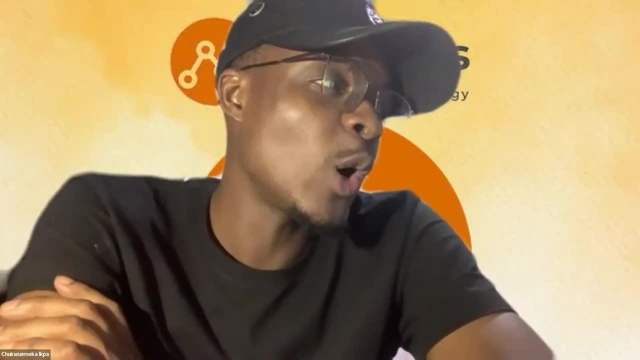 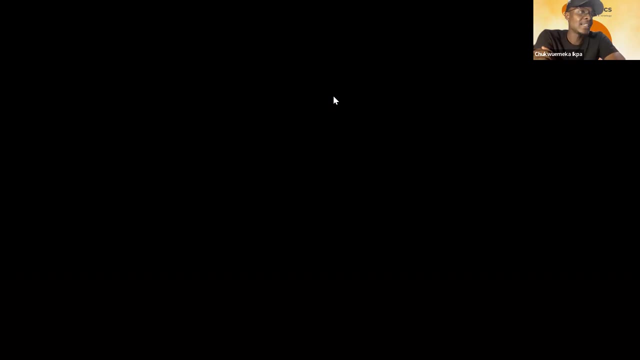 while she was still studying in school, And she was not able to take it all because of limitations in working hours. And one month after she was done again, she got two roles And at this point she now had the liberty to select the one that she wants to go for. 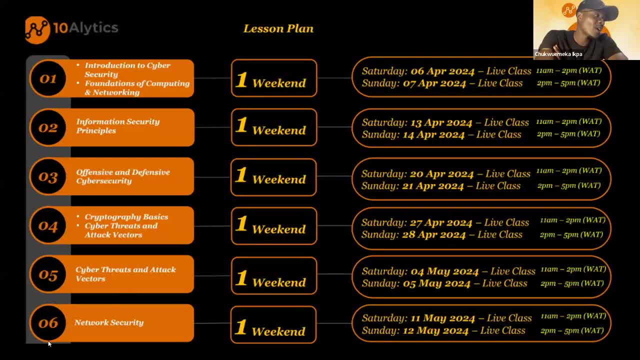 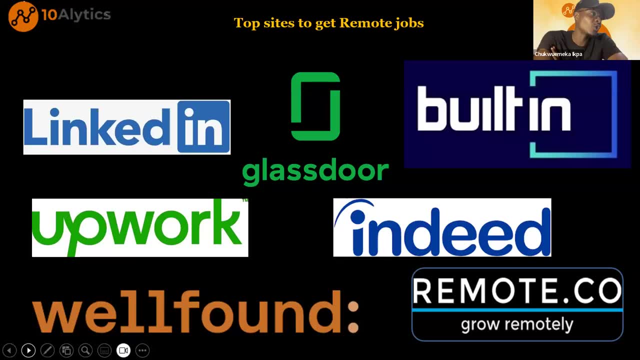 So this is still the question time. So if you have any questions for me, you can use the raise hand icon and ask questions, or you can drop it in the chat box. Remember, our next cohort is starting at the end of the semester. 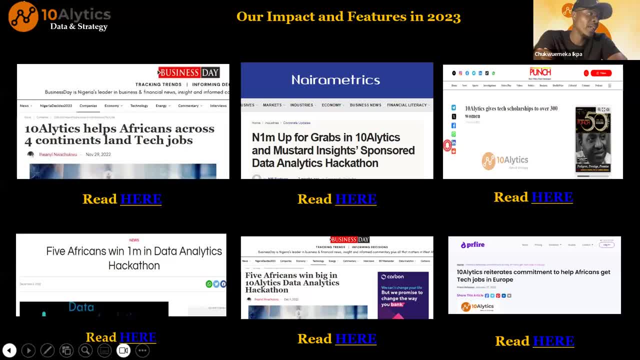 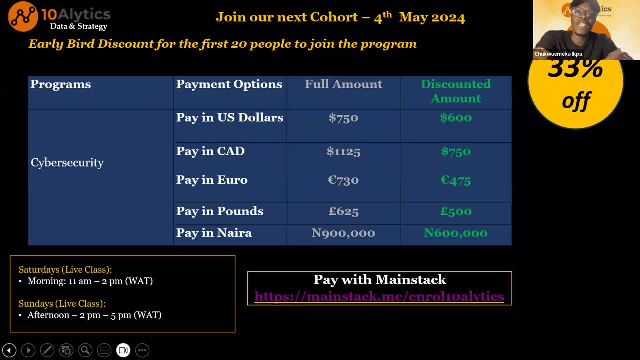 Fourth of May. That is Fourth of May And the payment is $600, $750 Canadian dollars, 475 euro, 500 pounds or 600,000 naira, all discounted for you to get into this exact Starbucks security field. And the classes runs on Saturdays. 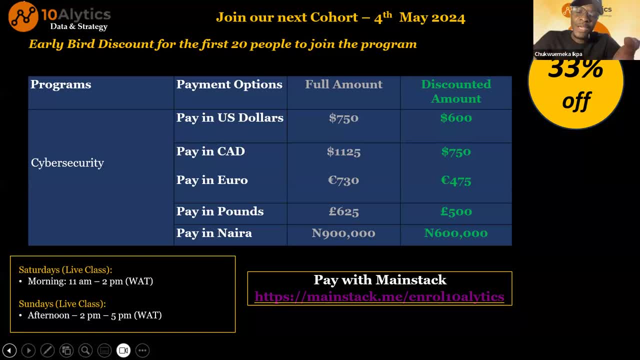 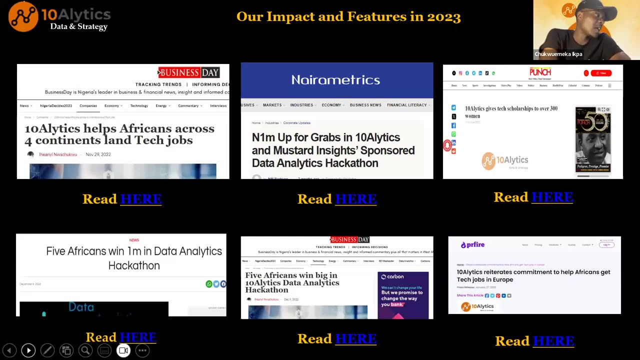 from 11 am to 2 pm West African time, And on Sunday, from 2 pm to 5 pm West African time. So what are you still waiting for? Here's a couple of ads that we've been on. 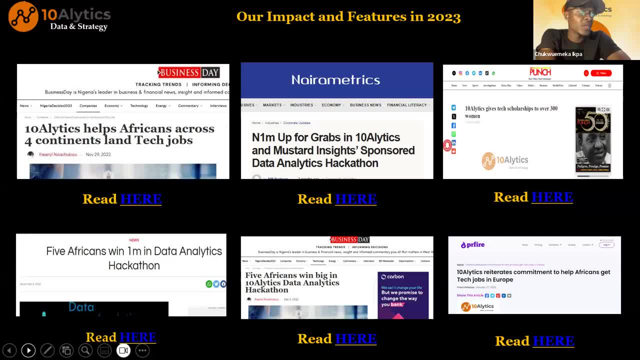 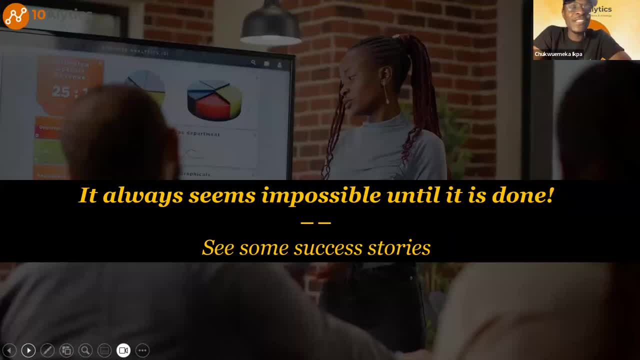 Analytics helps Africans across four continents to have tech jobs. So when you get this slide, you can always watch all this. Okay, So these things always look impossible, but it is done Right. When we speak about these things, it always sounds impossible. 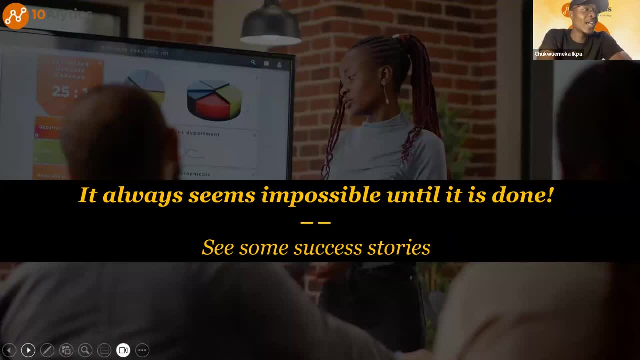 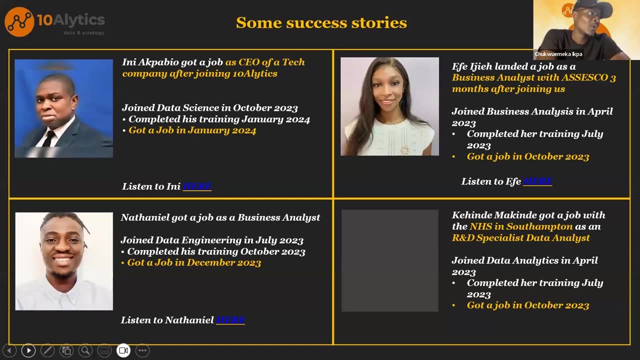 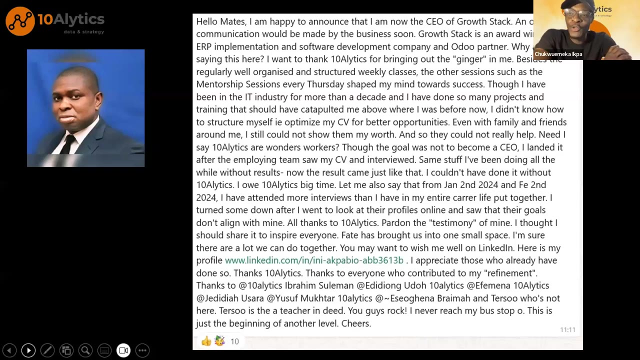 until you experience it personally. That's when you get to know that these things are possible. Now there is this amazing story that we have about Eni Apabyo, right? So this is a long message that Eni sent to us after he got his own- you know- job. 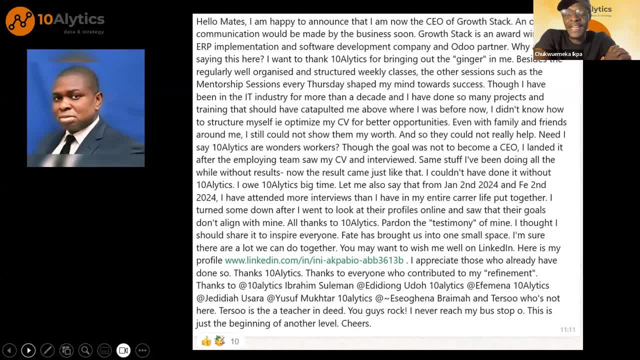 Now the funny thing about Eni's story is that Eni went for an interview for a manager role. On getting to that exact place, Eni was offered a CEO role after they saw what he has to offer, And it's not that he'd not be applying to places before now. 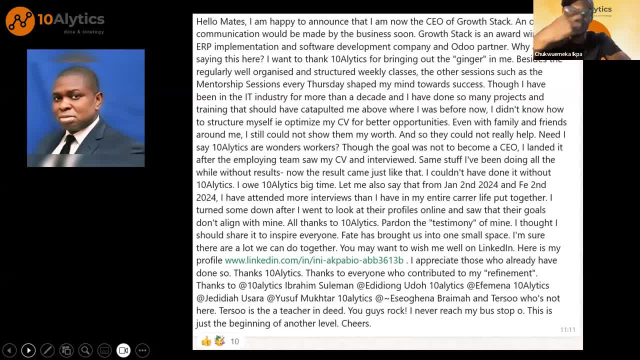 What he even said is that we unlocked him to give him the necessary skills for him to start pushing. Imagine going for a managerial interview and you are offered a CEO role. Now, if you talk or say these things out there, people will definitely ask. 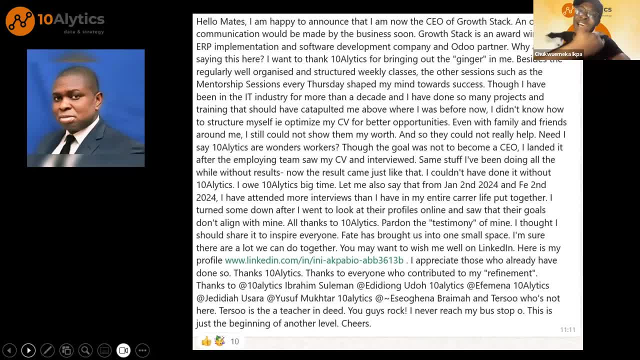 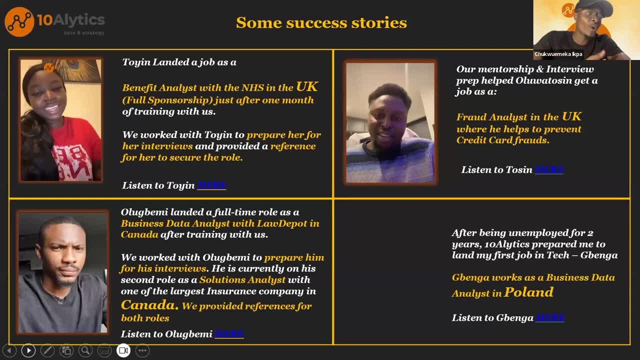 is it possible, But these are things that we have experienced. These are things that people have come back to tell us, And you don't really have to worry whether you have a technical background- right, Because even Joshua on Discord did not study cybersecurity. 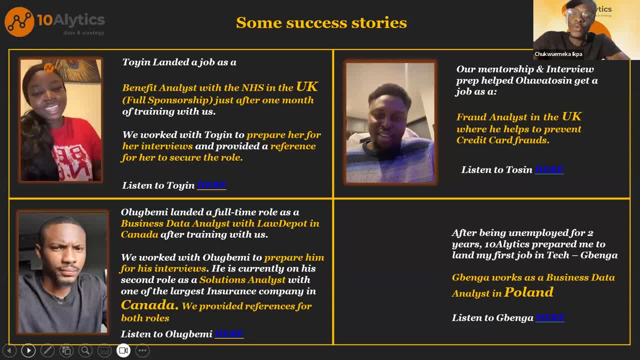 but today he's a cybersecurity expert with one of the top most banks in Africa, And we have a couple of success stories from people that have also experienced this, So I want you to you know. fill in the attendance form so that, once this call is over, 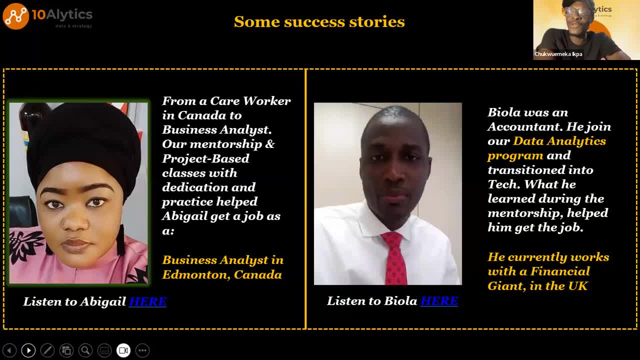 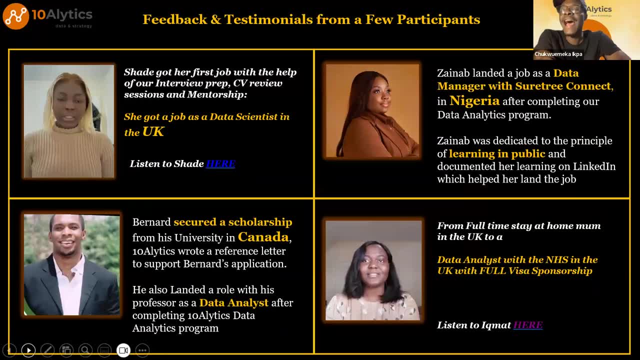 my colleagues are going to send this slide to you and also the recording of this session. So if you have any question, please feel free to use the raise hand icon and we are going to call you, Or you can drop your question in the chat box. 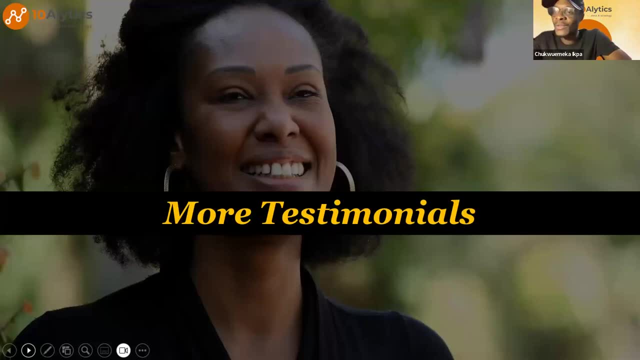 and we are going to pick it up from there. Okay, we still have a couple of people on the call. We've had Michael, we've had Elvis, We have Sam. We're on the call. We have Cheezy, We have Chukwu Emeka. 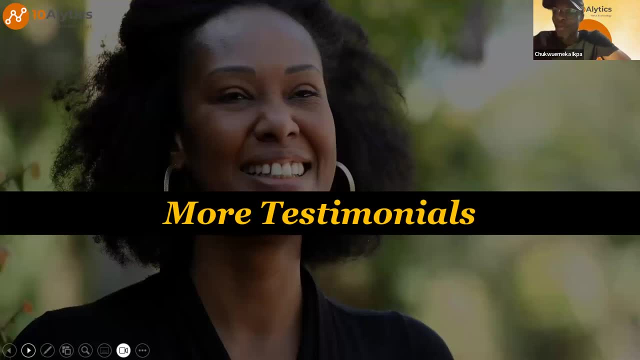 Hi Nemsik, We have Emmanuel. Hi Friday We have Godwin, Goodness, Harry, iPhone, Girade, Francis, Oyabimpe, Semitope, Steven Taiwo and Zoom user. If you have any question, please use the raise hand icon. 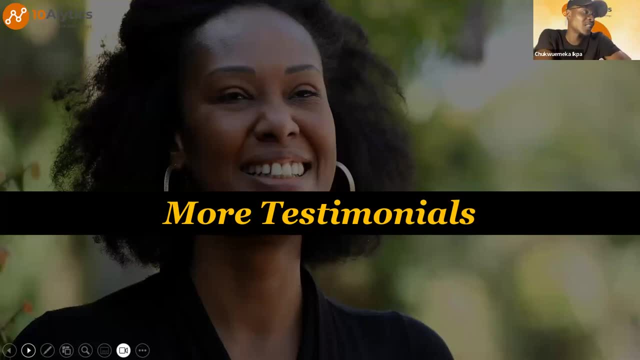 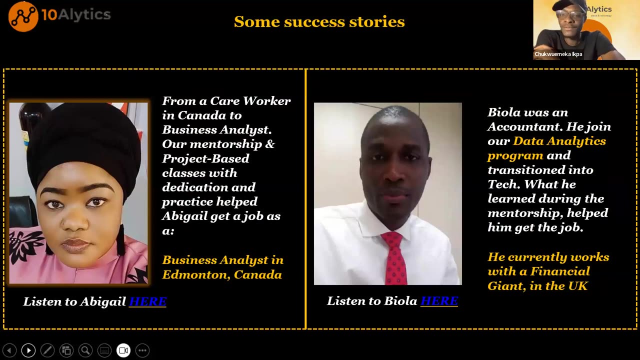 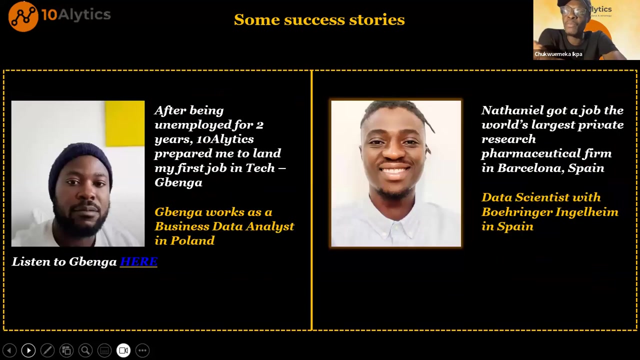 and we are going to call you. Or you can drop your question in the chat box and we are going to pick it up from there. Any question from anyone. Remember: the discount is not for everyone, It's just meant for the first 20 people. 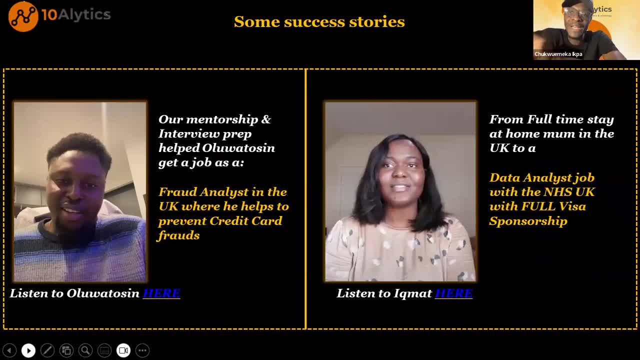 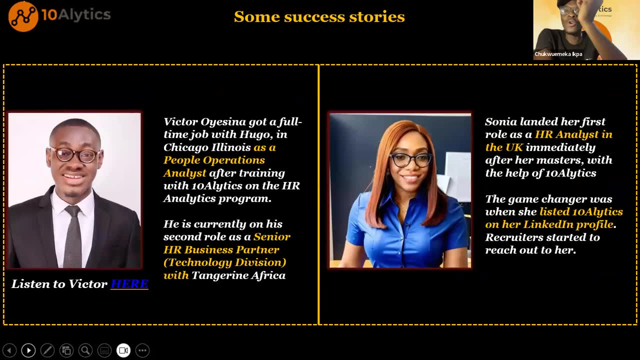 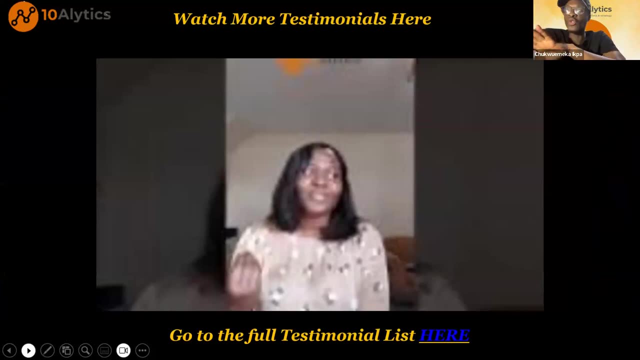 to join this exact program. So please try and take advantage of it so that not when you call you are going to get the talk like, oh, the 20 slots is fueled. Try to take advantage of it now that it's here so that you can get into the tech ecosystem. 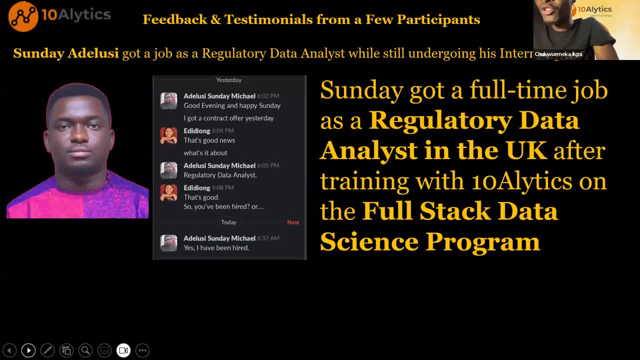 Okay, I don't know if there are any questions. Hi Joshua, are you still there? Hi Joshua, are you there? Hi Joshua, Okay, so I don't know if Joshua is still on the call. I wanted Joshua to give. 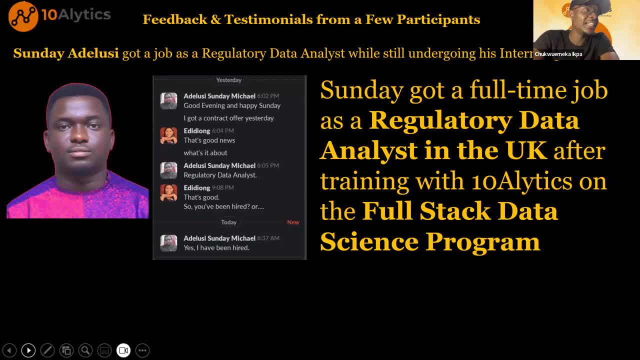 his closing remarks. before we call it a day. All right, so I'm going to leave you with this. What are you still waiting for? Remember: the time that you are, the best time to get into tech is yesterday, and the next best time is today. You can't keep pushing it forward. Last year, we offered discounts- 50% discounts- for International Women's Day and the price should be around 150,000 Naira. This year we offered that same discount- 50% discount- and the pricing was 250,000 Naira. 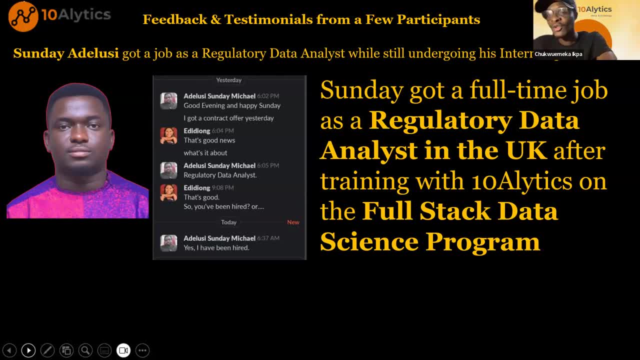 Now we are offering a 33% discount and it is 600,000 Naira. Tomorrow the discount may be there, but the financial amount may still have gone up, So I always advise people to take advantage of the pricing. That means at every point in time. you also have opportunity to defer, So that means 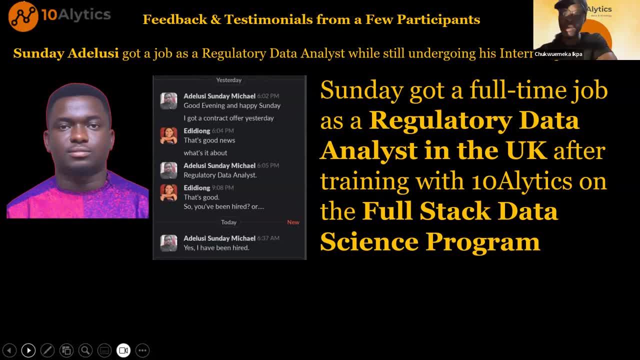 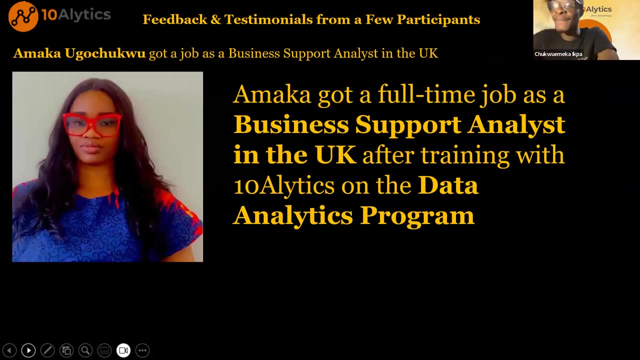 that you want to start the classes in June instead of starting in May. right, So you're making payments, You've locked down the exact pricing that is currently on, but you want to start your classes in May. In June, I mean, that option is also available. Okay, So, in absence of any other, 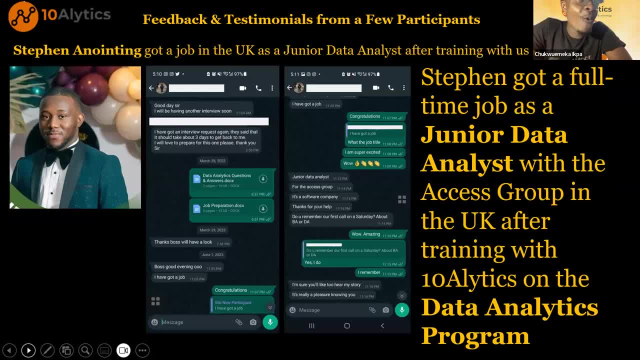 thing. we are going to call it a day, So I can't wait to see you guys in class. Elvis, Michael, I can't wait to have you guys in class. Thank you guys so much for joining us today. I'll see you. 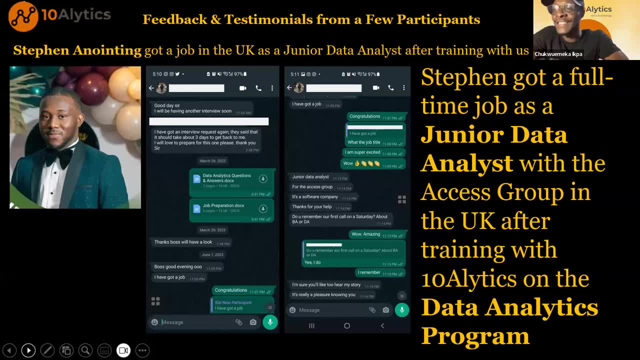 and this is where we round up for today. Thank you once more and cheers. See you next time. Bye for now, guys, Bye.